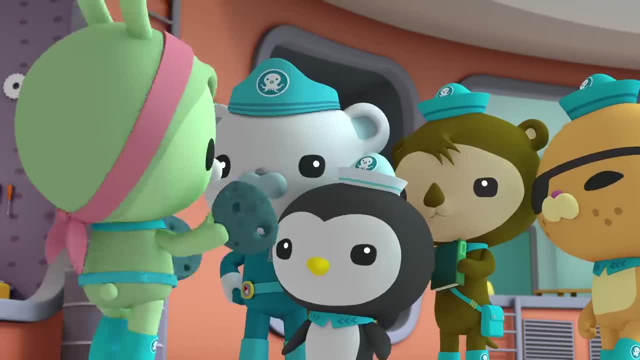 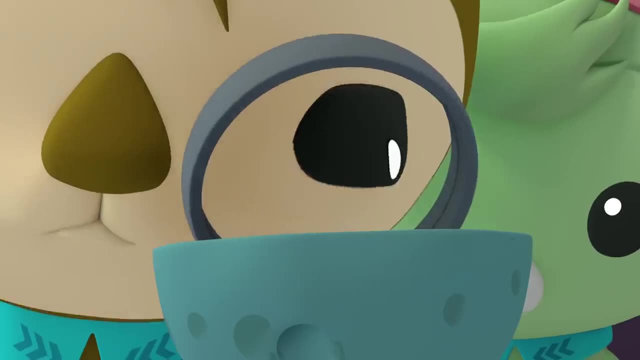 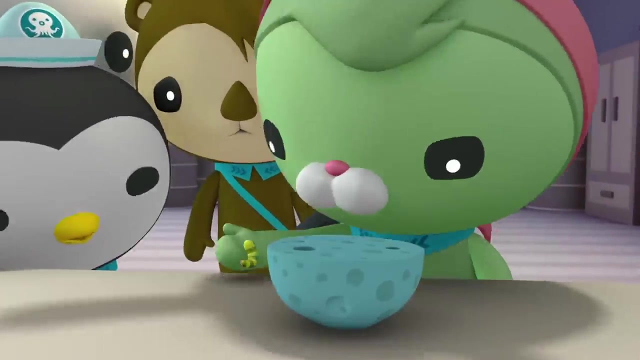 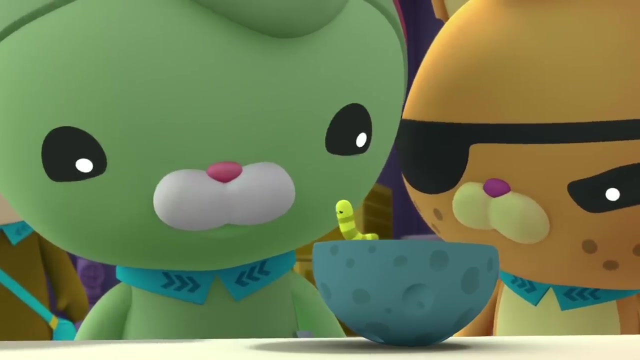 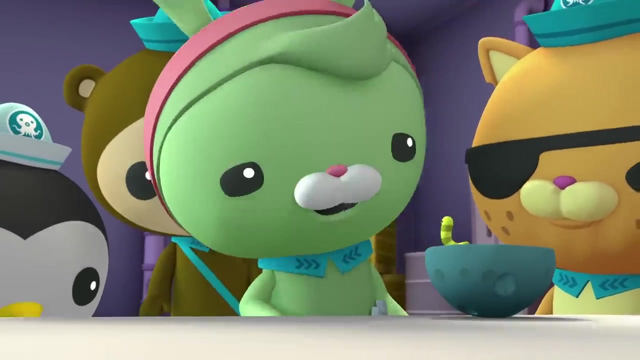 I think there's something alive in here. I'll go check. Ah Wait, Where am I? You're on the octopod, My house It's broken. No worries, little guy, We can put your house back together faster than you can say. 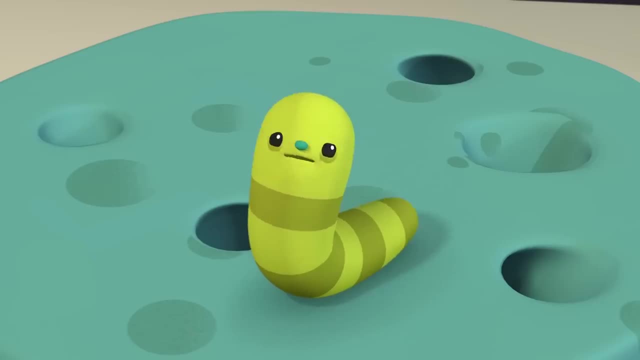 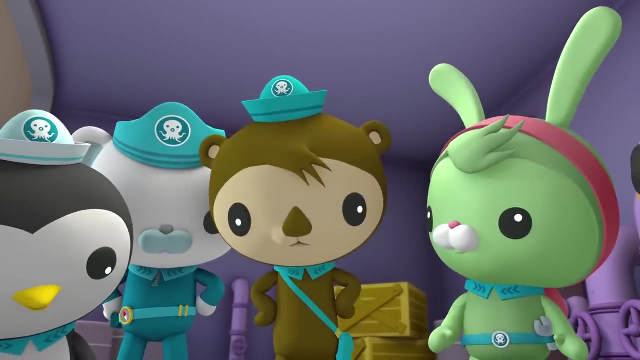 Bunch of munchie-crunchie carrots, Okay, But hurry freezing, and this light hurts my eyes. You live in the Midnight Zone, where it's always dark and the hydrothermal vents are very hot. The Octopod must seem very strange to you. 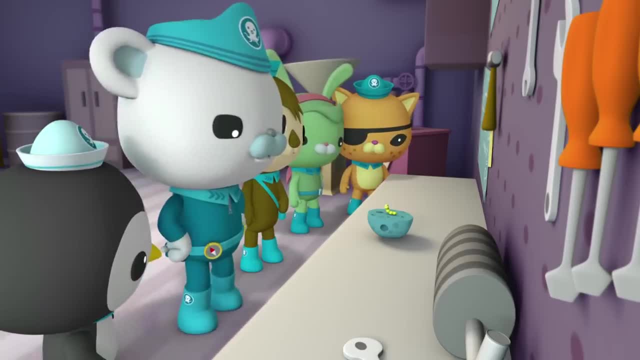 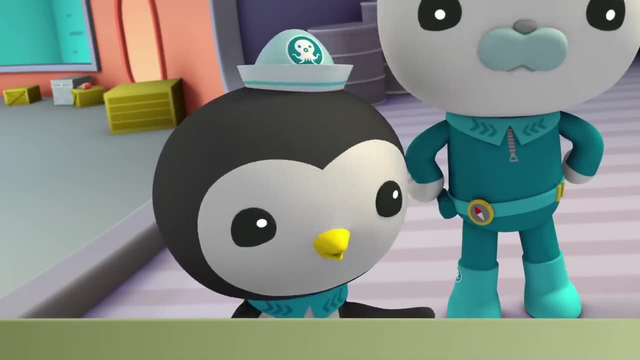 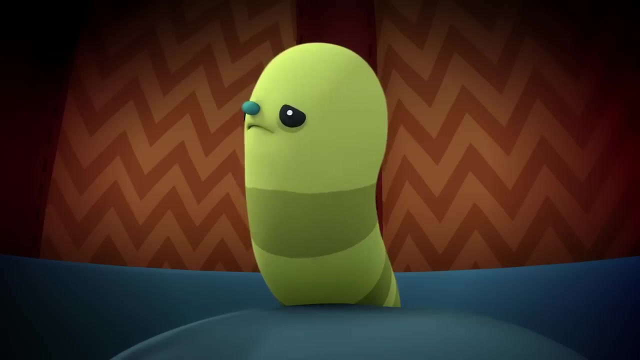 I want to go home. Tweek will fix your house and then we'll take you home to the Midnight Zone as fast as we can. In the meantime, we'll do our best to make you more comfortable. How's that Warm enough? 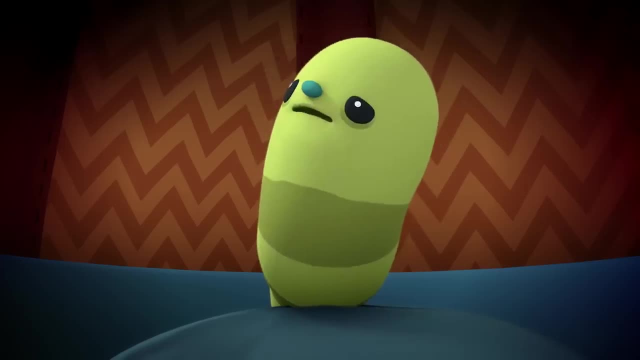 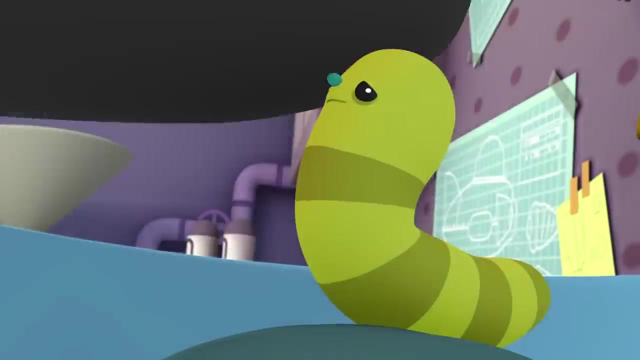 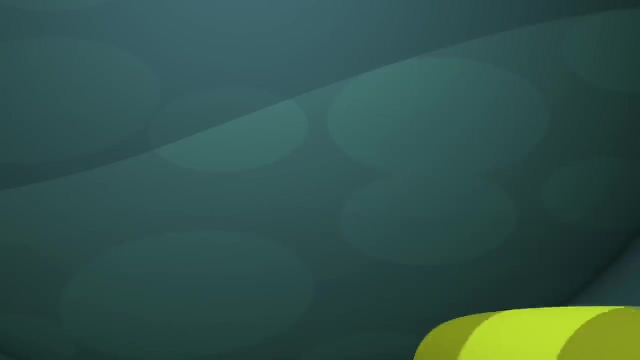 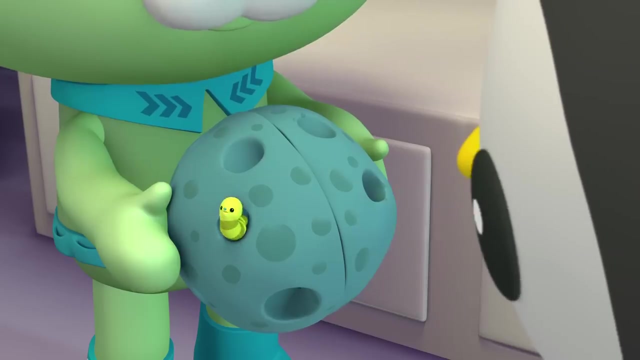 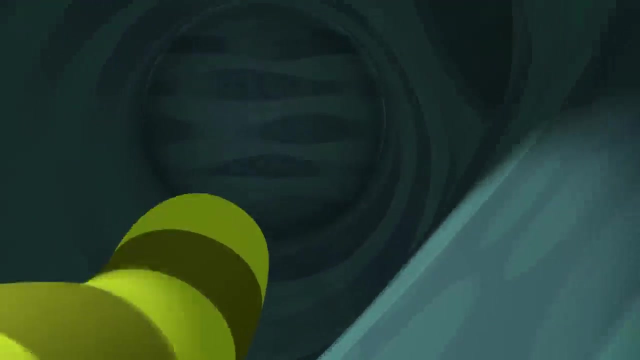 Dark enough. Better For now. Thanks. First we have to work out how the tunnels connect to each other. Give this a try. Wrong, Ok, Let me try again. Wrong, Hold on, That ought to do it. Wrong, wrong, wrong. 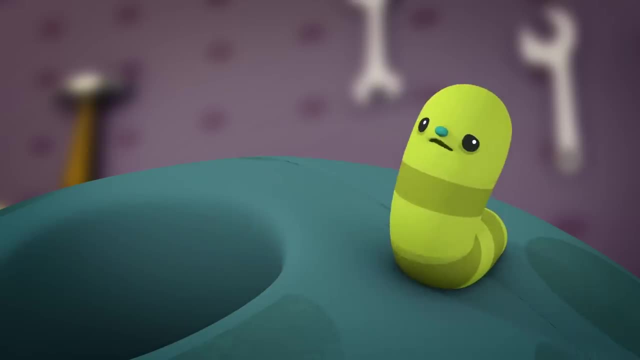 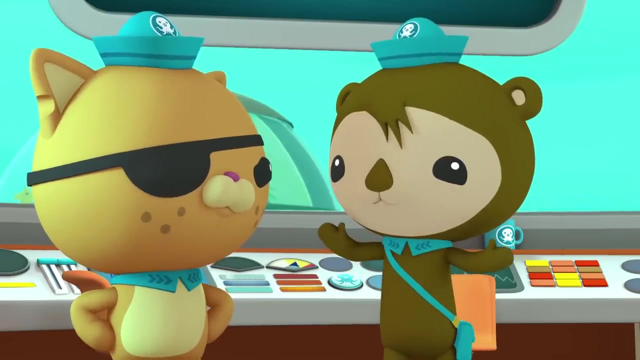 The holes don't line up. I keep bumping my head: Humm-humm-nooker-nooker up water. What Humm-nooker-nooker-poo-poo-poo-poo. What the hell do we do? 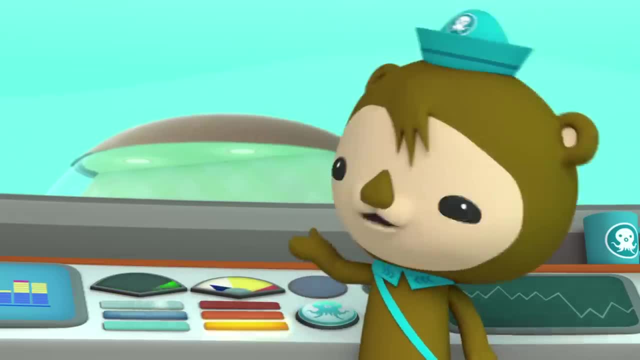 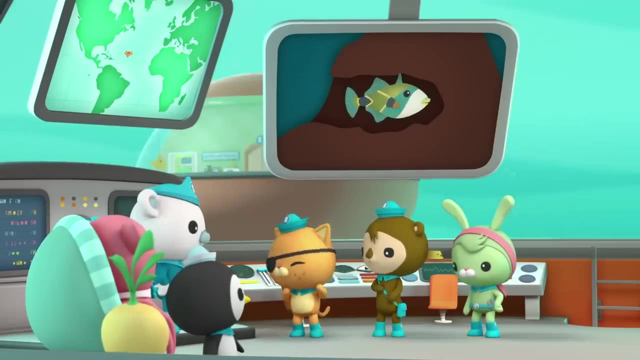 Humm-humm-nooker-nooker-poo-poo-poo-poo. When something scares them, they quickly hide in small spaces, then stay in there till it's safe to come out again. Who would want to scare these cute little fishies? 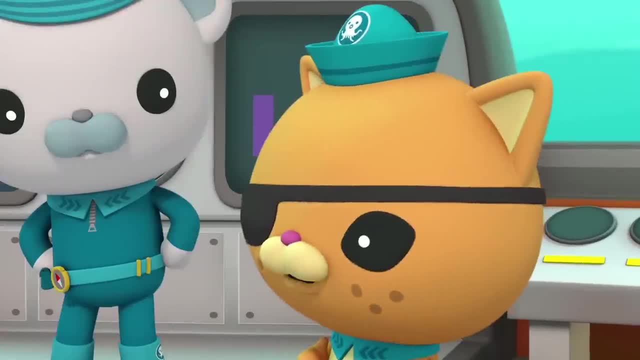 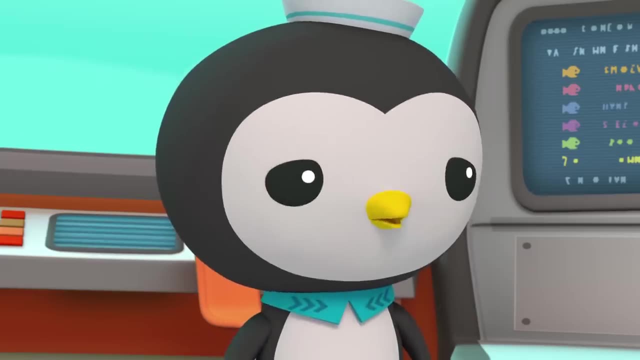 Um, actually it was you, Quasi Me. Yes, The Humuhumus thought that the gut bee was a shark. That's why they swam into the octopod. Oh Sorry, little fishies, Octonauts, let's split up. 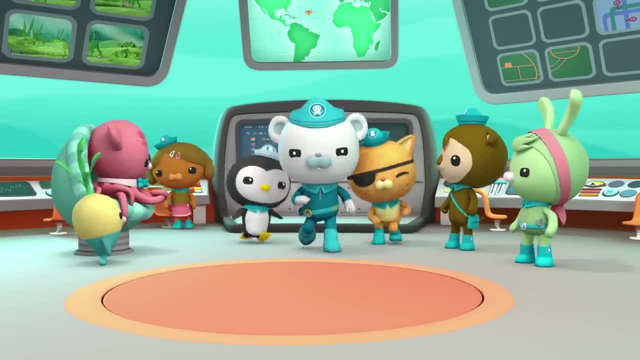 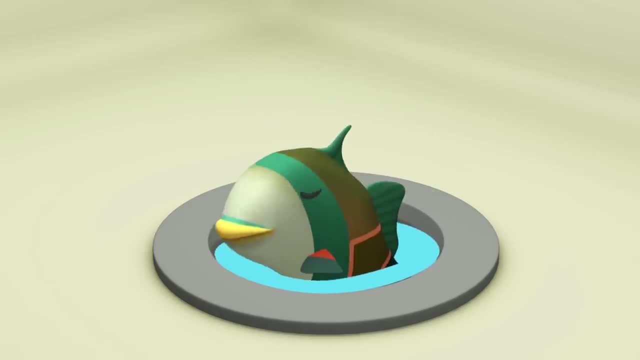 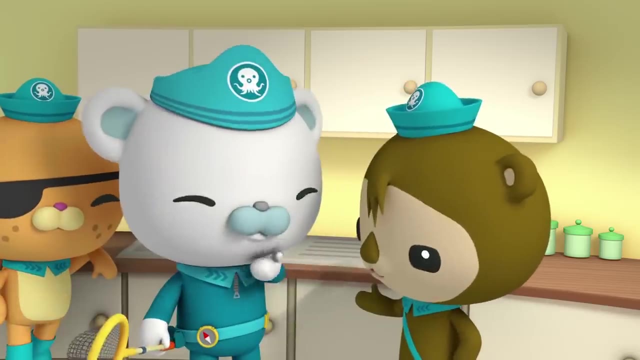 We've got to get the Humuhumus out now. Ahoy there, Humuhumus. There's nothing to be afraid of, Nothing to Fear. Oh, that's right, Humuhumus can blow strong jets of water from their mouths. 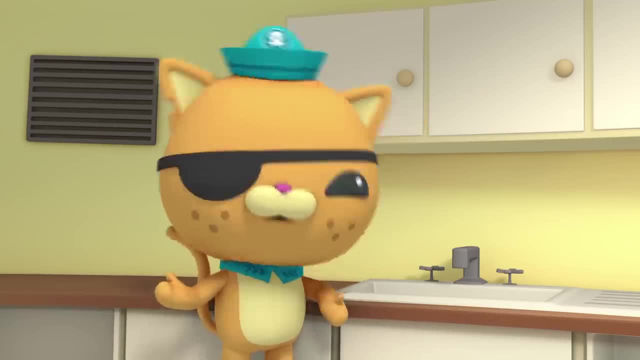 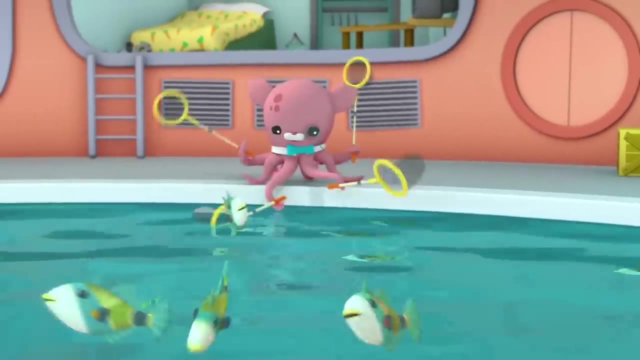 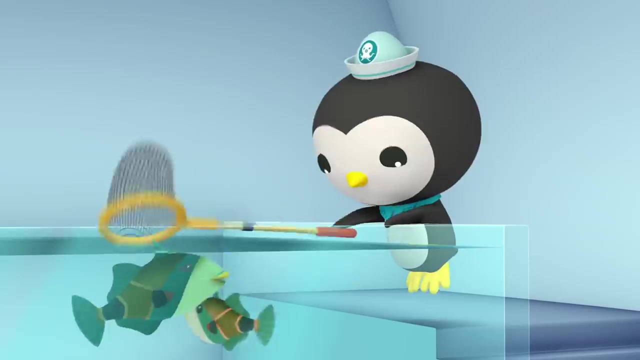 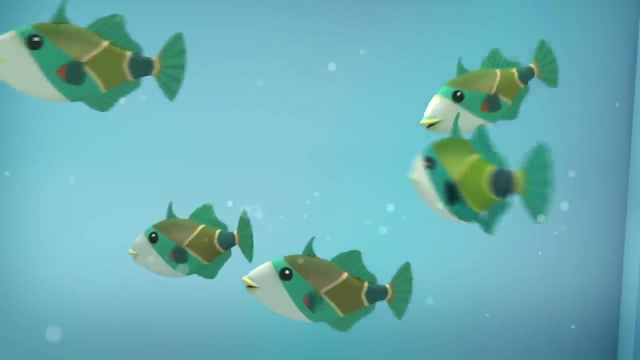 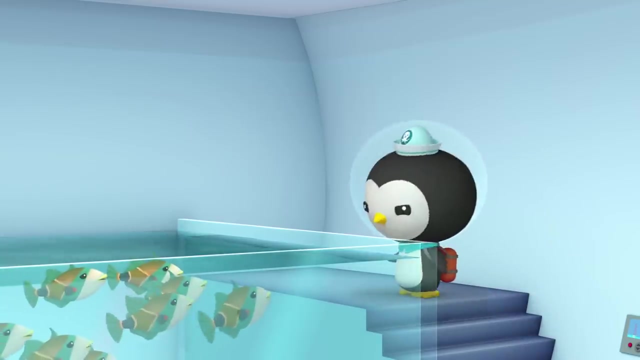 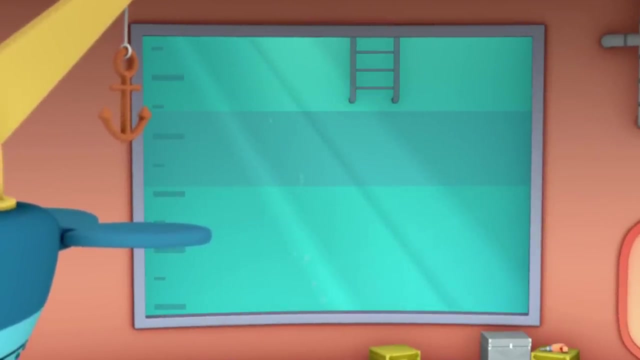 Hmm, now you tell me That's funny: Water in the face. Come here, little fish. Huh, Hank, Is that you? Wait, Hank, it's me Peso. Hank, that wasn't a shark, you saw in the water. 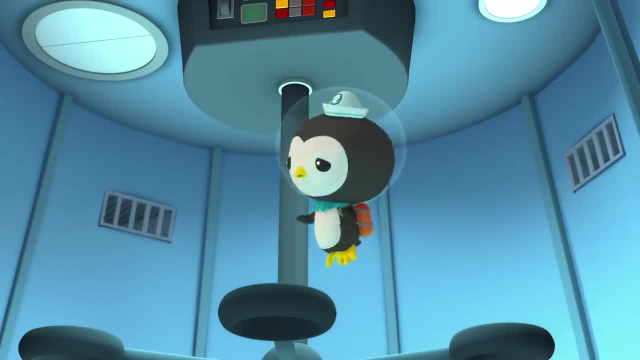 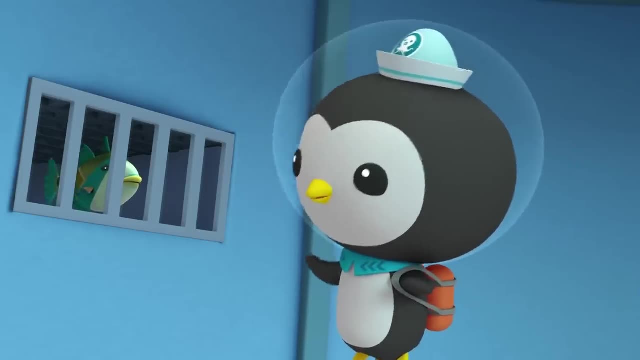 It was just the gut bee, One of our ships that looks like a shark. Ha ha, ha, ha, ha ha. Are you sure? I promise It really is safe to come out. Well, okay, Just a second. 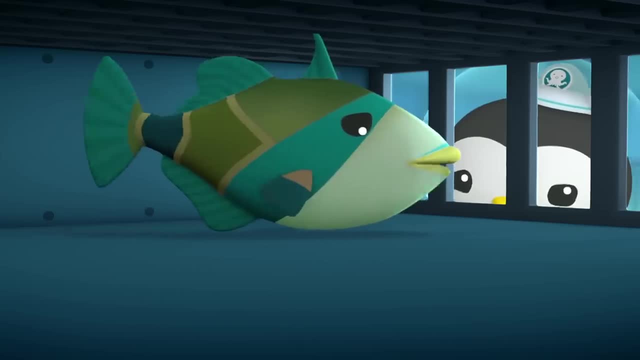 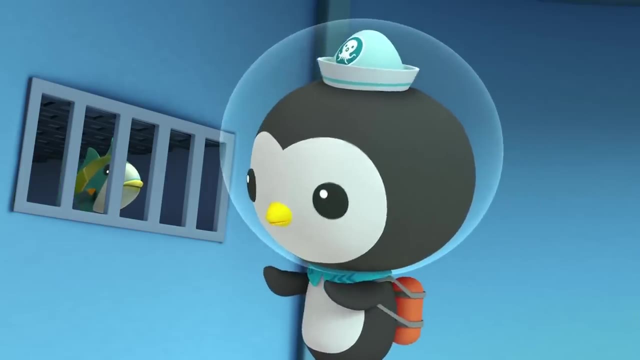 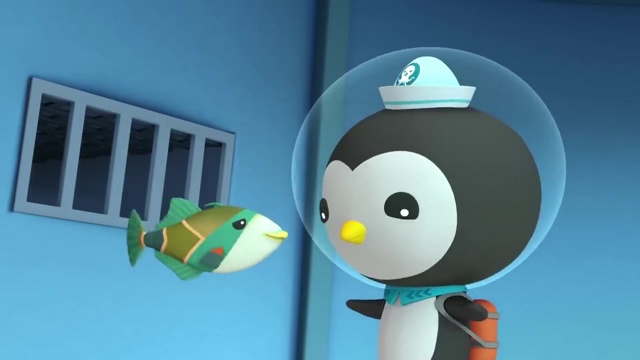 My fin is, oh, a bit stuck in here. Oh, When I get scared, a fin goes up on my back and locks me into my hiding place. Just relax, Just relax, Let your fin go down, All right. Thanks, Peso. 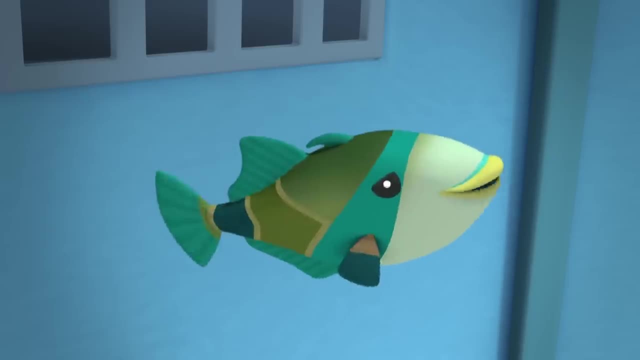 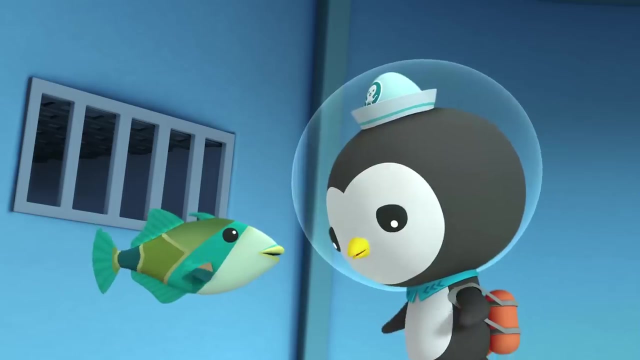 And sorry about squirting you back there. That's okay, But we have to get the rest of your friends to come out of their hiding places before one of them gets hurt. Can you help us? Absolutely. I'll just tell them all that it's safe. 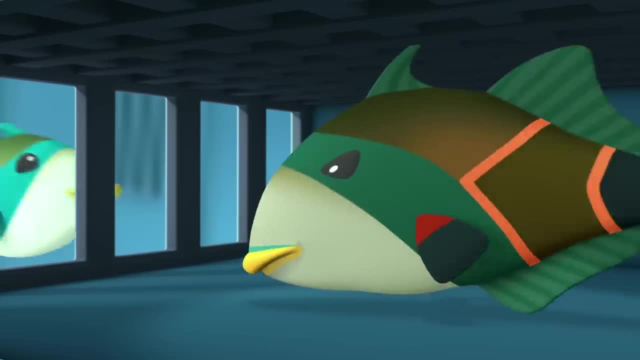 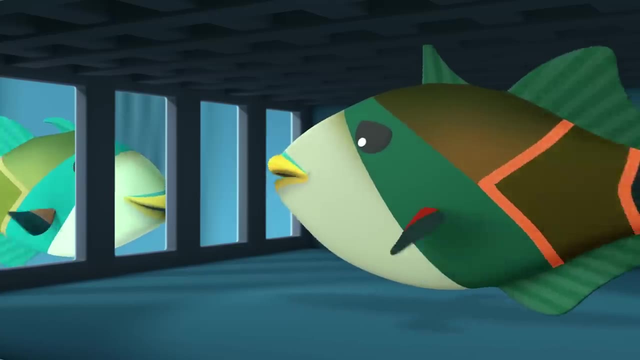 Great. Thank you, Hank. Hello in there, It's me, Hank. There's no shark. You can come out now. I want to come out, but I can't. My fin is stuck. I'm stuck too, Me too. 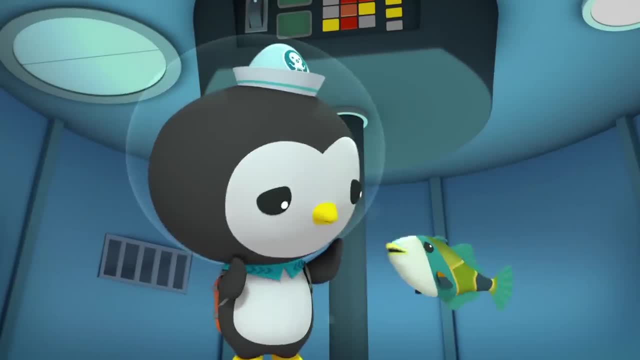 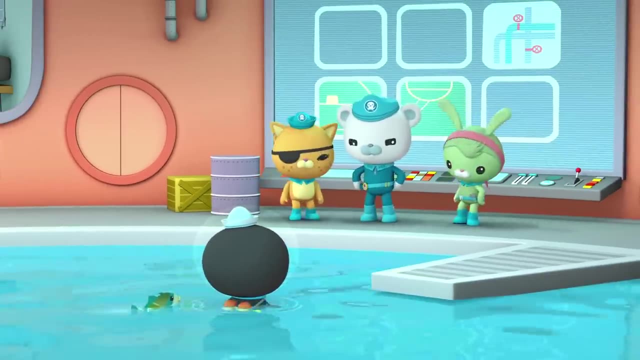 Get me out. I can't move, I can't move. Uh-oh, Come on, Hank, Captain. What is it Peso? We've got a problem. The Humuhumus can't seem to leave the octopod. 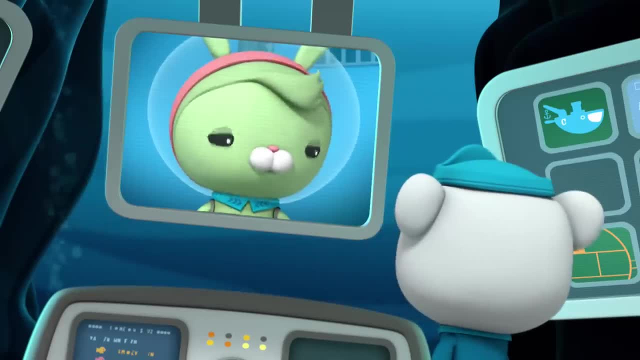 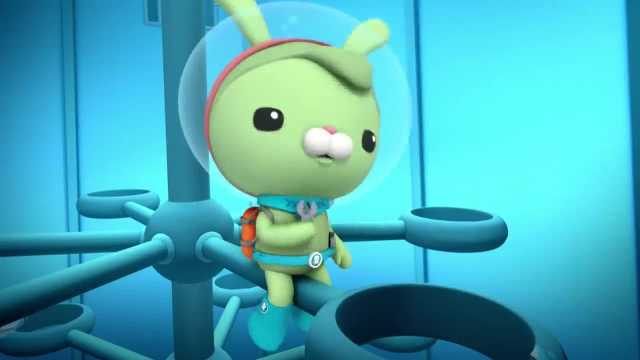 They're stuck in the pipes. I think I found the problem, Cap. Looks like something took a chunk right out of the engine. But don't worry, I'll have it fixed up faster than you can say. buncha munchy crunch Huh. 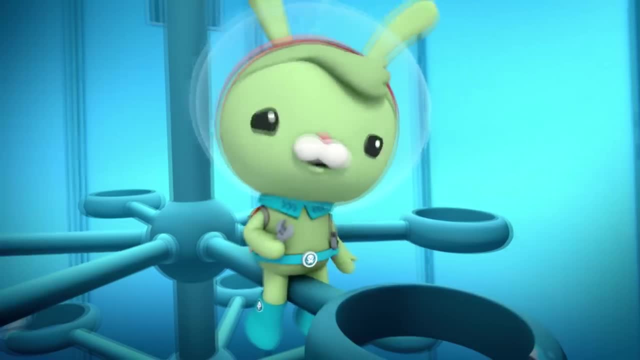 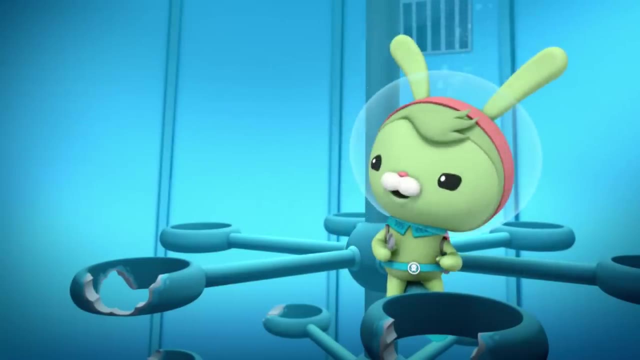 Huh, Huh Tweet. What was that noise, I don't know. But now there's another missing chunk. Humph, Humph, Humph, Humph, Humph, Humph, Humph. Actually Cap, this could take me a while. 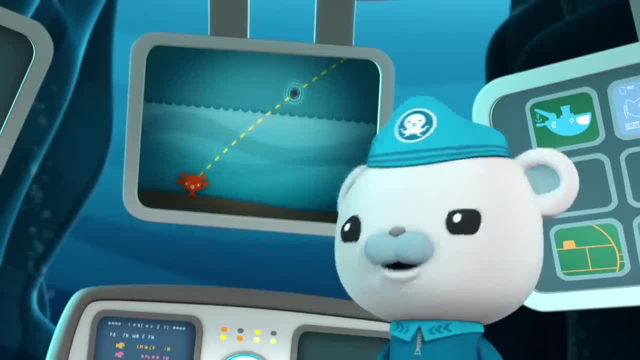 If we can't fix the engine and move the octopod in time, then we need to find a way to stop the meteor. Shellington Inkling. what else do we need to do? Shellington Inkling- what else do we need to do? 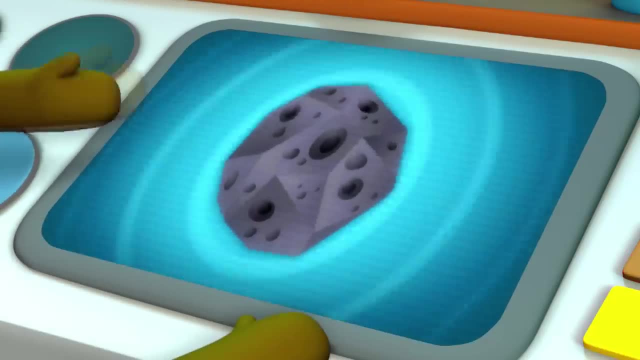 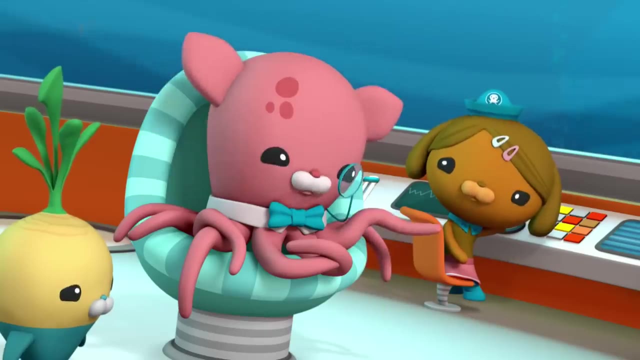 Shellington Inkling. what else do we need to do? What else do we know about meteors? Well, as you can see, they look like big black rocks, Yes, but they're actually part metal 처, That's right. 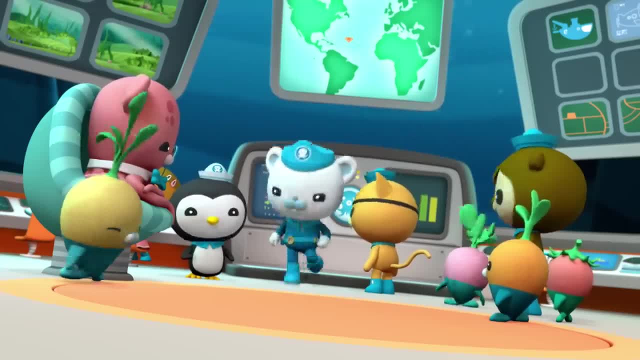 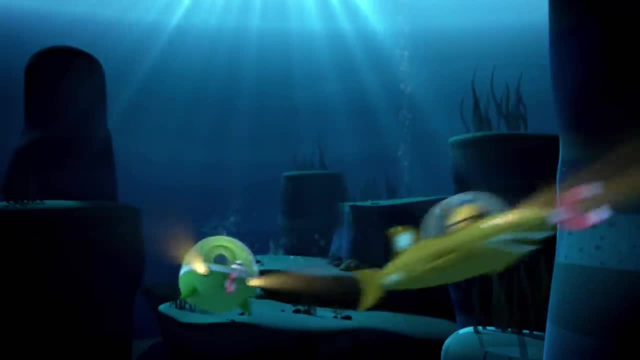 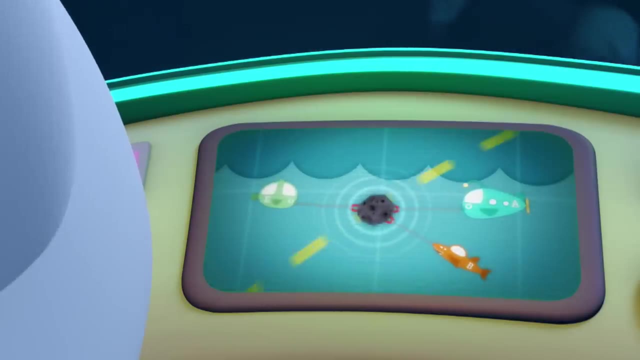 That gives me an idea: Quasi peso to the guns- Octonauts. these magnets should stick to the meteor and slow it down, but it's moving fast. We have to shoot our magnets and hit the meteor at the exact same time. 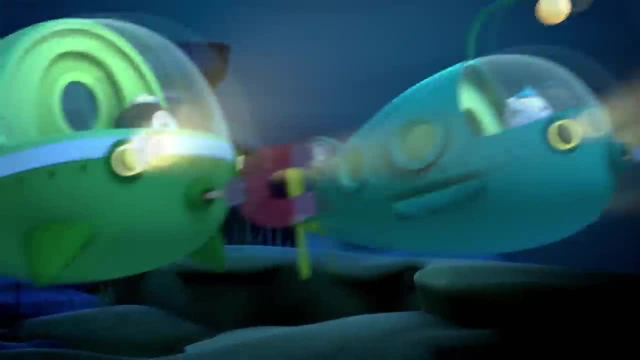 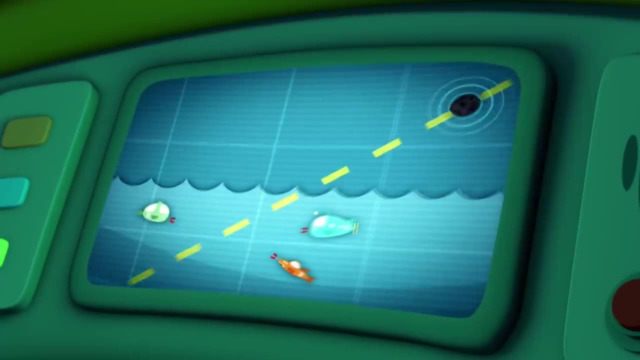 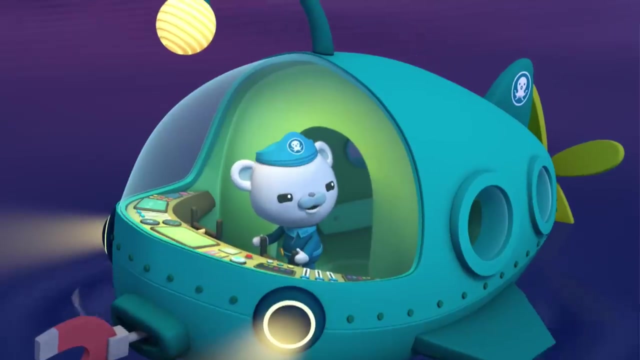 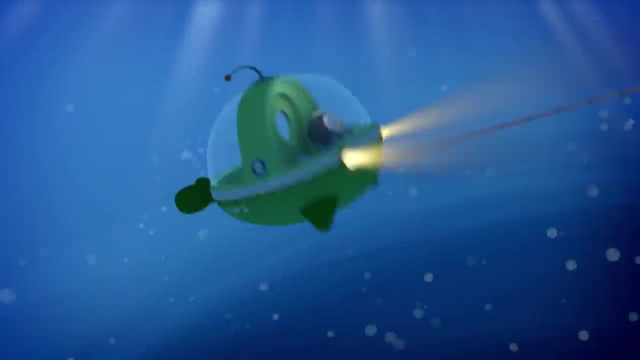 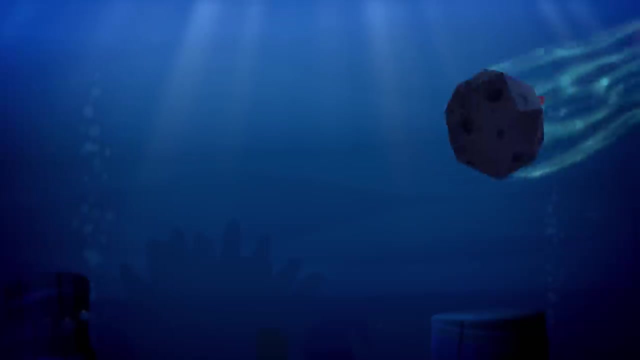 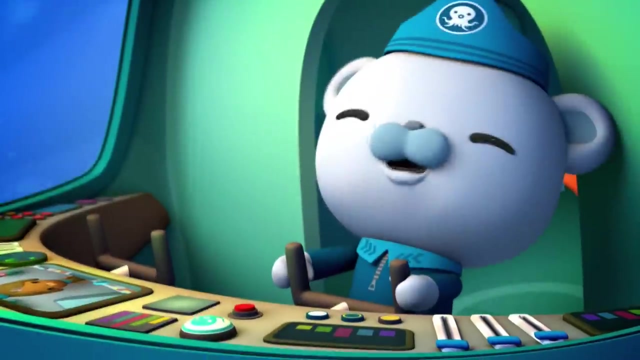 Quasi Peso. take your positions. It's coming in fast, mateys, Get ready. Steady, steady. Now, Dashie. I'm attached to the meteor, but I can't stop it. Prepare to evacuate the Octopod. 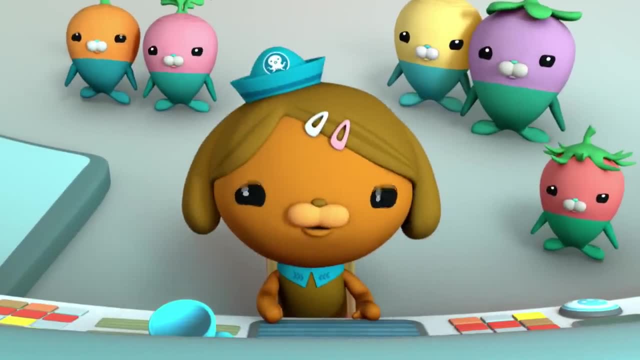 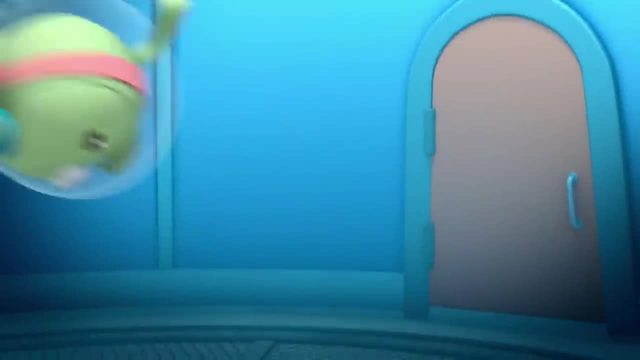 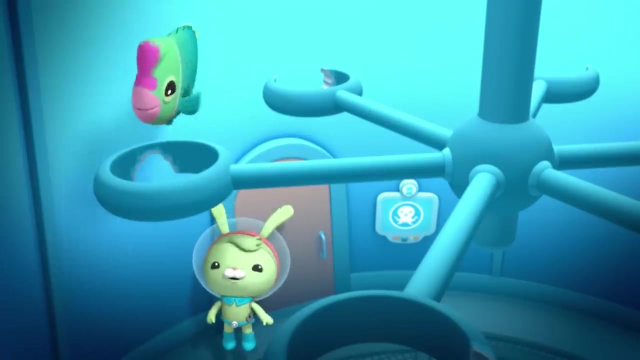 Attention: Octonauts report to the launch bay. We need to leave the Octopod immediately. Huh, Where's all this sand coming from? So you're what's been taking chunks out of our engine, What? I'm sorry, There are just so many interesting things to munch around here. 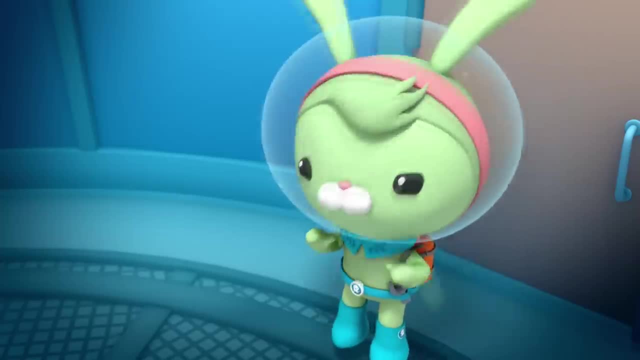 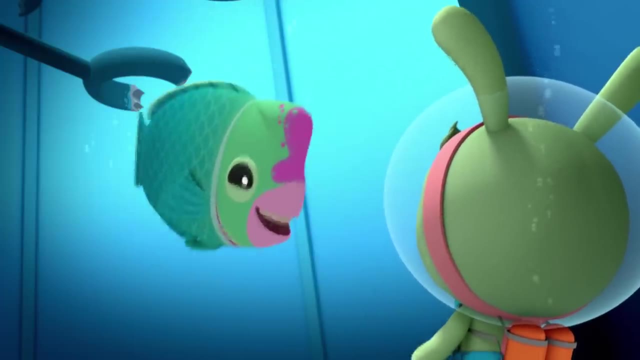 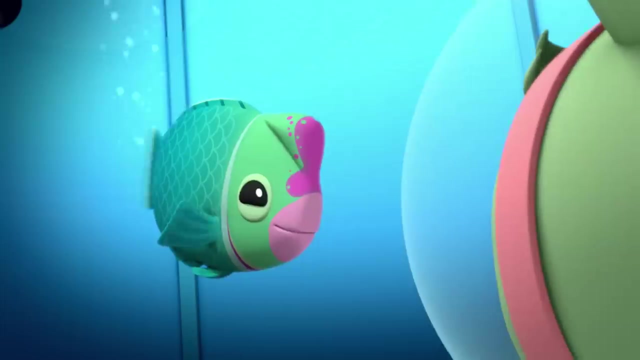 Well, you'd better clear out. A big rock from outer space is about to hit the Octopod. A rock From outer space Sounds delicious. Hold on, Hold on, Hold on. Hold this engine. I reckon you can chomp through that meteor. 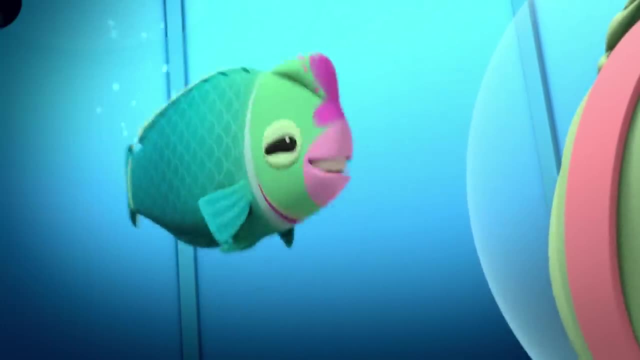 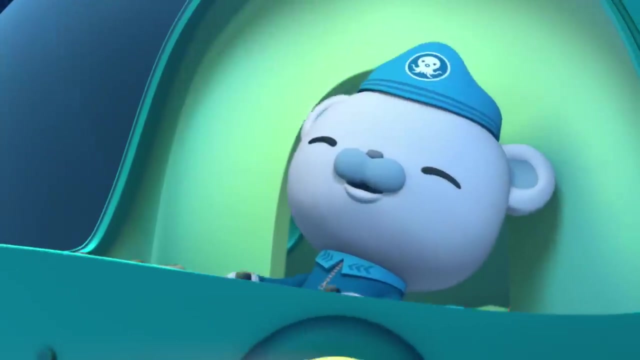 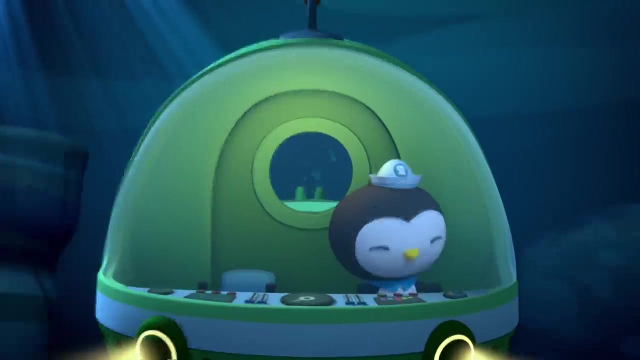 Chomping rocks is my speciality And I've never tasted one from outer space before. Um, do you have any friends around here? Second time, lucky Captain Ready Peso, I can do this. I can do this. 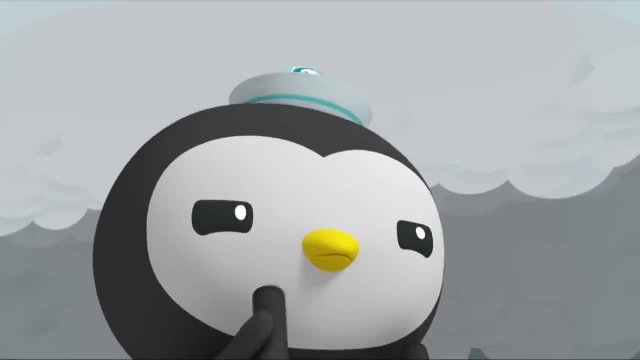 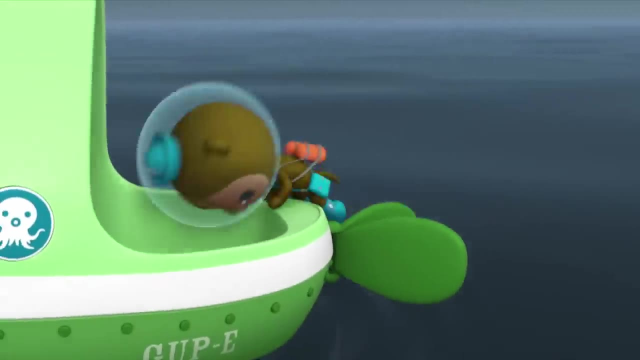 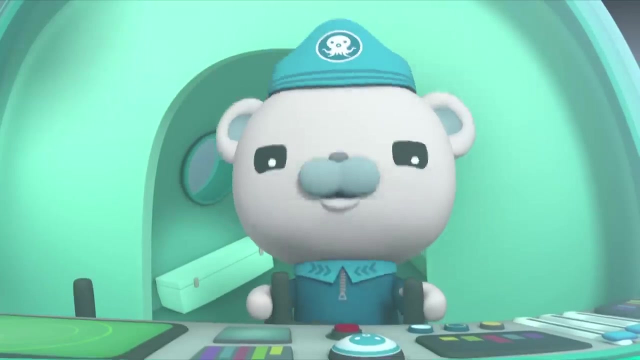 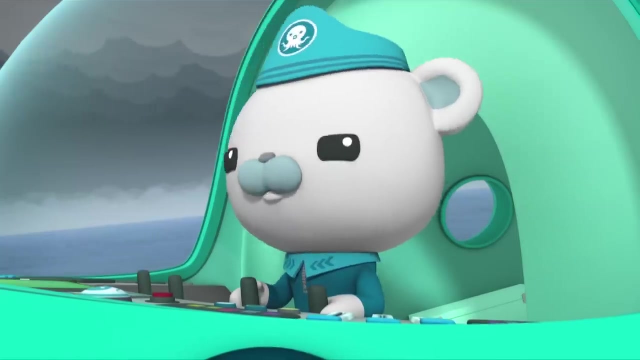 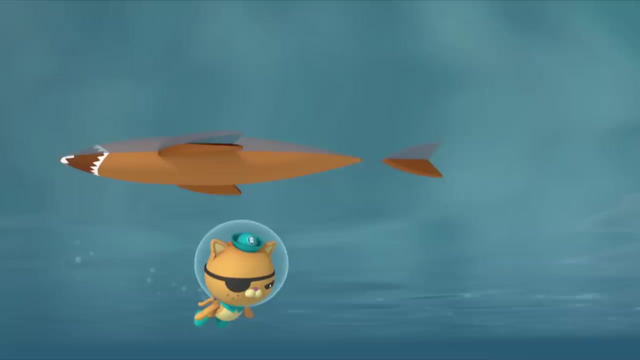 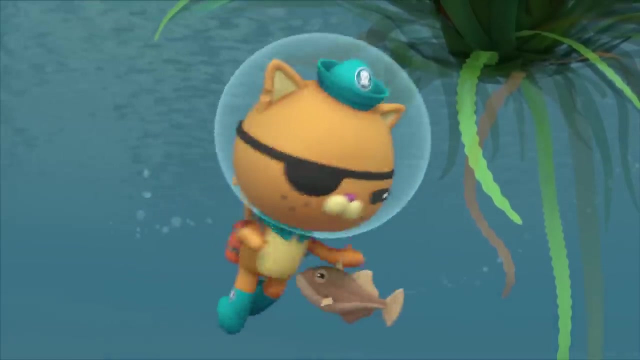 Yeah, Well done, Got it, Shillington hurry. Yes, All down, one to go. Captain, I've found the last float. Try to get it quickly, Quasi, Huh, Oh Hey, Watch it, matey. 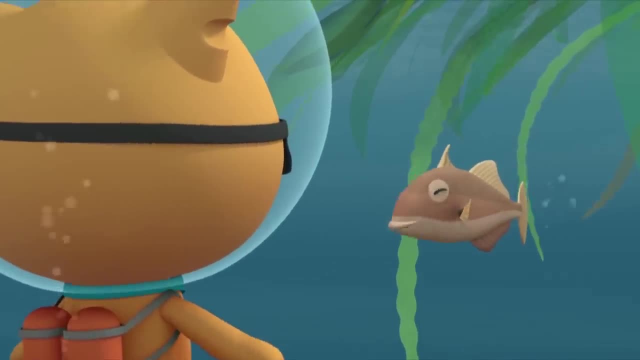 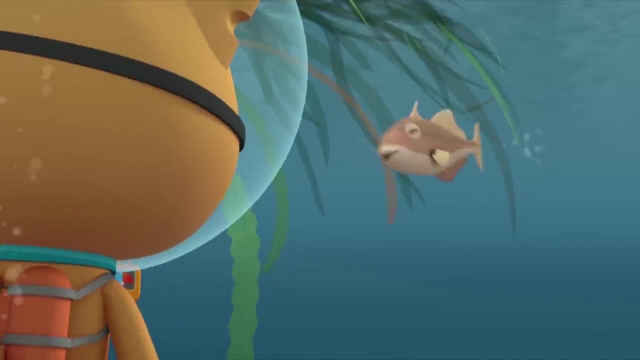 Oi, Who you calling matey? The name's Trixie, I'm Triggerfish And I'm Quasi Pleased to meet you, Trixie, But that's our float And we need it back. Oh no, you don't. I make my home under whatever I find floating on the surface of the ocean. 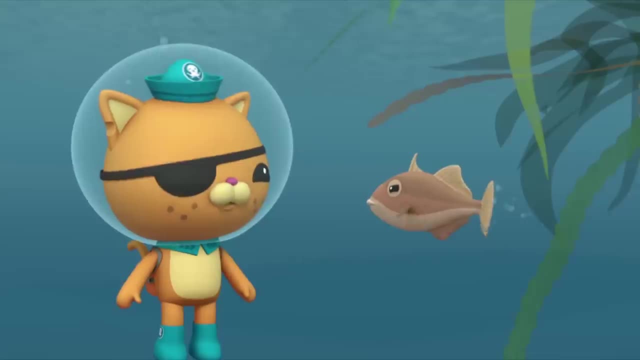 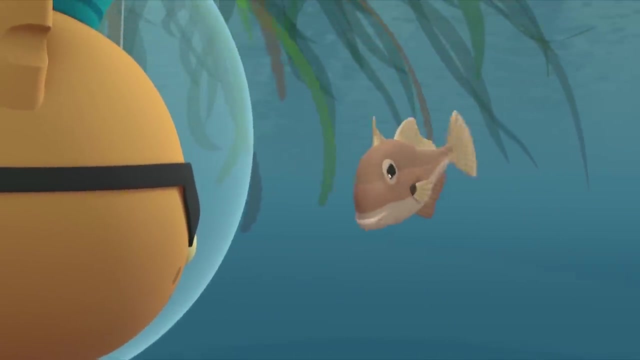 But I can't just leave this float out here. You don't want it littering up the ocean, do you? Oh, I've made a home out of all kinds of rubbish before now. Whatever keeps me safe from the birds up above and the big fish below. 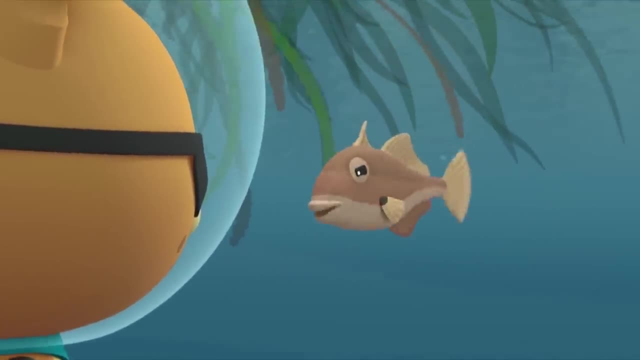 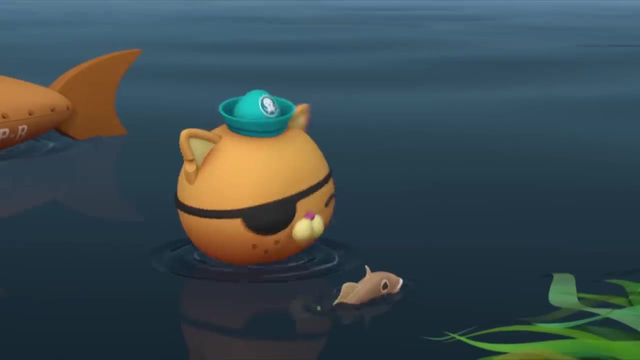 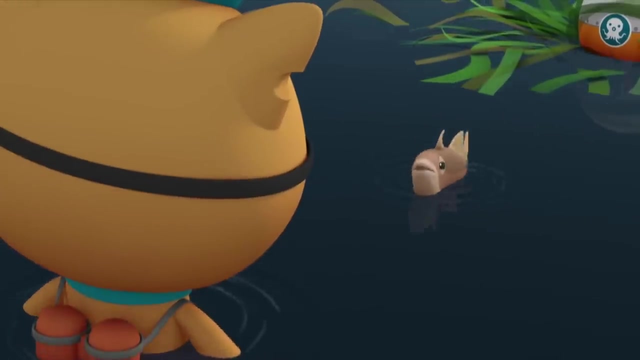 And when I find a home this good, I don't give it up easily. Eek, Eek And fast. There's no time to argue, Trixie. You'd better dive down deeper where it's safe. I'm staying right here. No water spout's going to scare me out of my own. 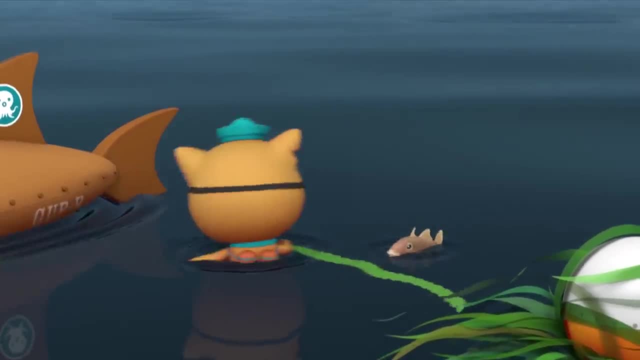 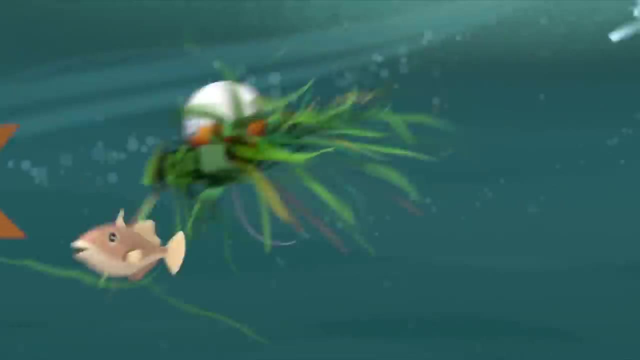 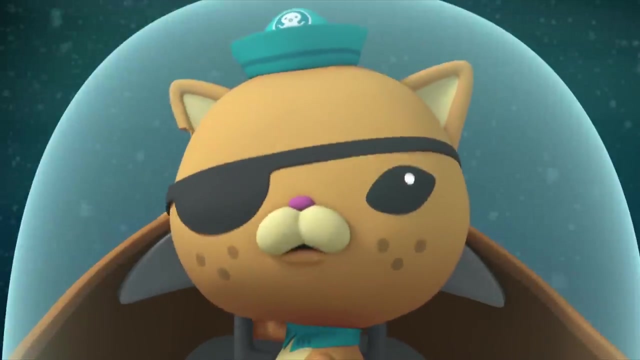 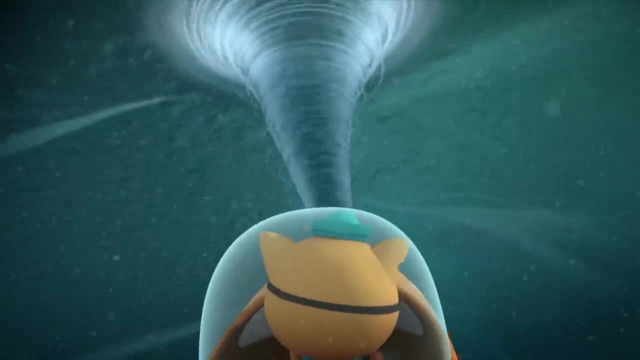 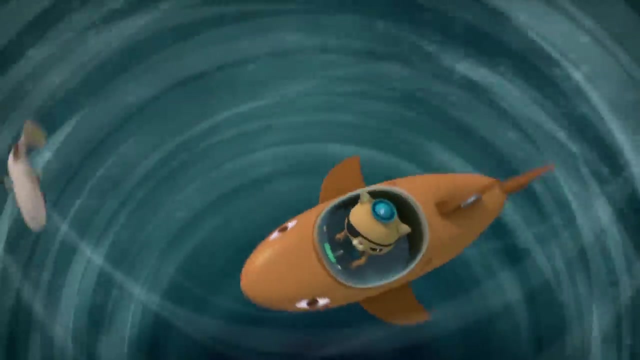 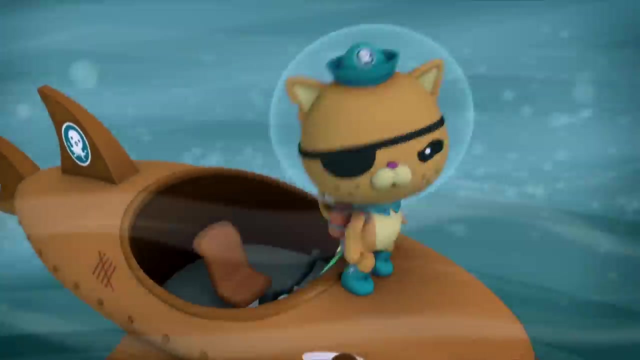 Right, You don't have to leave your home, but I've got to move it to safety. Follow me, Trixie, Trixie, Trixie, I'm coming for you. Trixie, Trixie, Whoa. 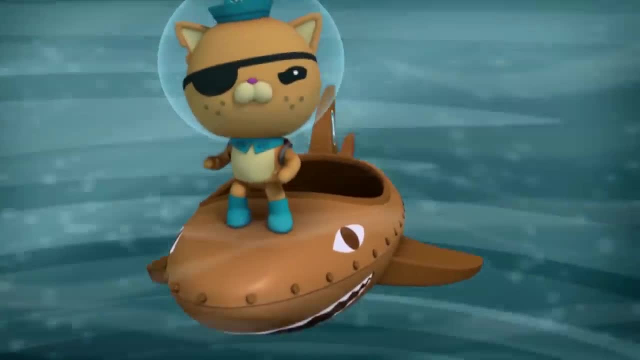 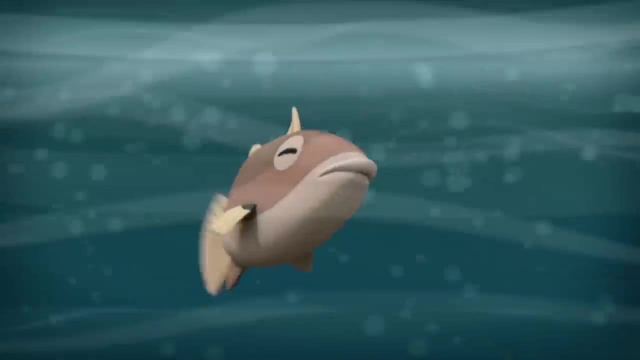 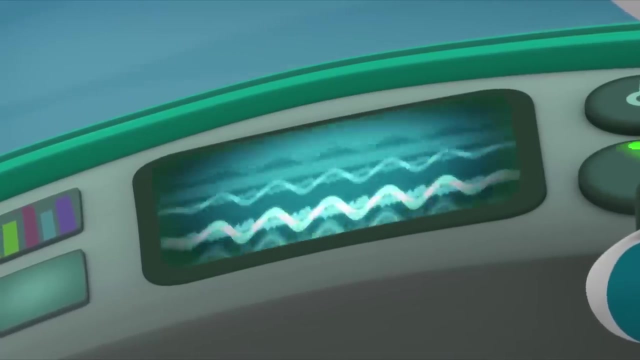 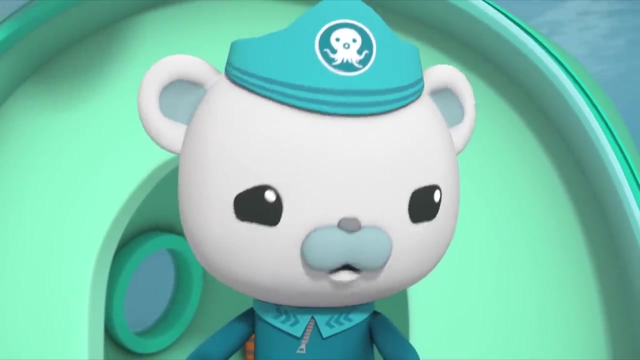 Whoa, Quasi. come in for a joke. Hard talk now, Captain. I'm inside a water spout. You're breaking up, Quasi. I said I'm inside a water spout, Quasi. Hmm, Sounds like he's in there with a pig. 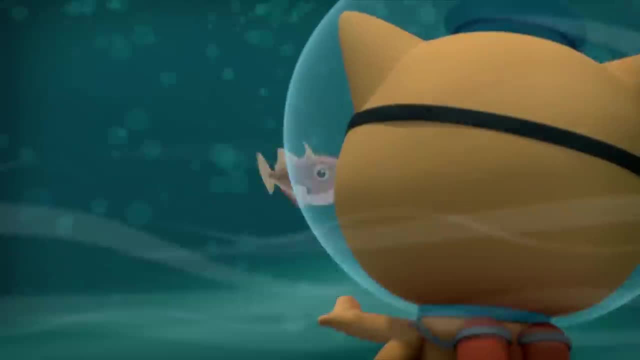 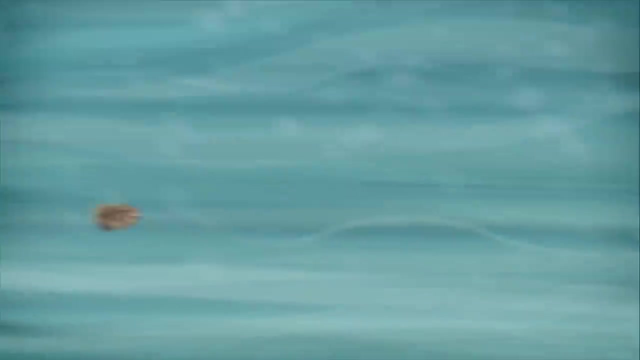 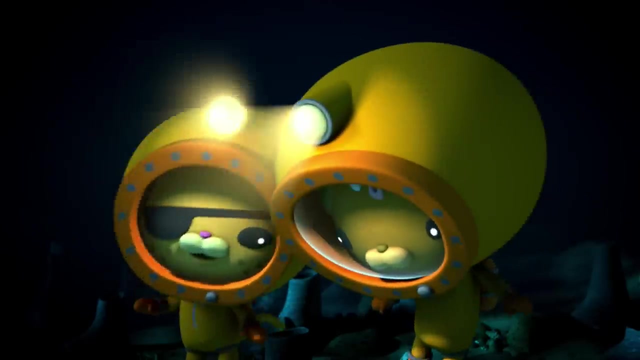 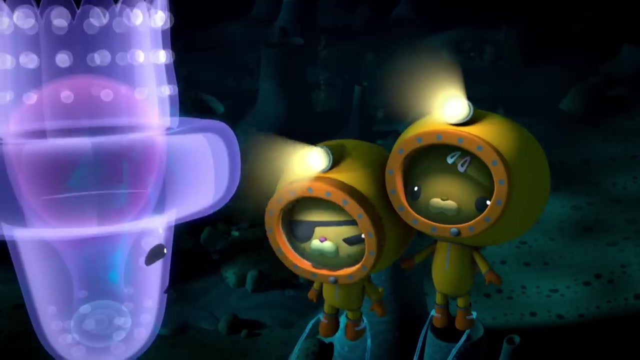 I'll save you, Trixie, Buy me whiskers, I will. Ah, Something's grabbed us. Oh, you mustn't leave. yet We haven't been properly introduced. You're that giant Siphonophore. 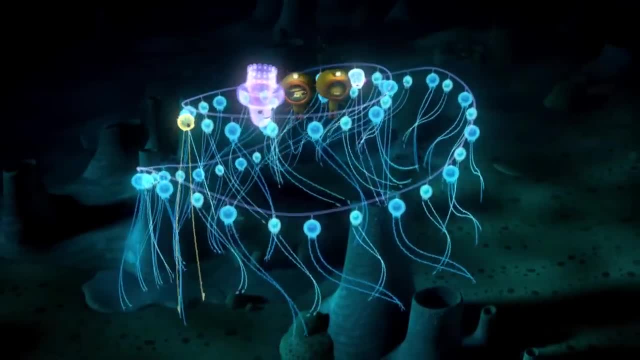 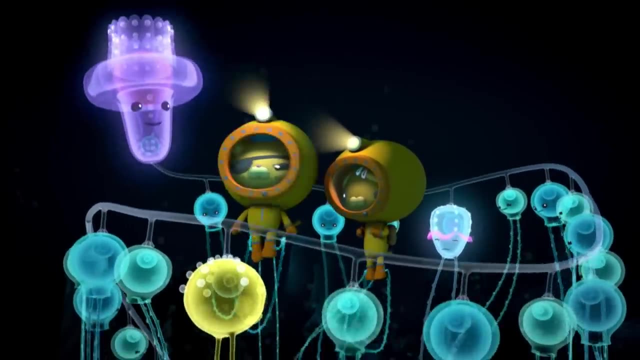 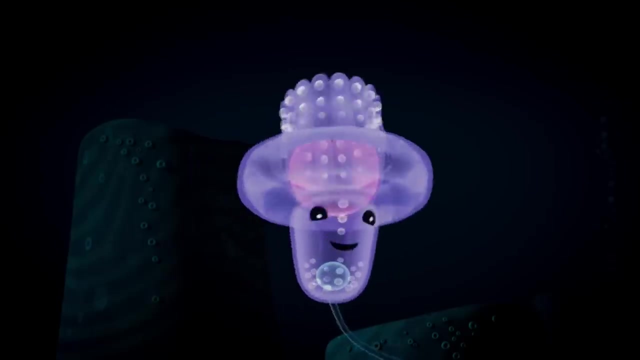 We are the giant Siphonophore. We look like one big creature, but we're actually a group of smaller creatures. We work together. see, Each of us has a special job to do. Some of us can light up Once you follow our lights and get close enough. then 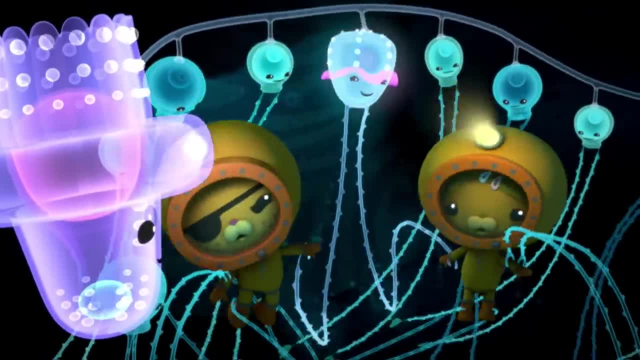 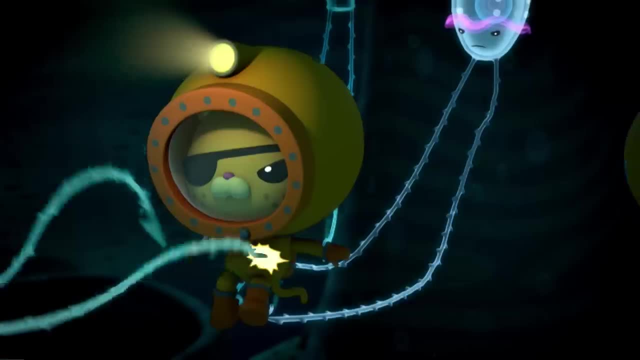 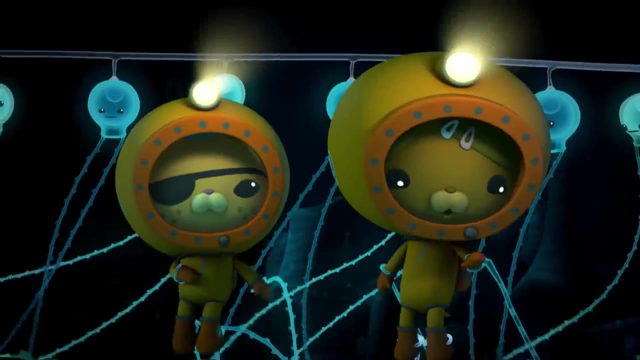 We do our jobs, see. We get our hooks in here, see, And then we use our hands- Powerful stingers- to sting you Like this. What's wrong? What's the problem? What stinging? What's talking? Our deep sea suits are too thick for their stingers to get through. 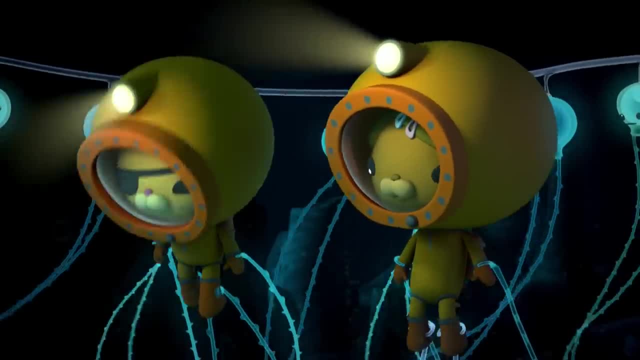 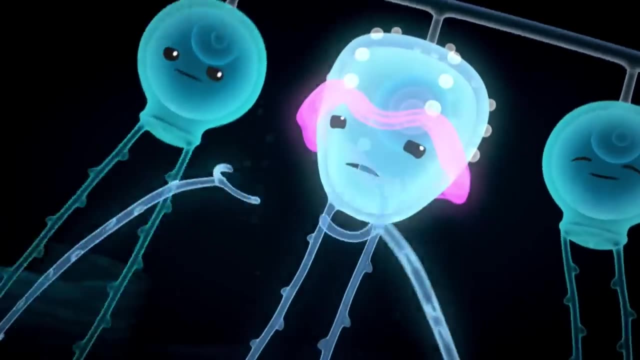 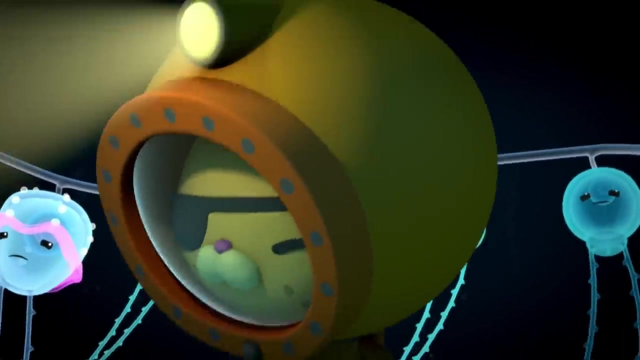 Ha ha, You can't sting us, you scurvy beasties. Bah, This is shocking. Our plan is perfect: Lights, hooks, Stingers, Diggers. Well, you won't be having us for dinner yet. The giant Siphonophore. 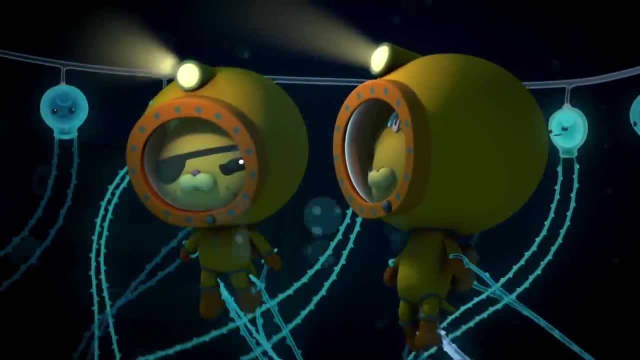 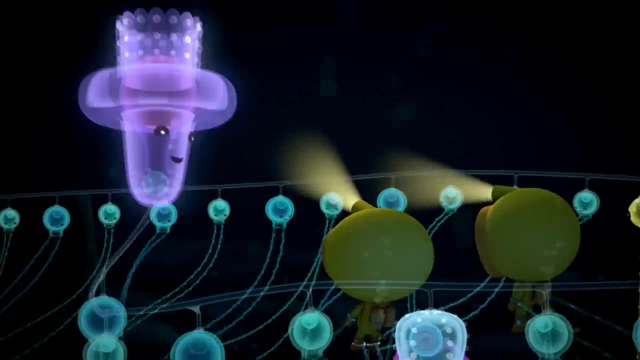 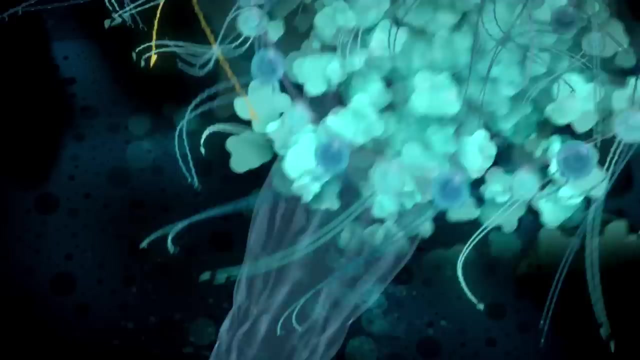 Siphonophore, That's what I said. Another geyser You've got to. let us go and move away from here. Oh, we're not giving up that easily. But we're right on top of a Shiver me whiskers. We're going up. 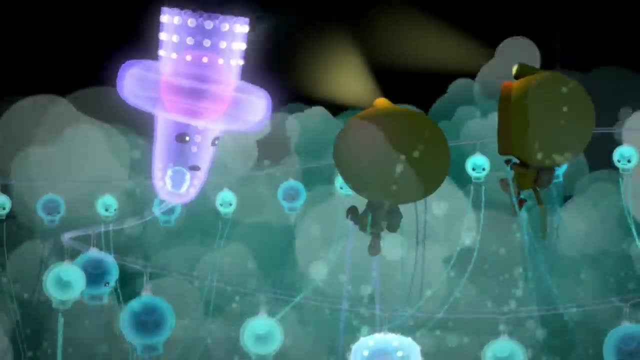 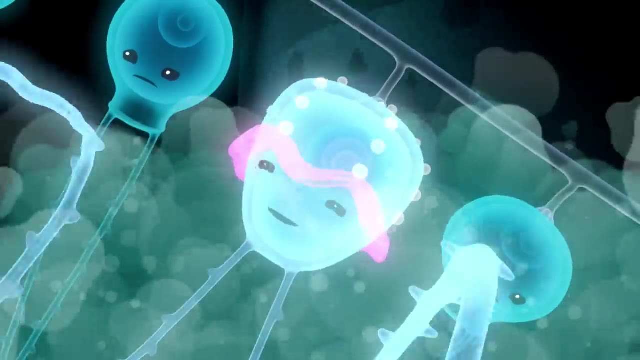 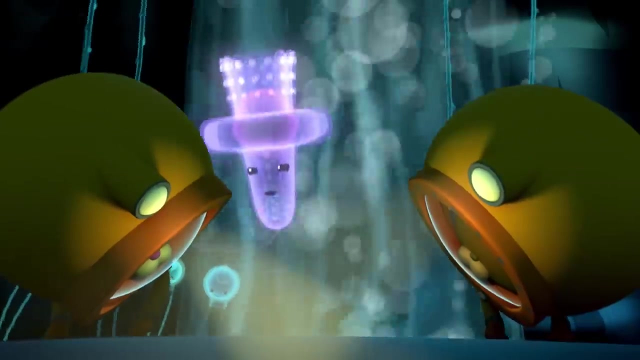 And if you go up too high We'll burst. Let's try to grab that ledge And pull us all off the geyser. Aye, Unhook our arms. Good idea, see, Grab Now. awfully nice of you to save us after our little. 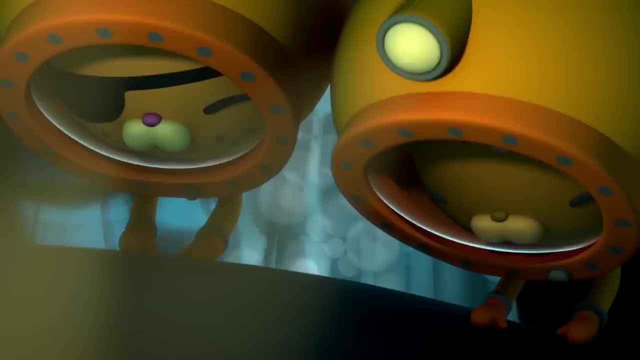 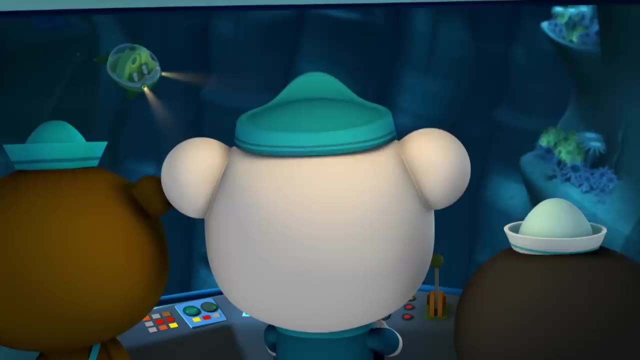 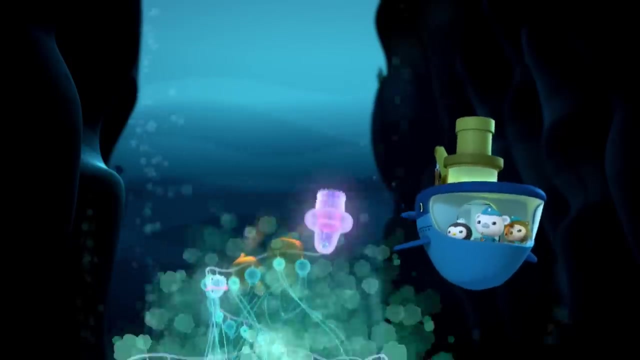 Dinner misunderstanding: Whoa, Whoa, There's the Gump, But I can't see Dashie or Quasi. And something else is on its way up: It's the Siphonophore. Captain Need help, No. 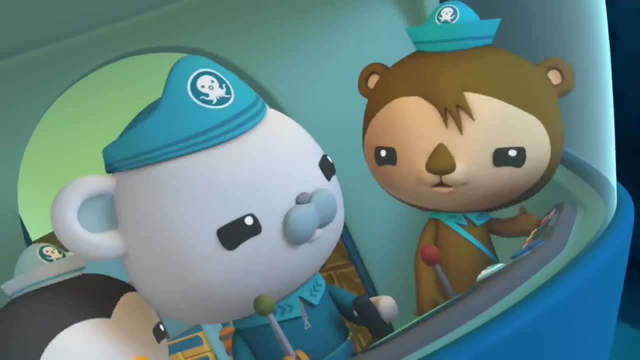 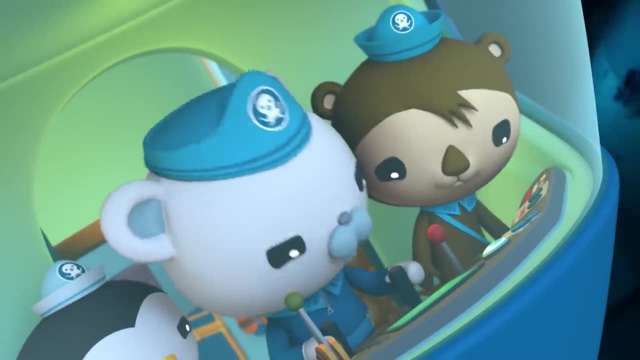 We're trapped in a geyser. No, Meet the Giant Siphonophore. The Giant Siphonophore is going to. I'm a Siphonophore, He-he-he, He's a giant Siphonophore. 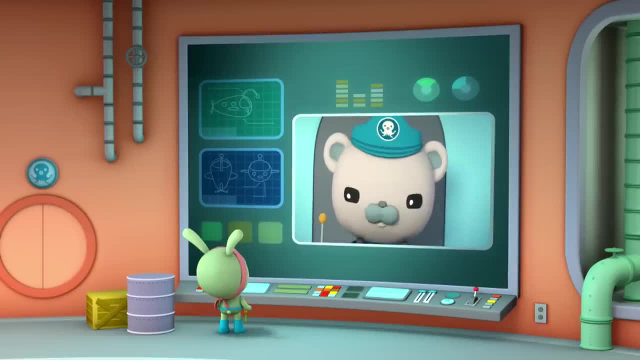 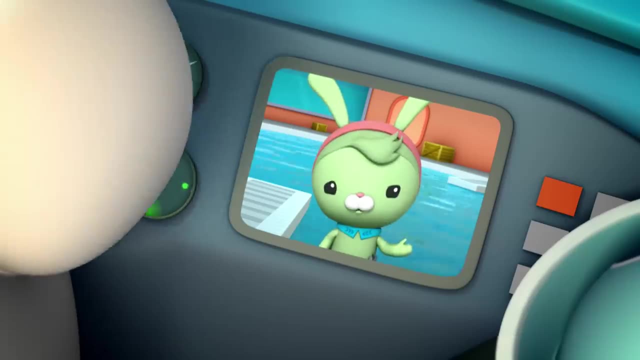 A giant Siphonophore. eigentlich it's A giant Siphonophore, yes, But It's the Gump. It's a Gump, It's the Gump And it has A giant Siphonophore. 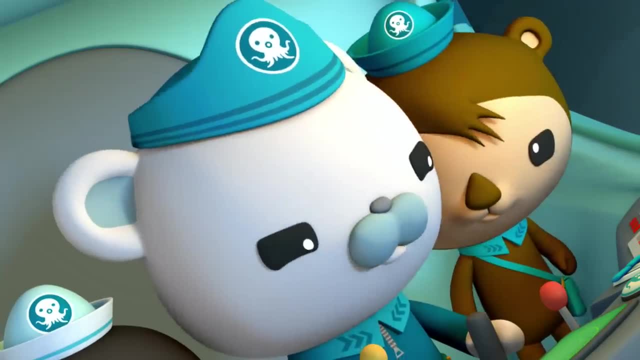 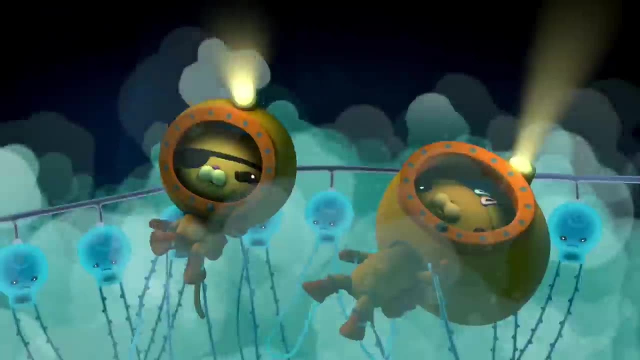 No, It's the Giant Siphonophore. Good plan, Tweed Hurry Got it. Cap, Hold on everyone. Oi, Captain, We don't really have a choice. Tuna, while I put the bubble engine in reverse. 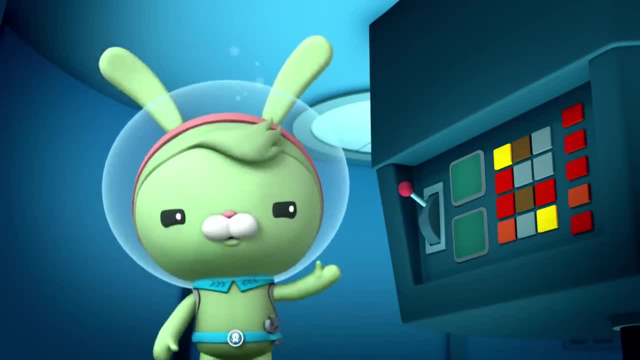 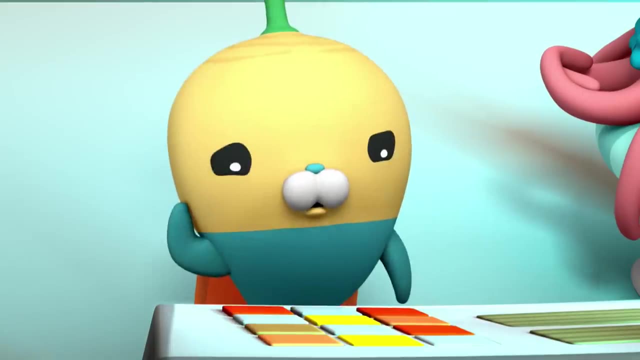 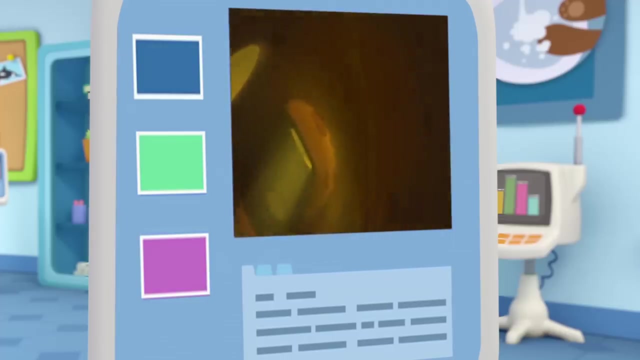 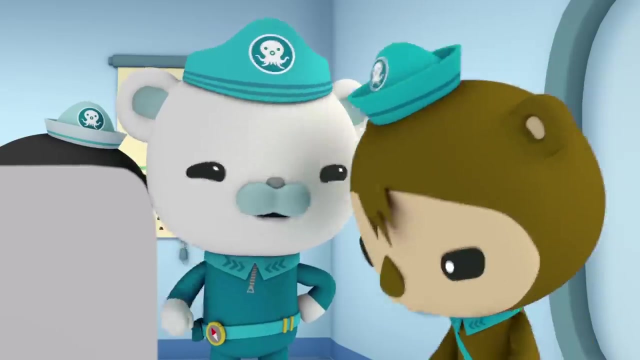 you need to move the octopod, so it's right over the trench. Just there, That button. Oh, Having a look in note. See anything yet, Peso, Ah-ha, Chellington, what is that creature? 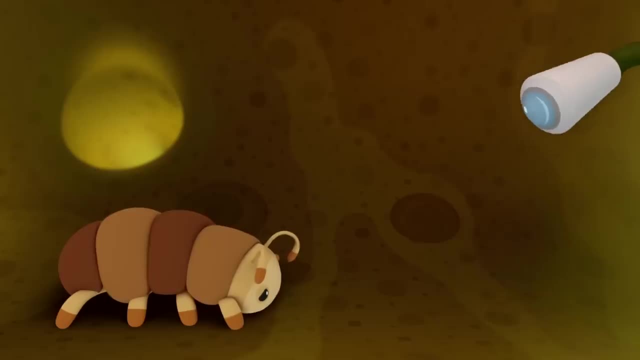 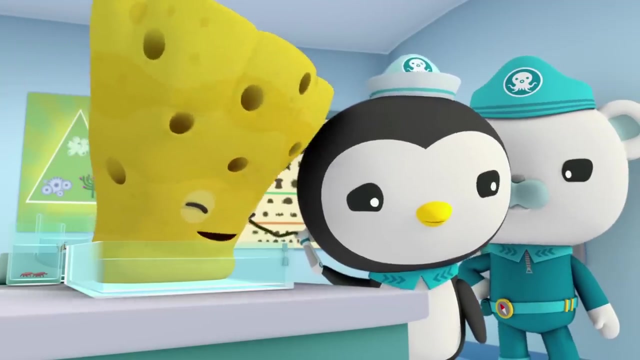 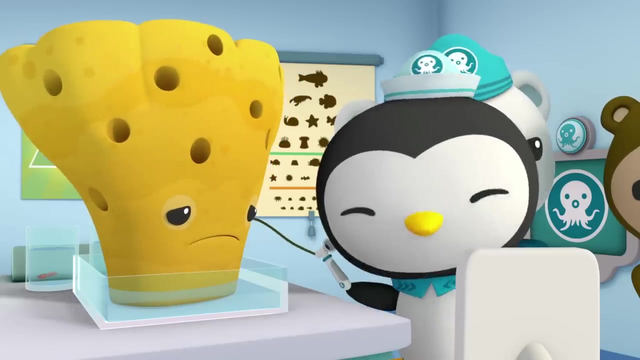 It looks like a louse, A whale louse. What are you looking at? A louse? No wonder I'm feeling so lousy. That thing doesn't belong inside of me. You're telling me He doesn't look like he's feeling very well either. 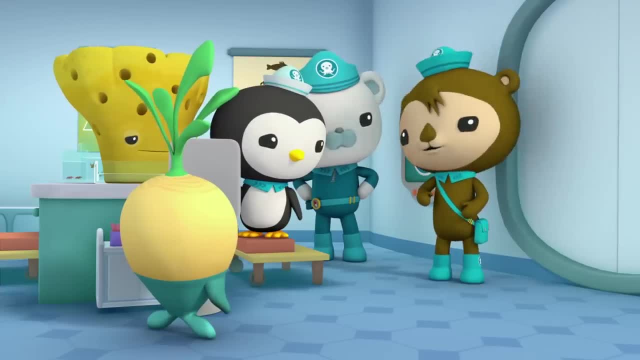 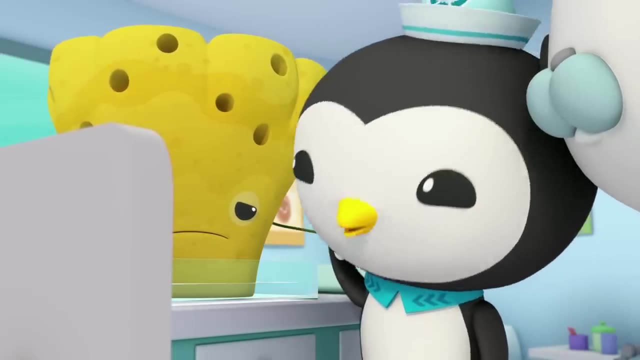 I've found something. Of course he isn't. Whale lice can only survive on whales, not inside sponges. Excuse me, Mr Louse, but we need to get you out of this sponge right away. Oh no, No way. 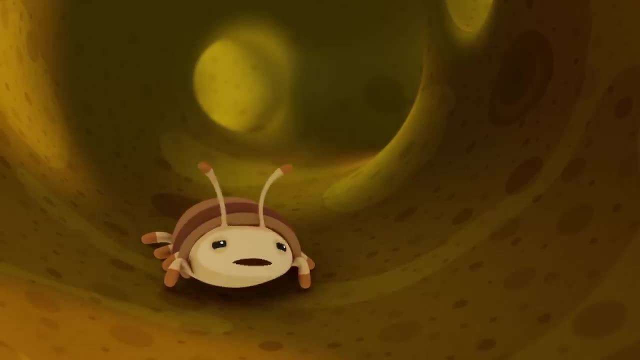 I'm a whale louse. I ain't leaving until somebody finds me a whale to live on. Captain, the sponge won't feel better until the louse is out of her and the louse won't feel better until he's back on a whale. 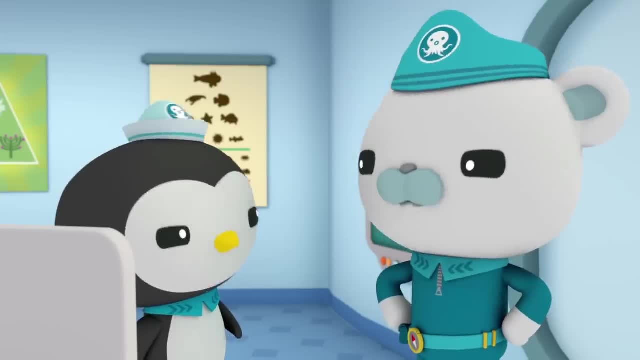 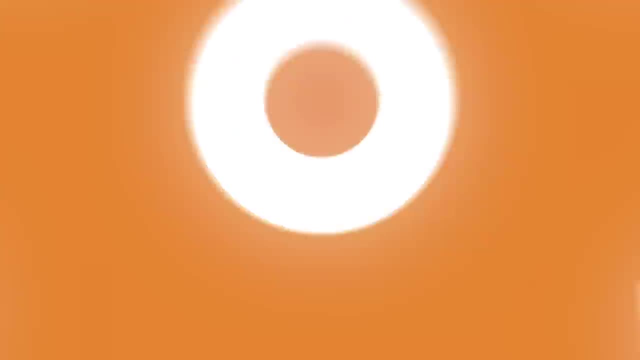 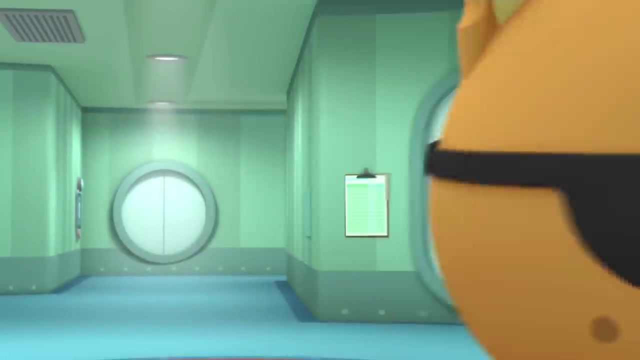 Then there's only one thing to do: Peso sound the octo-alert Octonauts to the HQ Octonauts. we have to find a whale for a sick whale louse, And we need to find it fast. 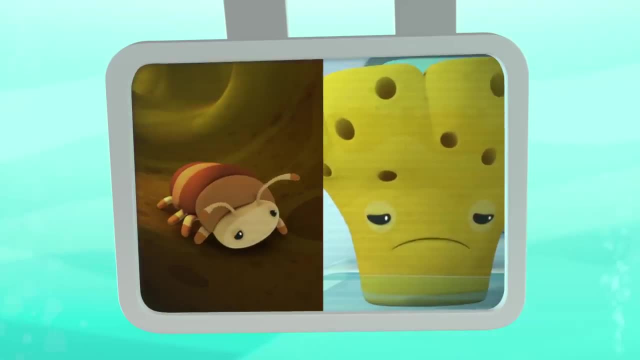 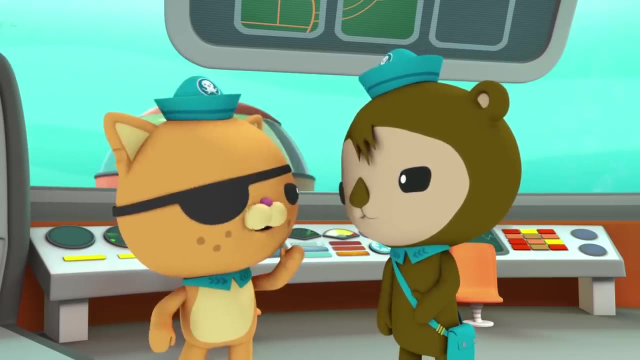 Both the sponge and the louse are feeling worse and worse. Oh Ah, there'll be plenty of whales swimming these waters. We'll find the nearest one and give the little castaway a home to call his own. Oh, it's not that simple, Quasi. 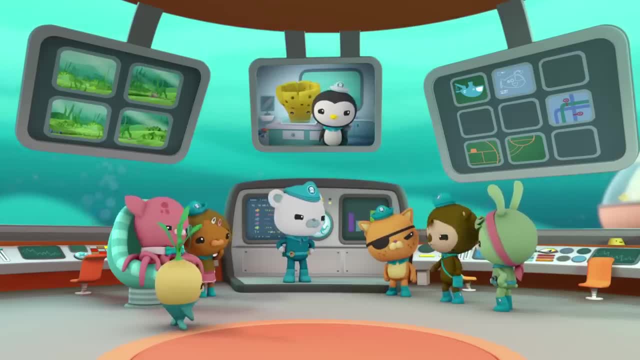 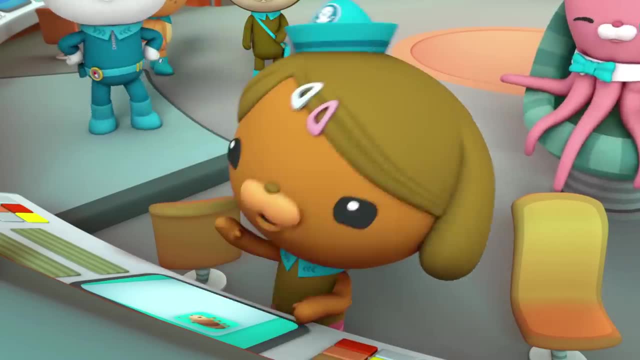 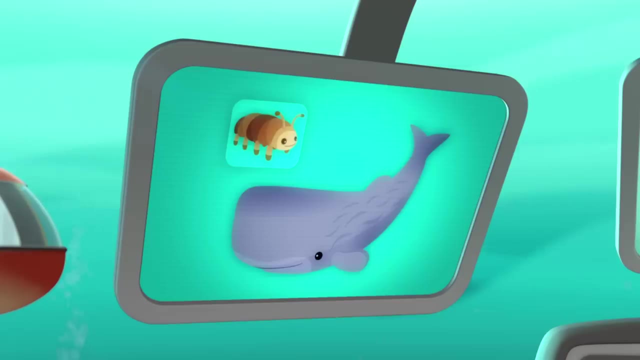 Different kinds of whale lice live on different kinds of whale. We have to work out which whale species this louse came from. I'm running a scan now. There Looks like this louse came from a sperm whale. There's no time to lose. 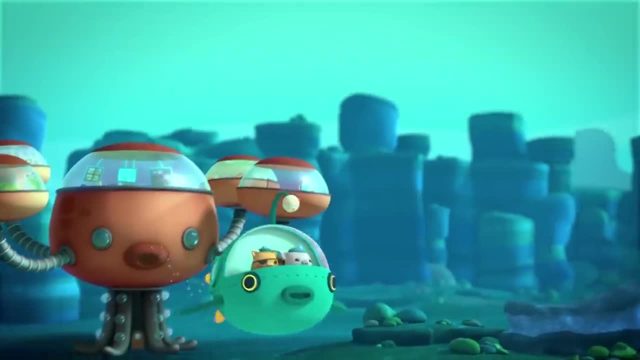 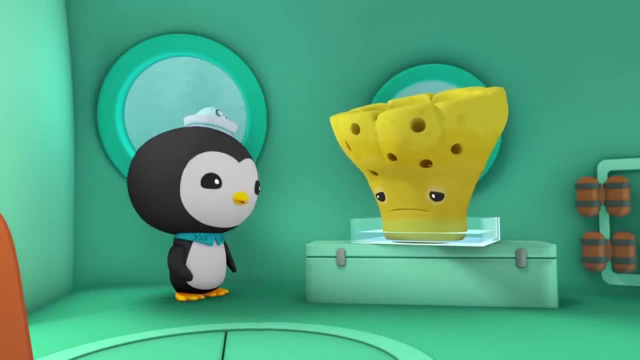 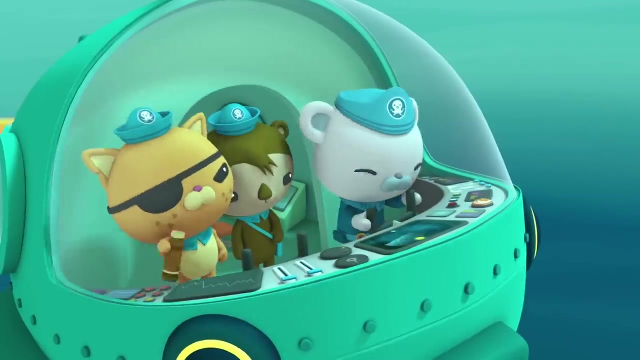 Octonauts, let's do this. Don't worry, We'll have this louse out of you in no time. just as soon as we find him a sperm whale, There's something big coming up. Avast, It's a whale. 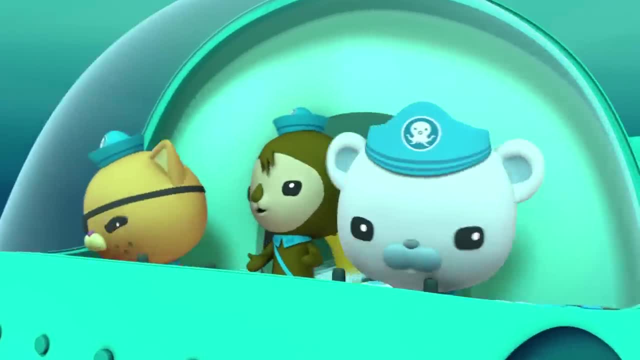 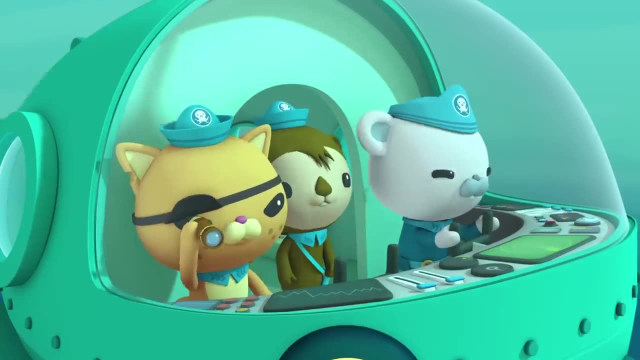 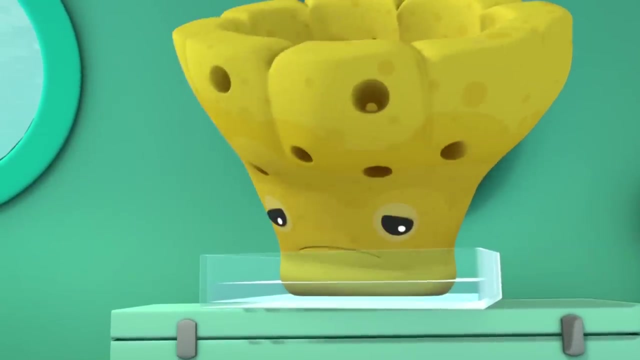 Oh, but it's a blue whale, not a sperm whale. Hmm, Keep looking. everyone There. Nope, that's a humpback whale. I knew that I'm starting to feel a little faint. Oh, you're feeling faint. 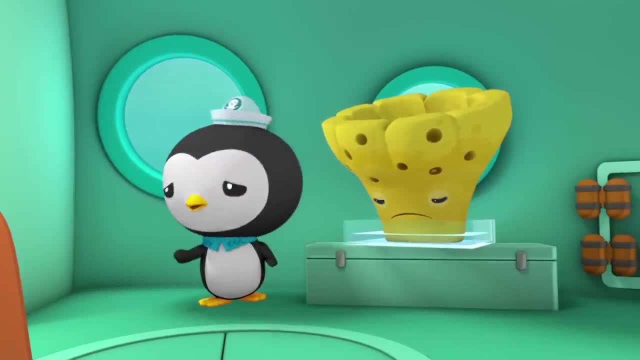 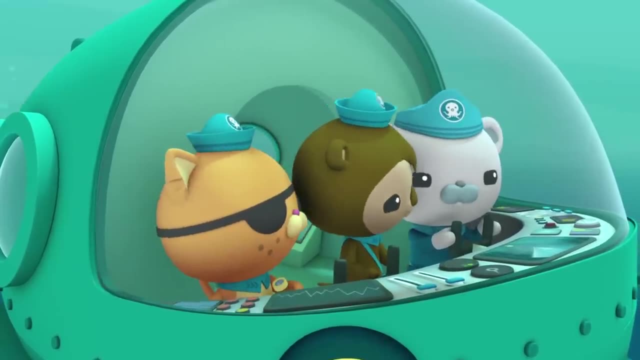 How do you think I feel Hurry, Captain? They're getting worse. We're coming up on another whale now. Uh, I can't tell what kind it is, Captain. It's uh, it's uh, a sperm whale. 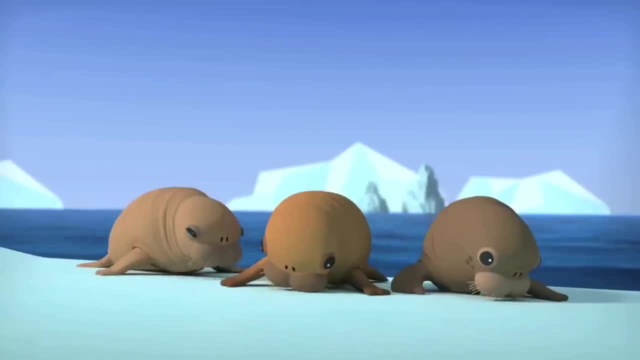 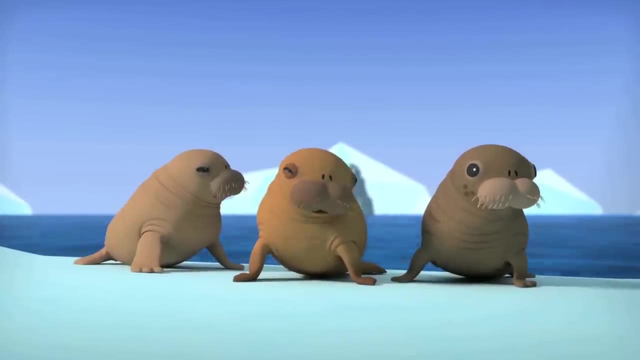 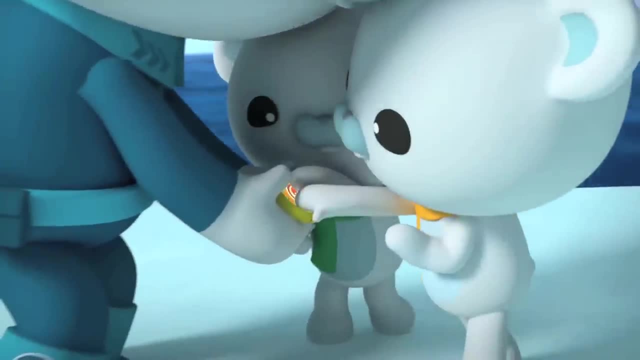 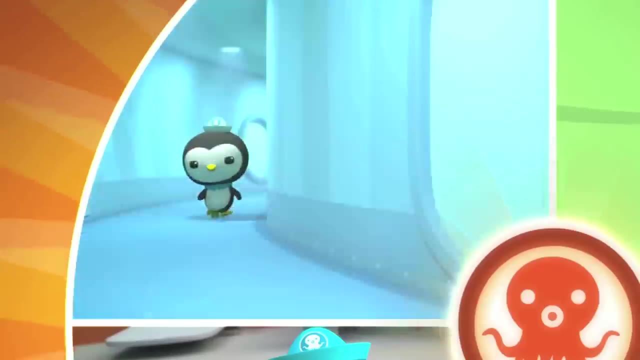 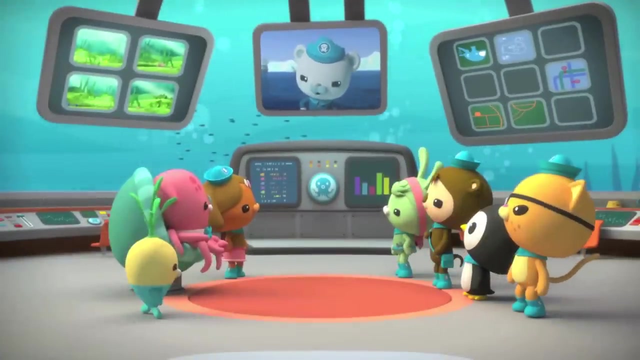 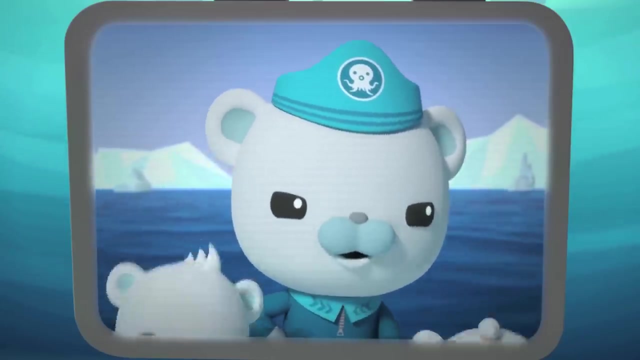 Cubs, would you Sound the auto alert? Octonauts to the HQ Octonauts. the cubs and I are on a runaway iceberg with three walrus pups. The pups are too weak from hunger to swim very far And we've got to sound the octo alert. 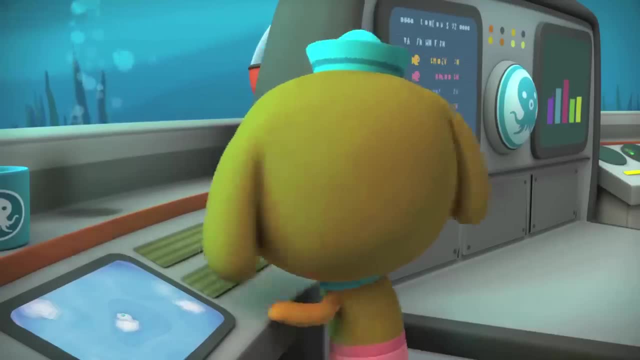 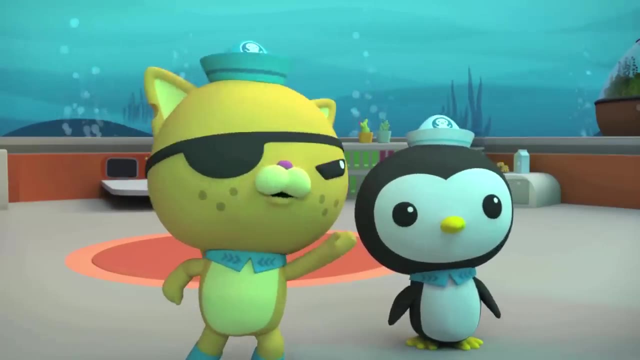 We need to get these walrus pups to safety. Captain, we've located your iceberg. We'll be there as soon as Shiver me whiskers. You're on a crash course with two other icebergs. Oh no, When the icebergs crash into each other, you could all get hurt. 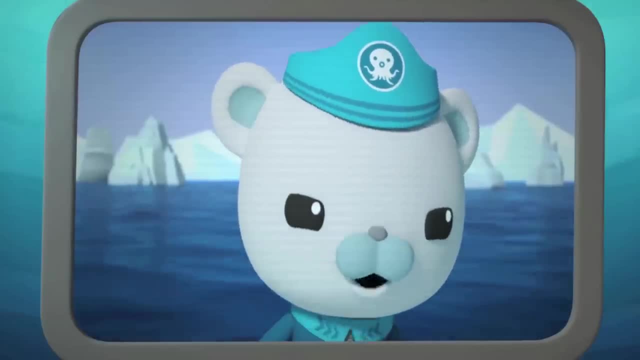 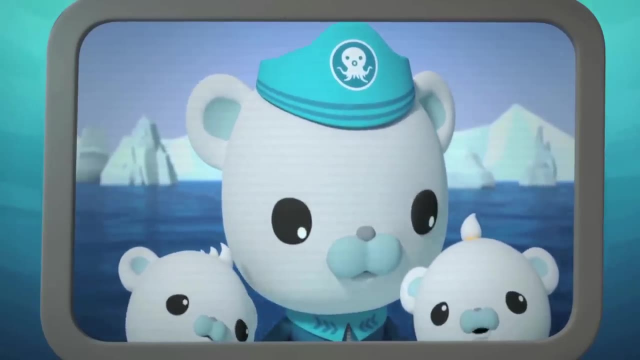 Quasi Peso. take the Gup S and catch up to us as fast as you can And please bring something for the walrus pups to eat. They're really very hungry. Tunip, you and the Vegimals can help me prepare some bottles of walrus pup formula. 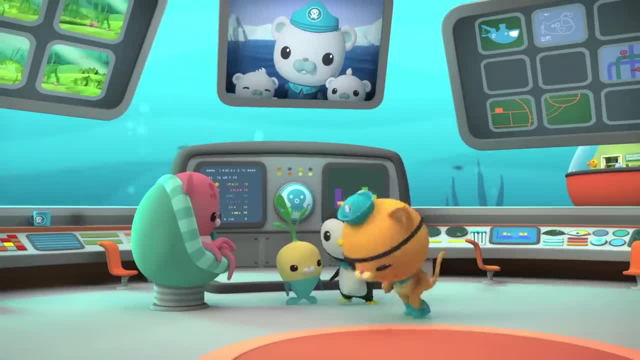 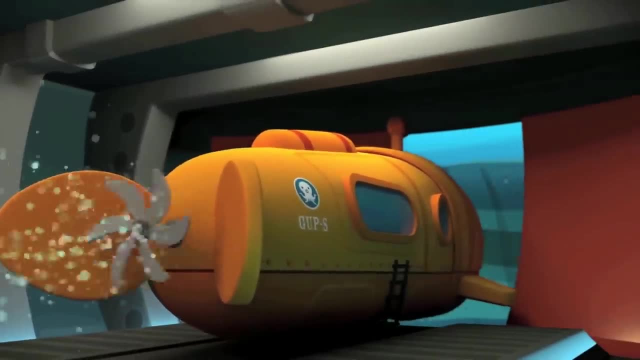 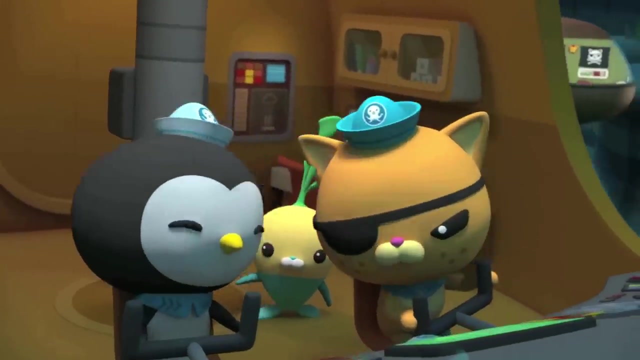 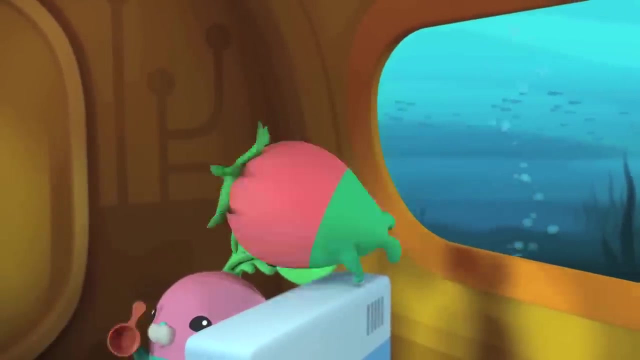 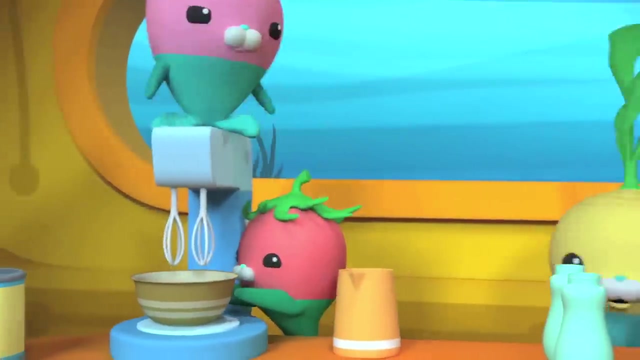 We're on our way, Captain, To the Gup S mateys. We'll catch up to that iceberg and fast Ready to mix up some walrus pup formula. Robble, robble, Ah, Chubba, chubba. 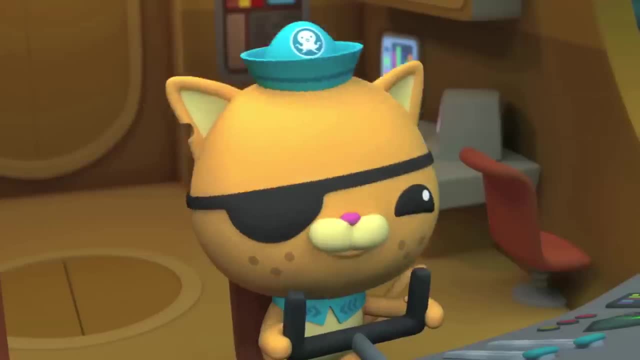 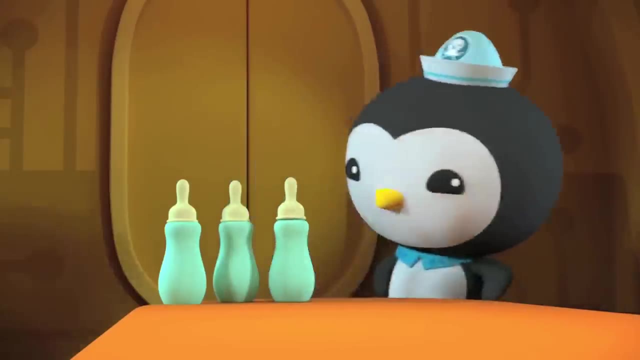 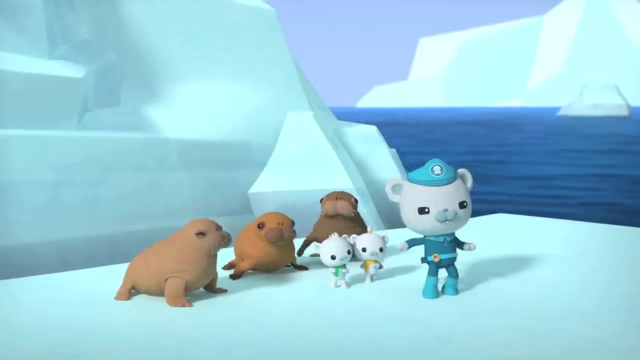 Chobbaba, chubbaba, Chubba, chubba, Ta-da, Ta-da, Chubba. That iceberg's getting really close, Too close. Move to this side, everyone Now. it's really very close. Hold on everyone. This could get bumpy. 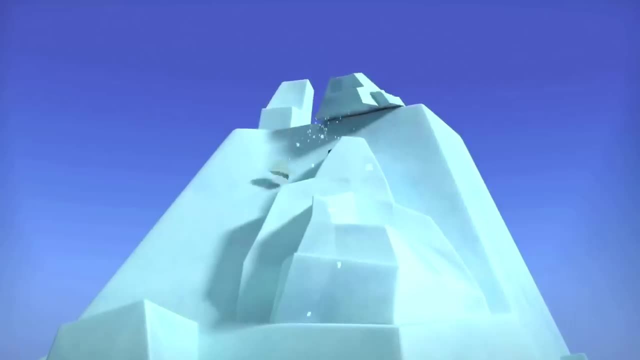 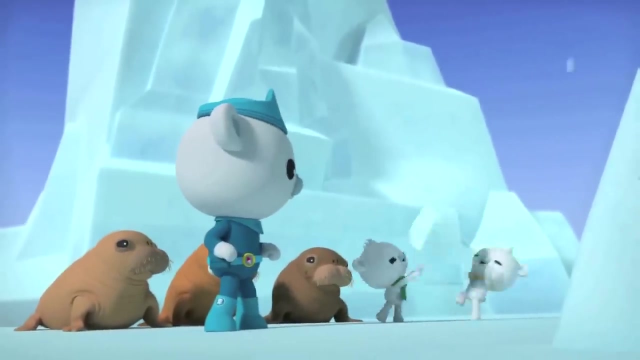 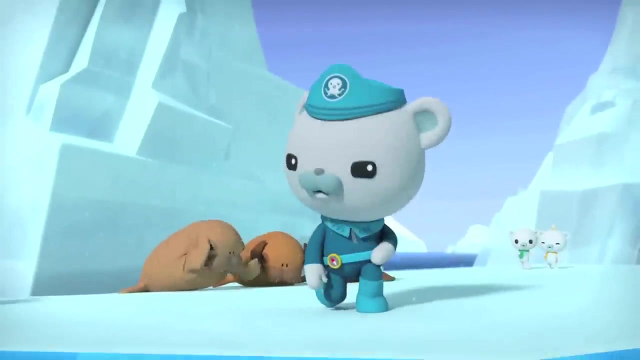 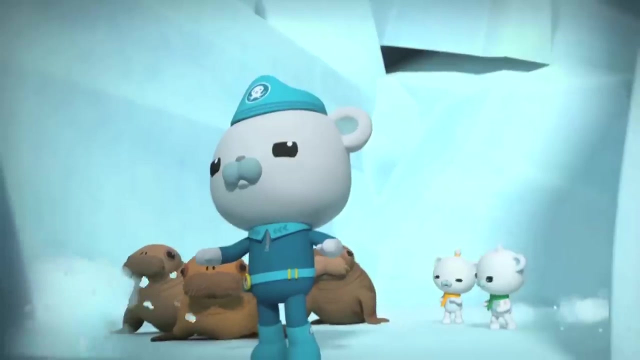 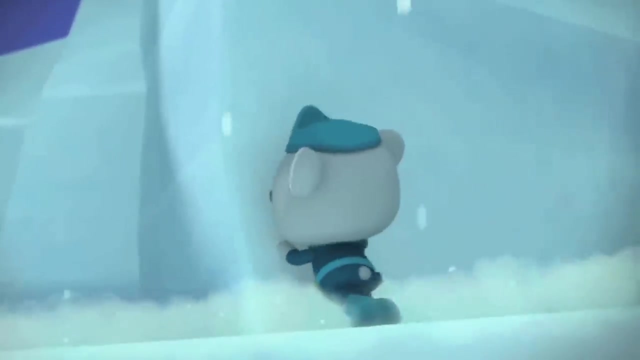 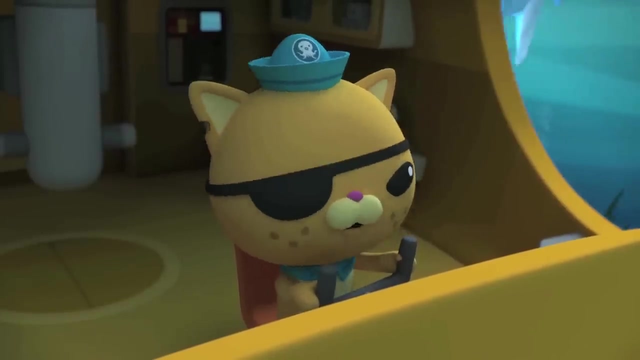 Whoa, We've got it. Well done, Cops, Watch out, Got it Everyone. move back Bonnacles to Quasi. Are you getting close? We're under the icebergs now, Captain, It looks like you're trapped right in the middle. 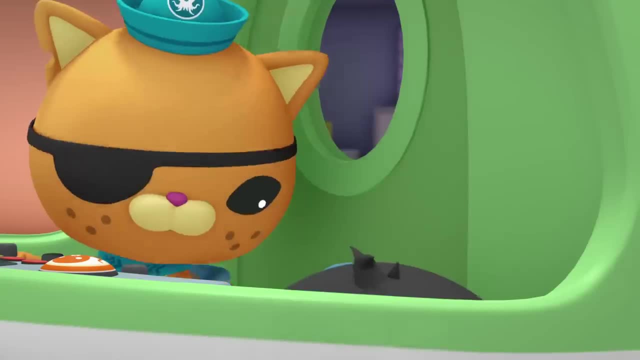 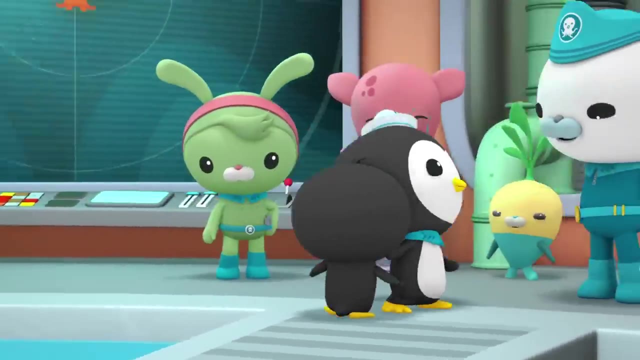 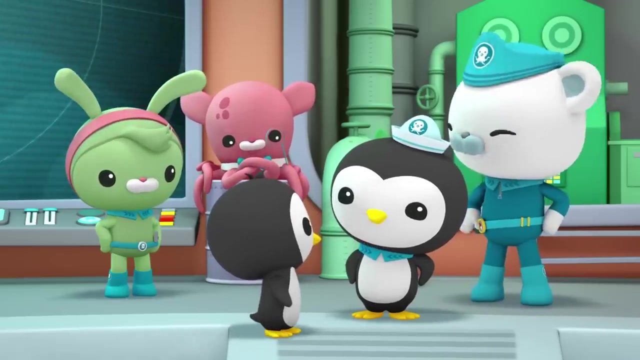 Here we are: The Octopod Pinto Peso, Captain Bonnacles and my fellow Octonauts. this is my little brother Pinto. Welcome aboard, Pinto, Thanks. This is Professor Inkling, Tunip and Tweak. 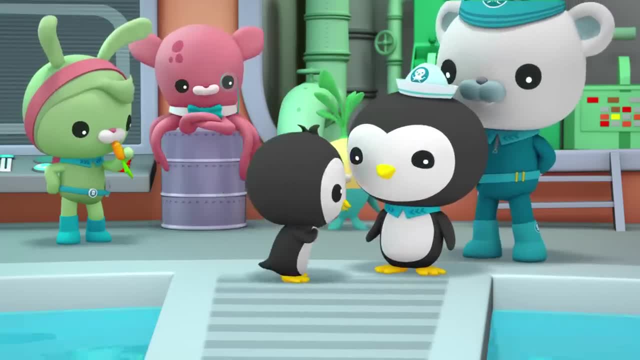 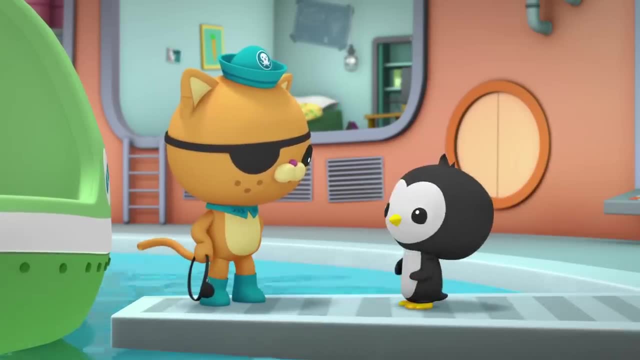 Hi, Was your trip? okay, It was the best ride ever. Quasi taught me how to talk like a pirate. Aye, matey, Shiver, me flippers. This is for you. me hearty Welcome aboard the Octopod. 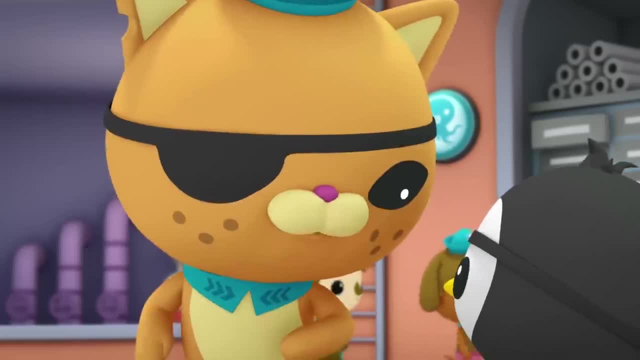 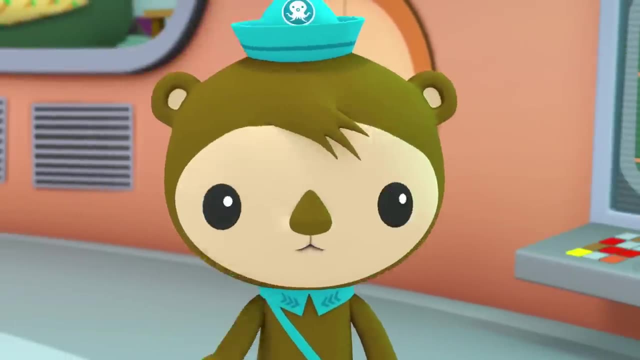 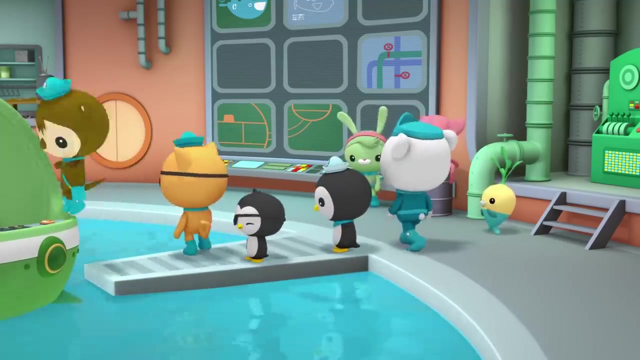 Do I look like a real pirate? Yow Yow, I'm ready for action. And this is Dashie and Shellington. Hello, It was great to meet you, Pinto. We'll see you when we get back. Are they taking the Gutt-E on a real mission right now? 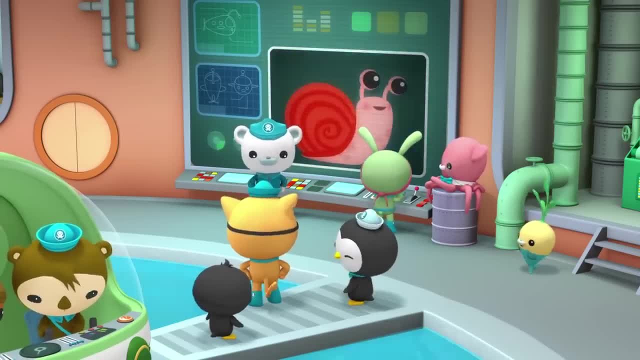 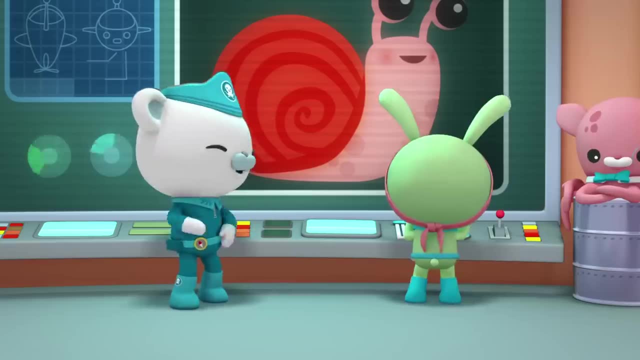 Yes, They're going out to study baby sea snails. Baby sea snails can be hard to find because they're so tiny. That's why I have my magnifying glass Tweak open the octahatch. Aye, aye, Captain. 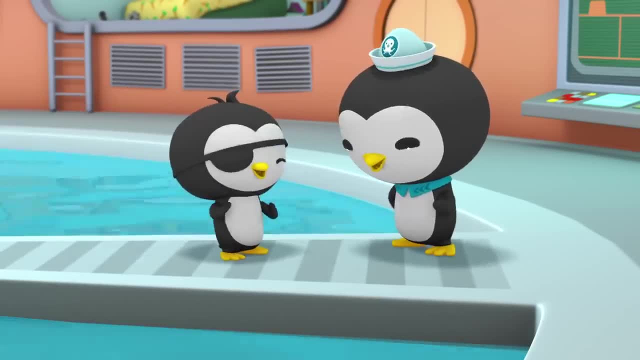 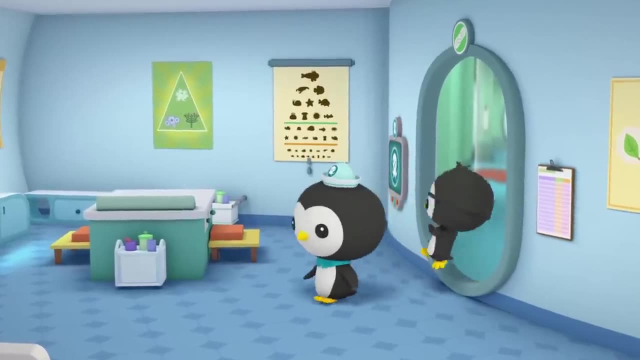 I want to go on a mission too. Let me show you around the Octopod. first, Quasi told me that the life of an Octonaut is really exciting. Oh, it is. As a medic I Do. you search for sea monsters like Quasi. 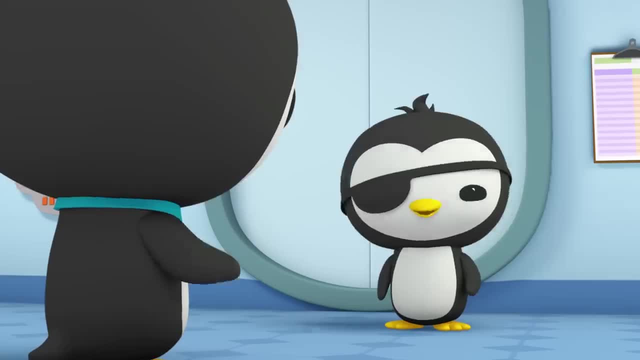 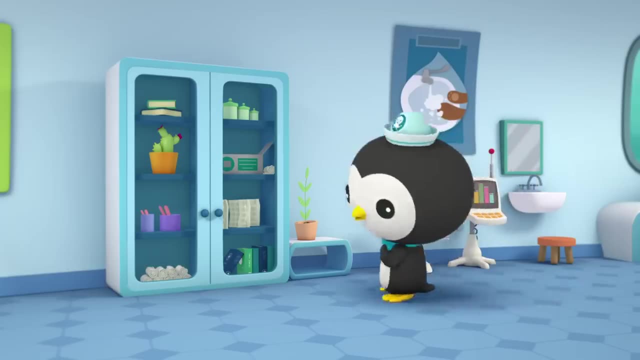 Er? well, here Let me show you what I do. I And Quasi says that an Octonaut has to be prepared for anything to happen. That's true. You want to try doing something that I do? I'm ready for anything. 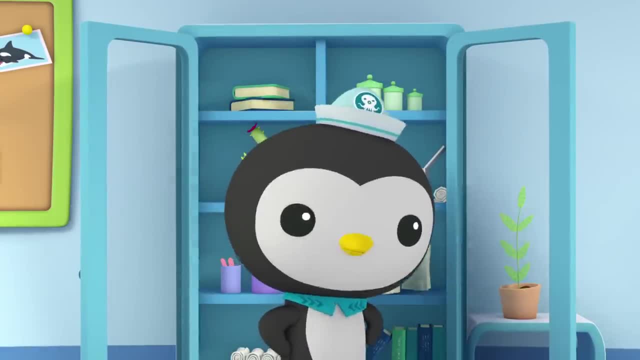 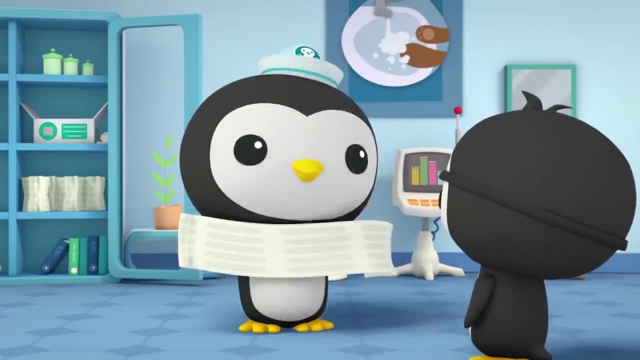 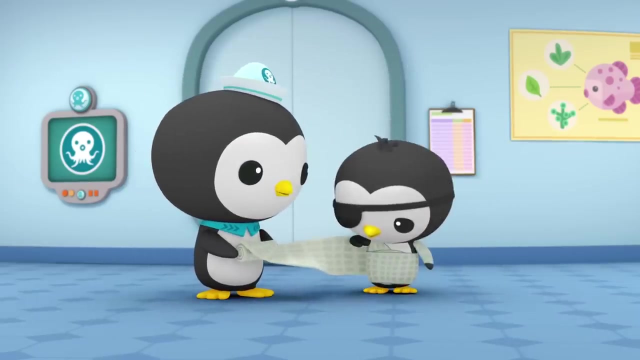 All right, then Here's a real challenge: Bandaging. We'll practice a combination bandage: A flipper sling and a rib wrap. Now you try it. I want to learn how to be an Octonaut- not a medic, But I'm an Octonaut and a medic. 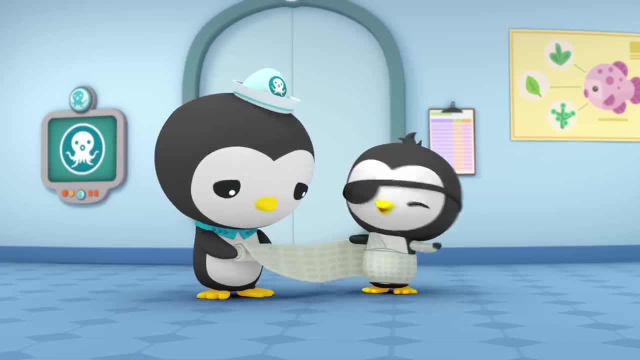 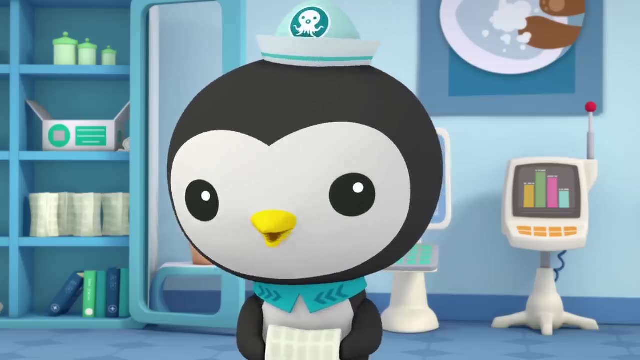 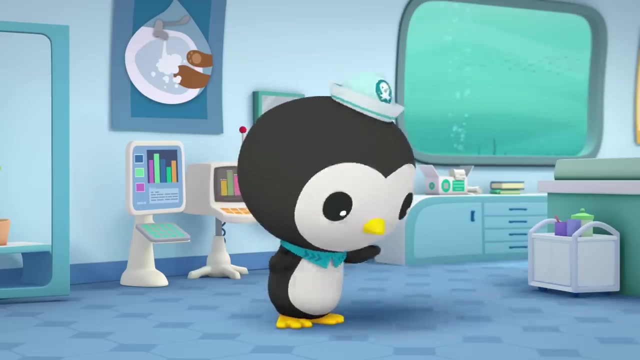 I mean a real Octonaut Like Quasi, Ready for action. Oh, I have to be ready for action too, you know, In case something happens, In case someone gets hurt, Quasi, Wait, Is the shop under attack? 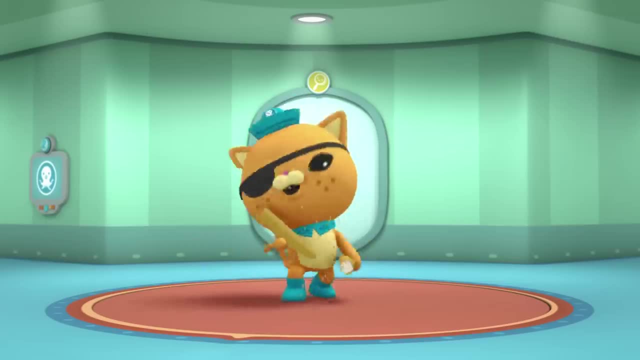 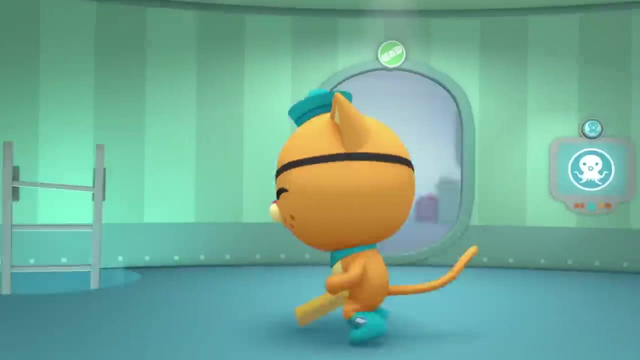 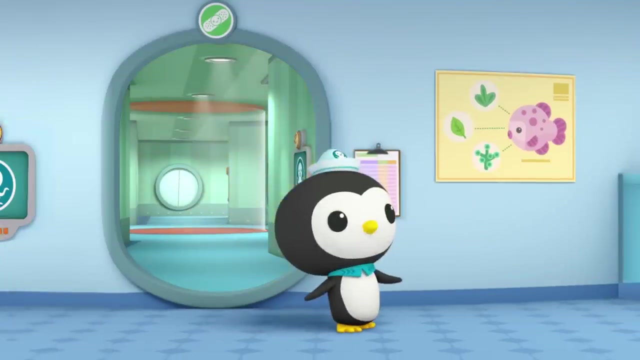 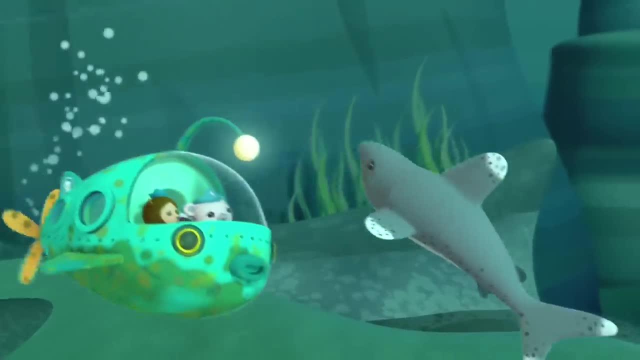 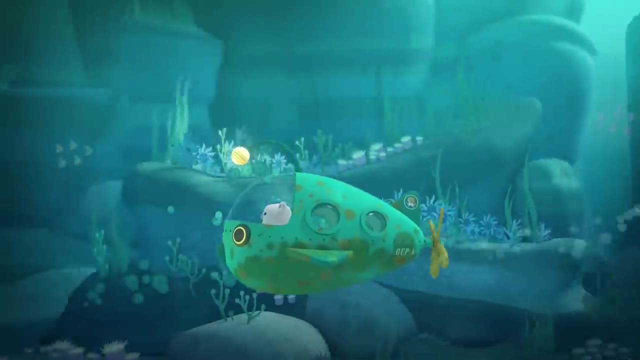 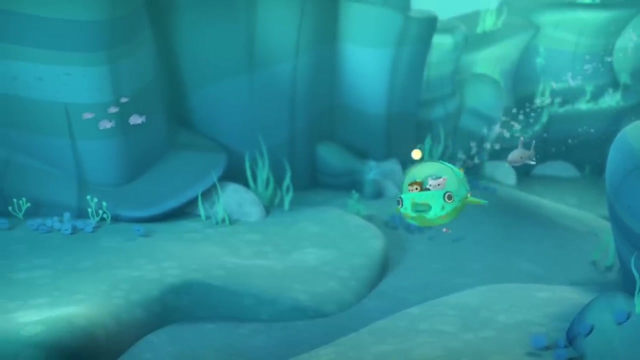 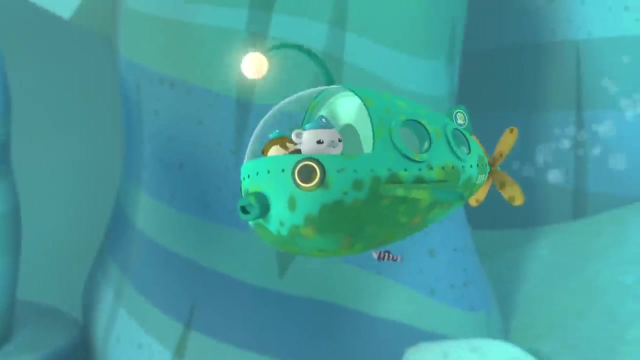 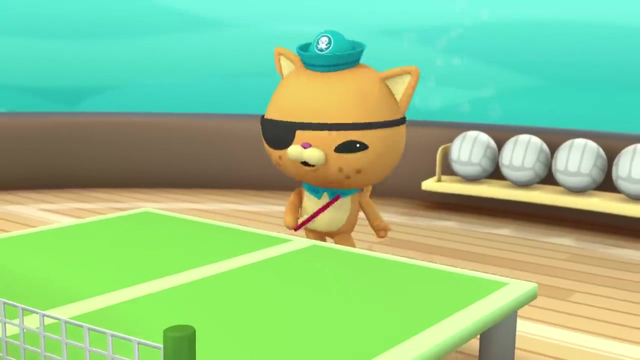 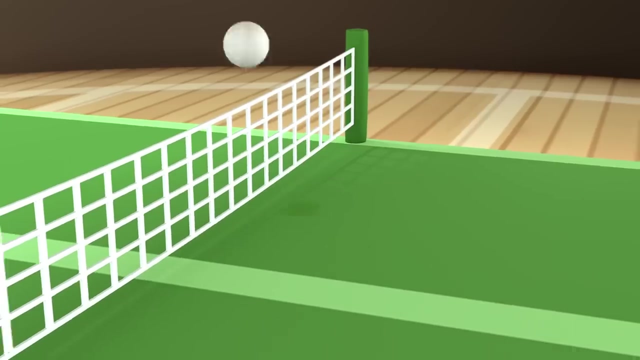 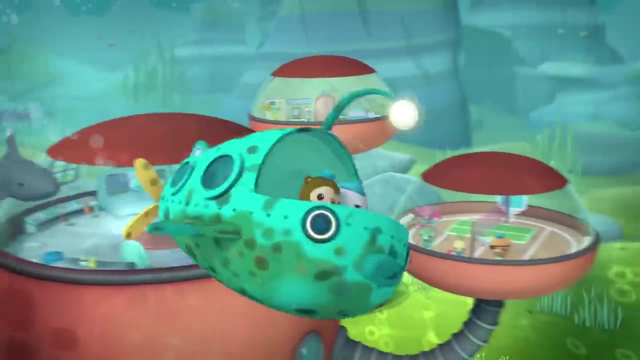 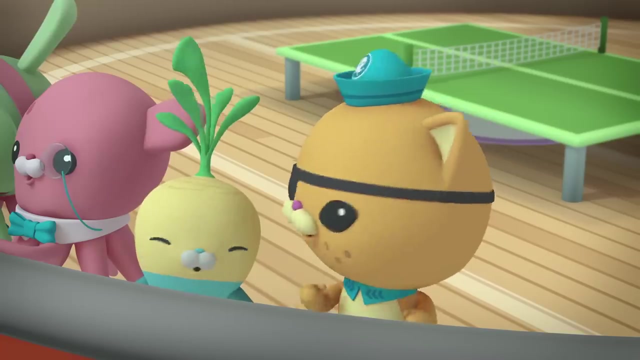 Captain, what's going on? 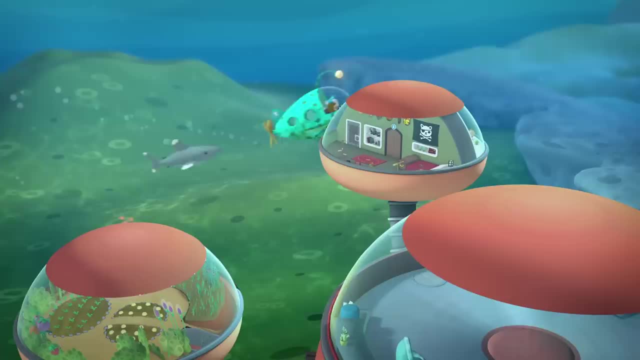 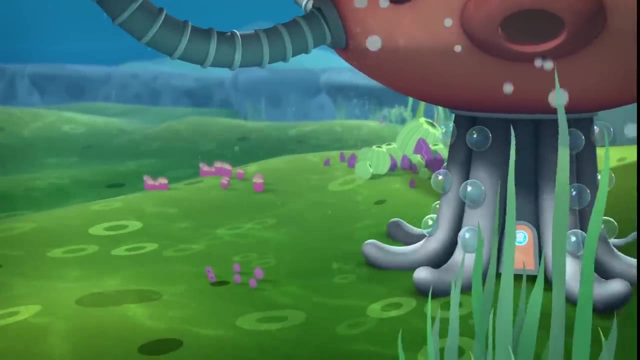 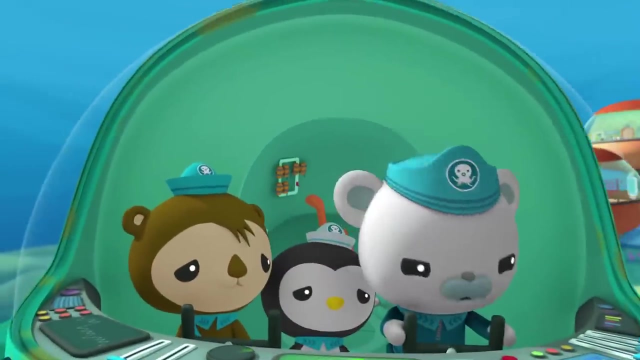 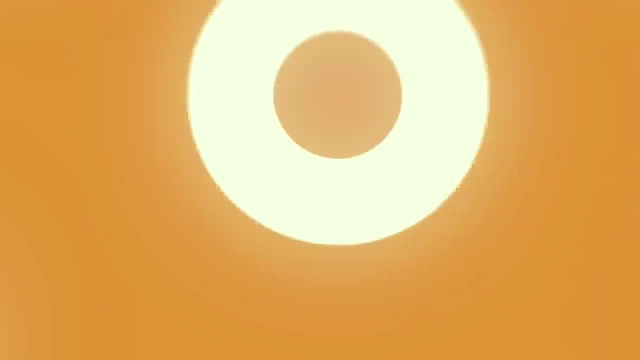 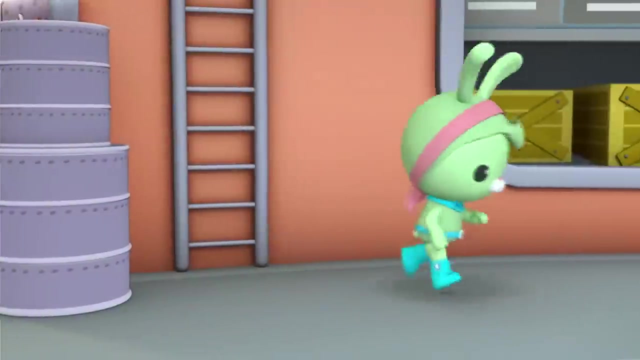 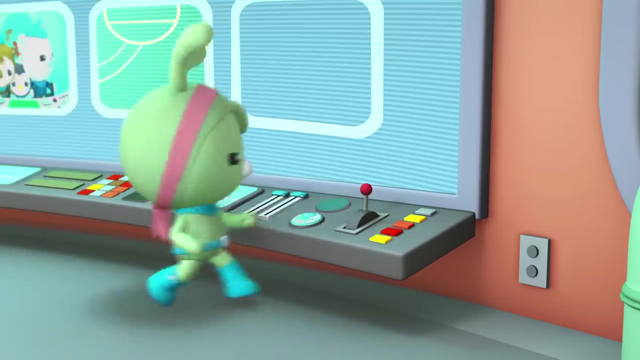 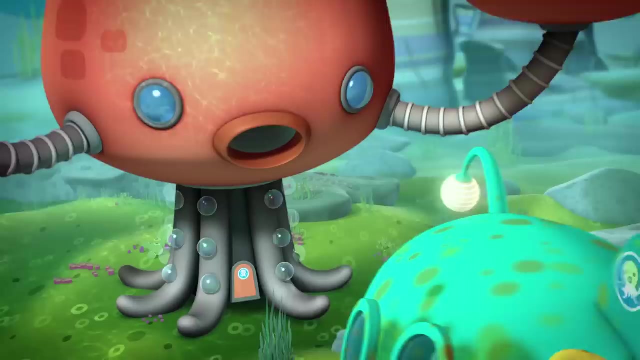 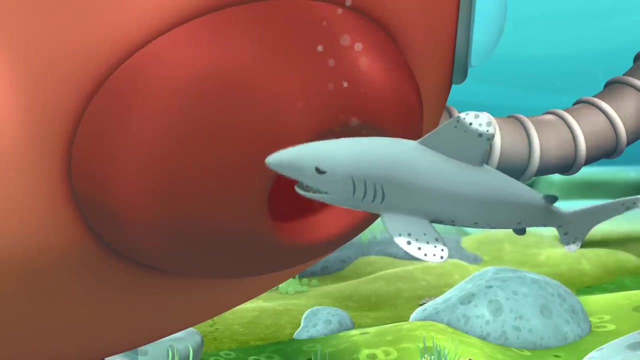 Octonauts, we need to get away from this shark. Open the octohatch Tweak. You got it, Cap. Hold on everyone Ready. Tweak, Now close it. Phew, Good work, Octonauts. 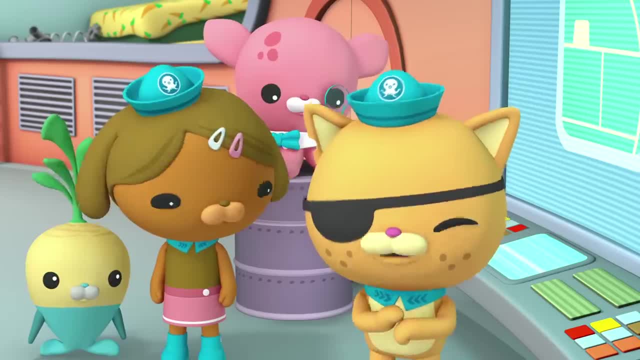 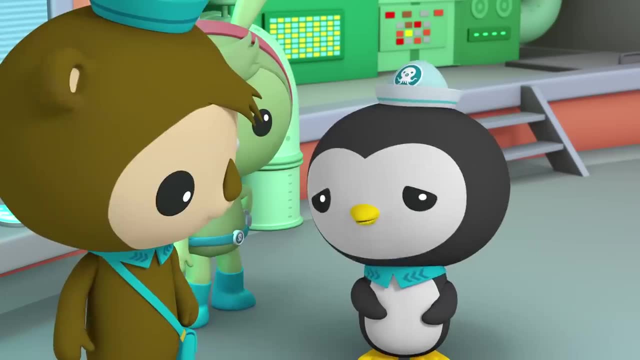 Fascinating. I wonder why that shark decided to chase us. Maybe you looked like a tasty dinner me hearties. No, that can't be it. Sharks don't eat ships. I'm just glad that shark didn't catch us. That'll teach me to take out a gunky gup. 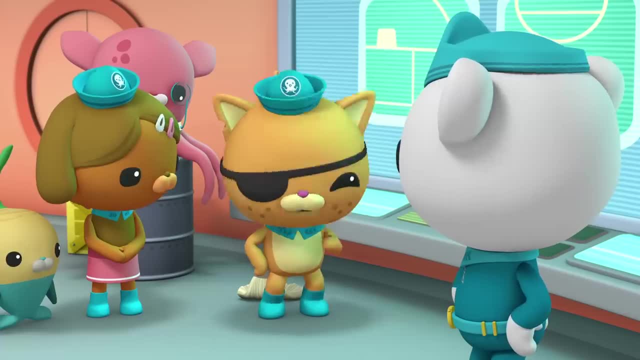 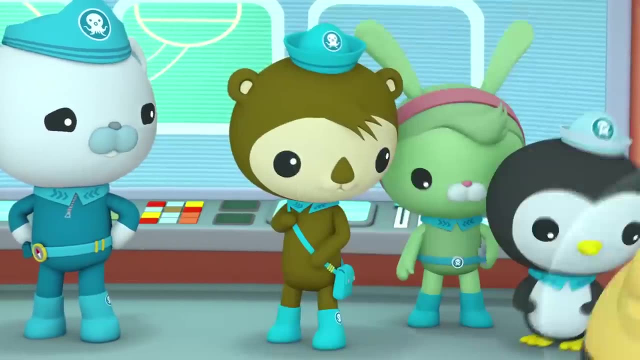 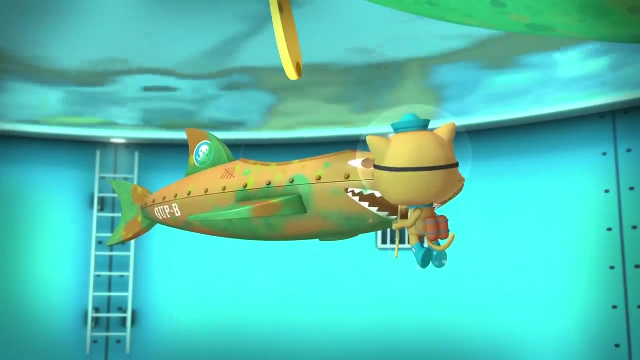 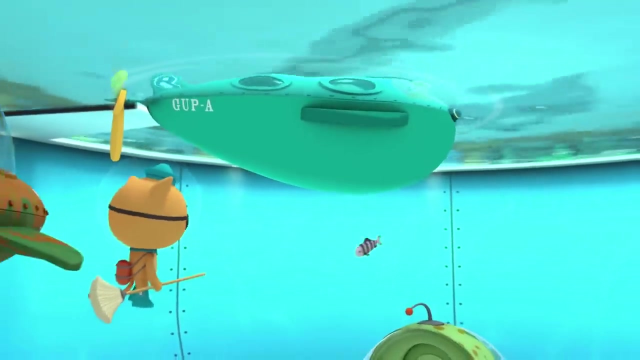 Um, how's the gup cleaning coming along, Quasi, I haven't start- finished yet, Captain. Well, back to work. What? Who cleaned the gup? eh, I did. Hello, How did you get in here? 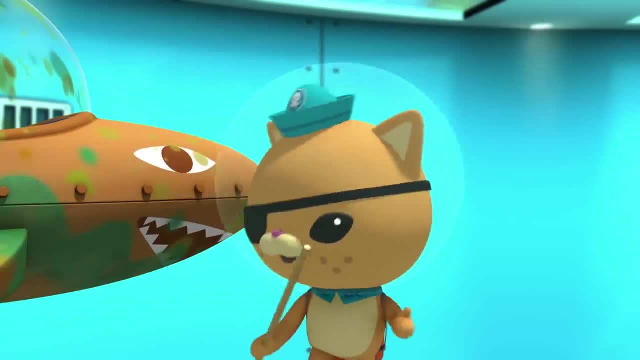 I followed the gup and I'm ready for more, more, more. You mean? you like cleaning, Like it, I live for it. I'm a pilot fish. It's how I get food. I eat the gunk off of things. 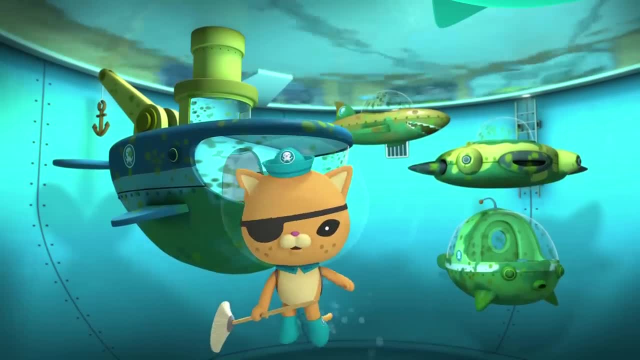 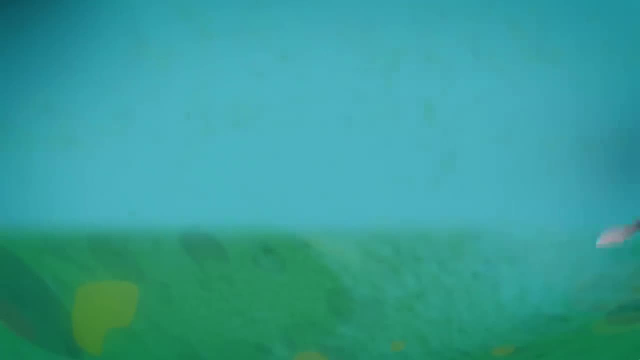 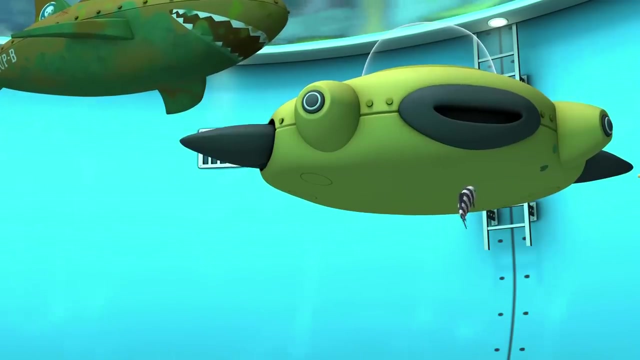 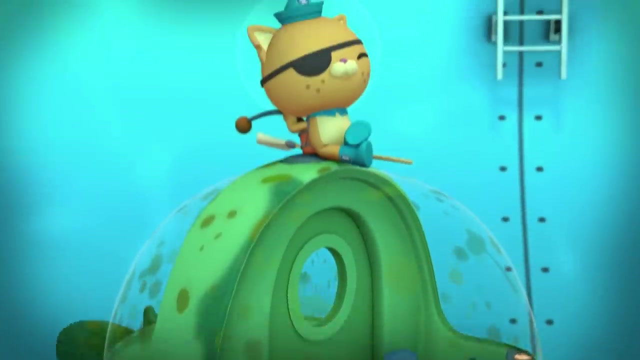 Eat and clean, Clean and eat. Then dinner is served. Oh yeah, look at that, That's filthy Delicious. Oh, look at that Filthy. Bravo, Mortimer, We need an actor of your talent for a special mission. 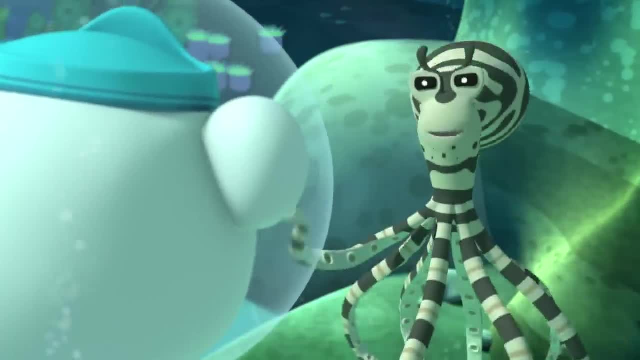 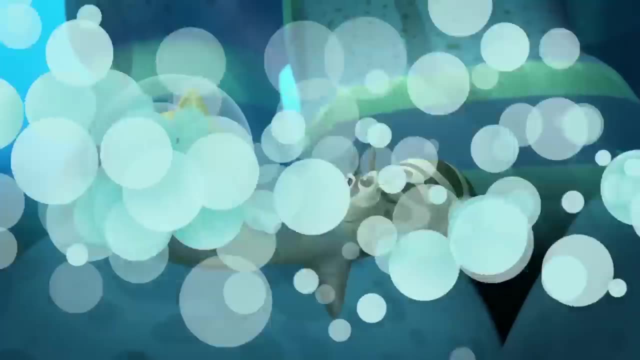 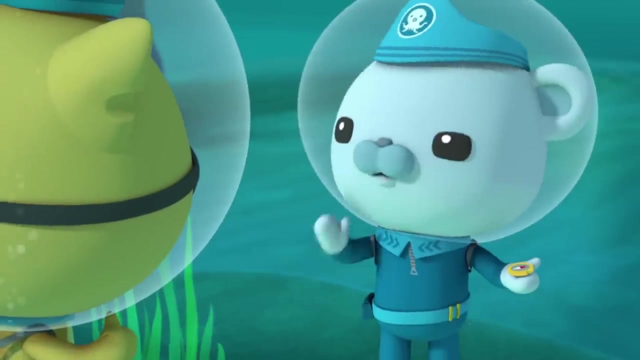 Do you think you could help us Lead on my seafaring friend, My audience Away Show-off. I heard that There he is. All right, everyone. Here's the plan. Step one, Quasi, on my signal, you'll lure the eel out of his lair and lead him into this rocky reef. 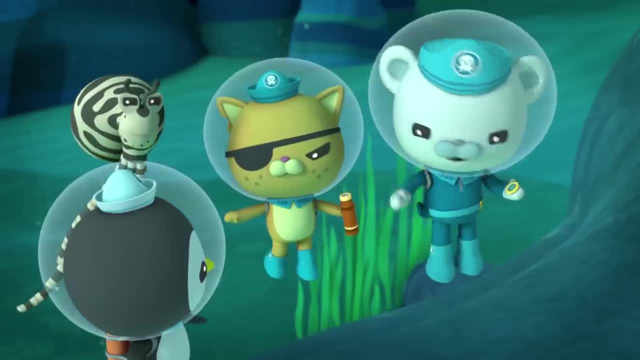 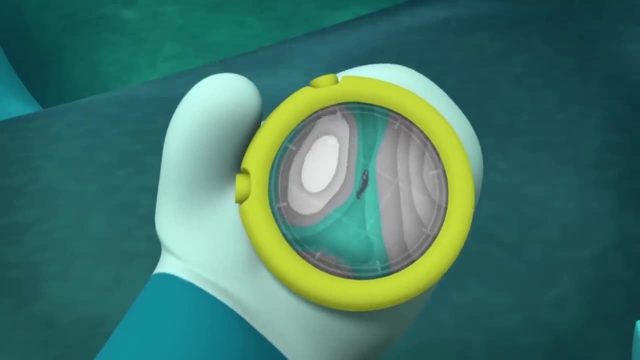 Aye, aye, Captain. Step two, Peso you swim inside to look for the bottle Right-o. Step three: To keep the eel from coming back too soon. Mortimer will create a distraction here. It shall be among my greatest performances. 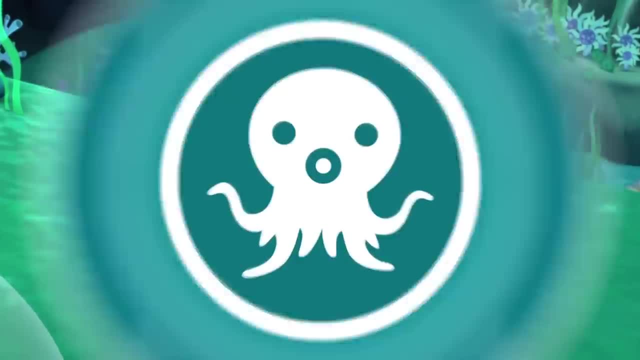 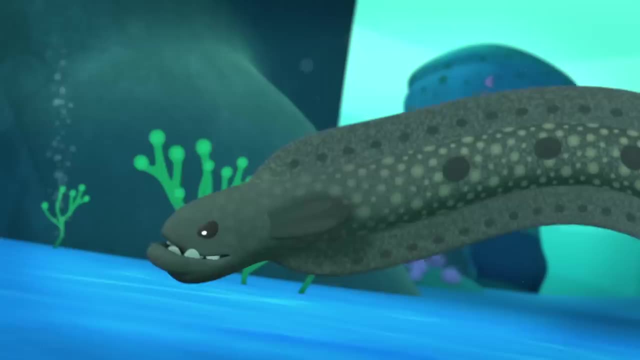 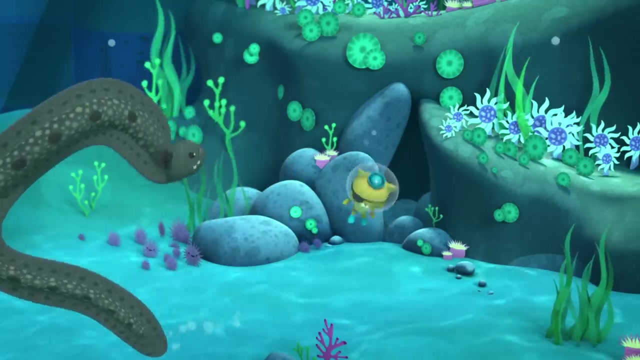 Octonauts and Mortimer. let's do this. Step one, Quasi, go, Stay away from my home. Come and get me you toothy lump. I knew you were asking for it, Arrgh Peso. time for step two. 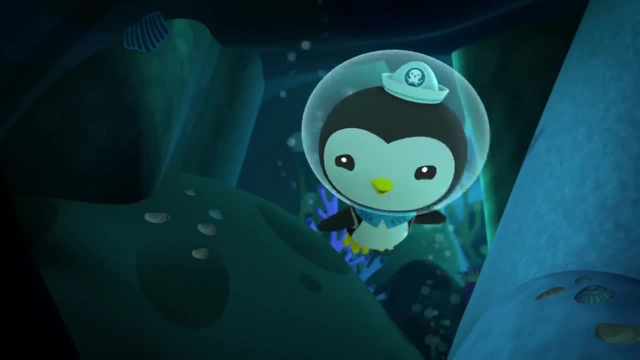 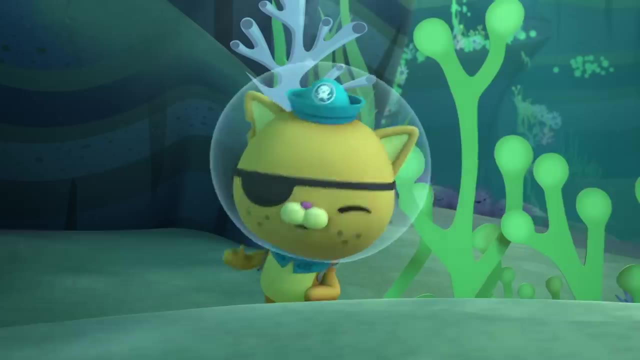 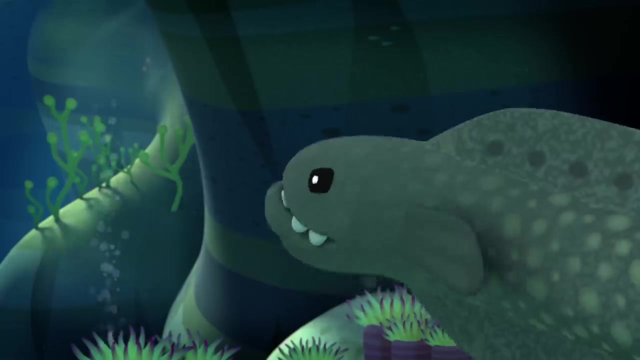 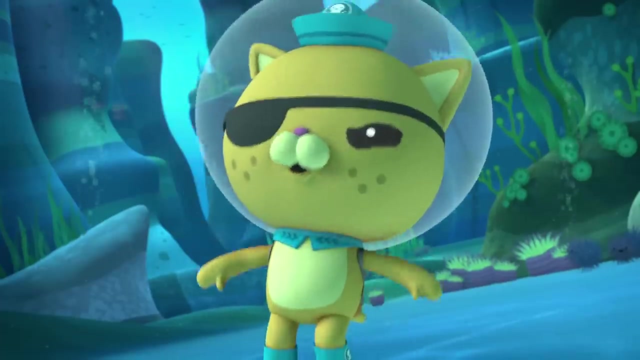 I'm entering the lair. Captain, The algae has to be around here somewhere. Ha-ha, You'll have to be faster than that, matey. Arrgh, Arrgh, Lionfish, Yow Arrgh, Heh-heh. 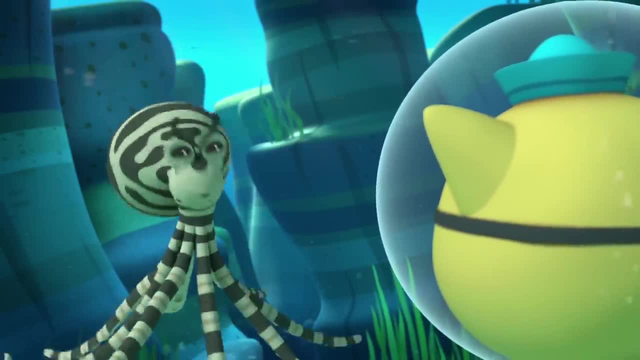 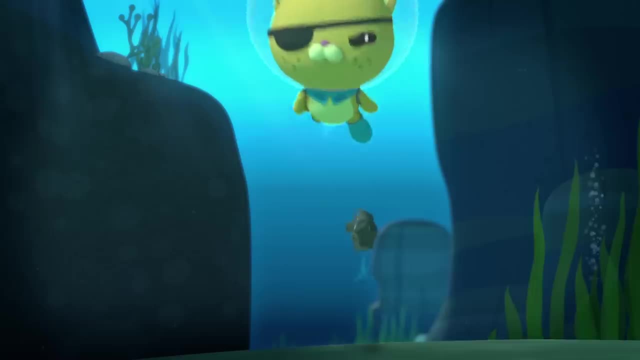 Huh, Admit it, My lionfish impersonation Had you fooled? Well, I suppose, But only for a second. Arrgh, Arrgh. I don't know how much longer I can keep this up, Quasi, in here. 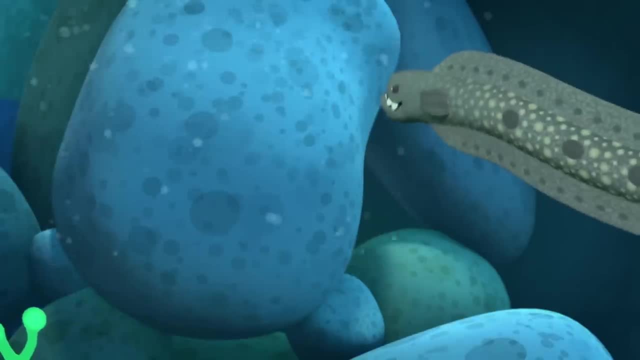 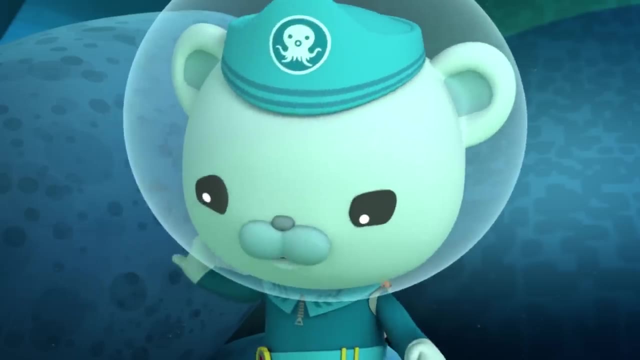 Arrgh, Arrgh, Ha-ha, And you'll stay in there if you know it's good for you. He's heading back to his home, Quasi, are you okay in there? Yes, Captain, Carry on with the plan. 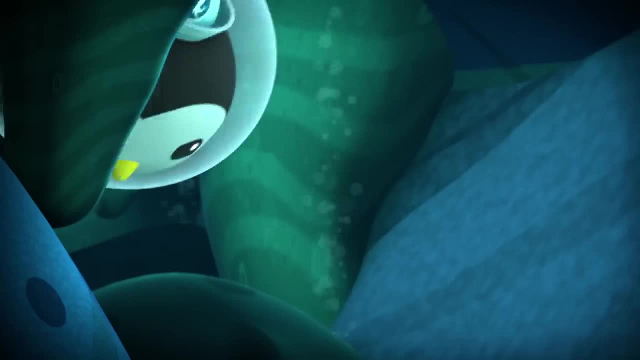 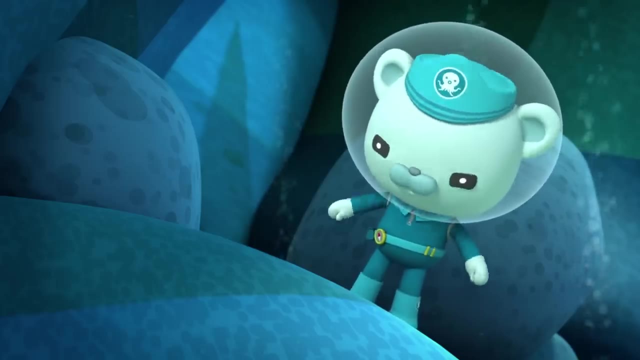 Come in Peso. Any luck finding the red algae? Not yet, Captain, It's a bit of a tight squeeze in here. We'll buy you some more time On to step three. Here he comes, Ready Mortimer. 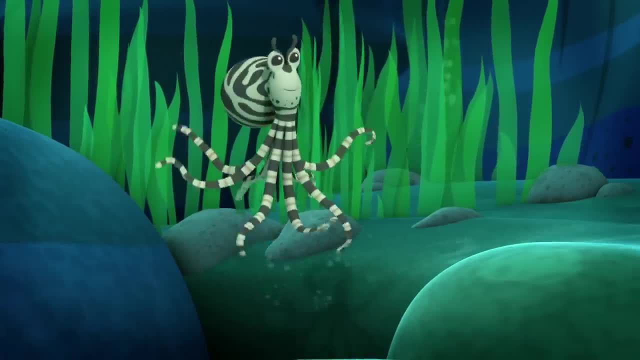 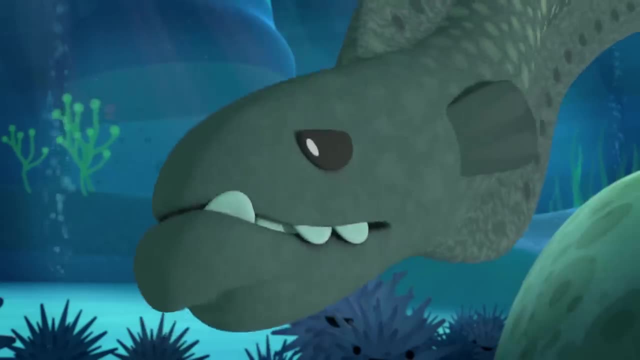 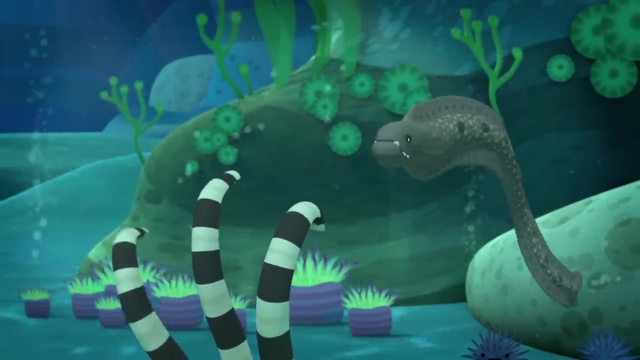 Ready for the performance of a lifetime, dear boy. Ah, No, Not sea snakes. Yes, We are one, two, three sea snakes Begone. Oh, We'll fight you inside out. Hiss, Hiss, Hiss. 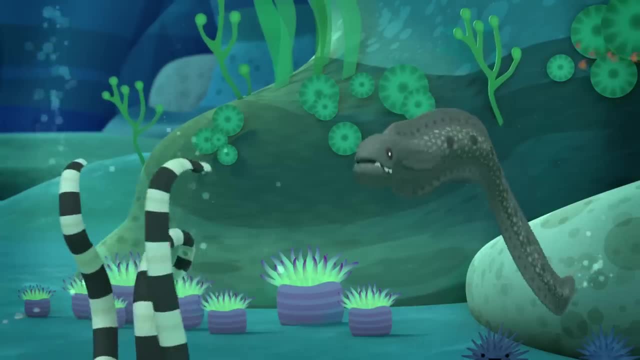 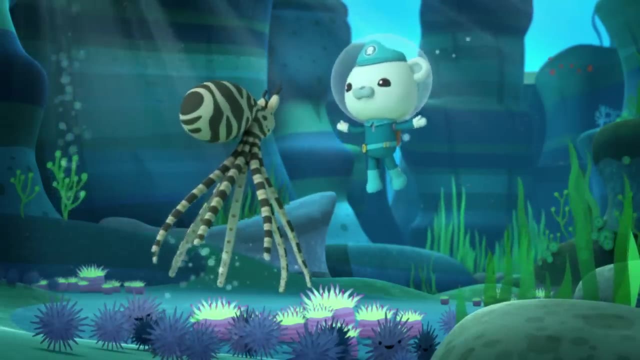 Hiss, Hiss, Hiss. Don't overdo it. Aye-ya, I think I'll take another way home. Excellent Mortimer, Another five-star performance. Thank you Well, Peso. any luck, Captain. I think I see the bottle. 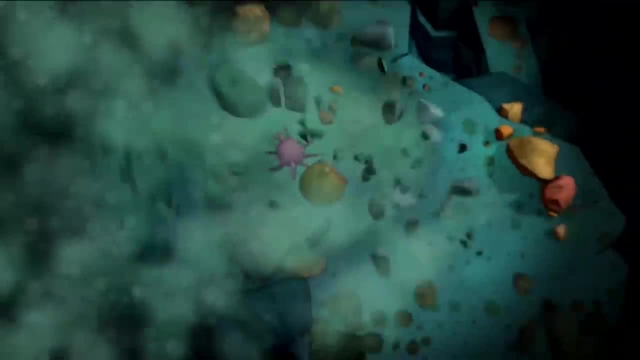 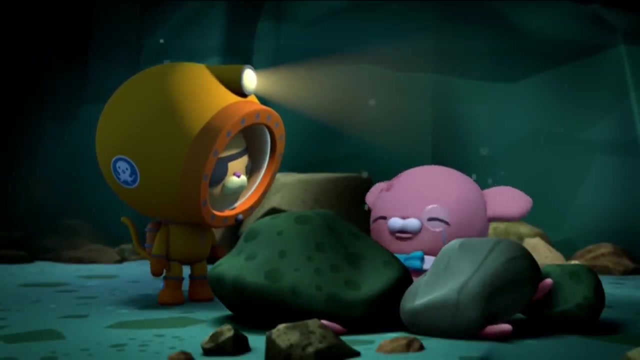 Arrgh, Arrgh, Arrgh, Arrgh, Arrgh. Uh, I think um, I think um. I may need a little help getting my tentacles untangled. I'll get you out. Professor, Those rocks are no match for me. 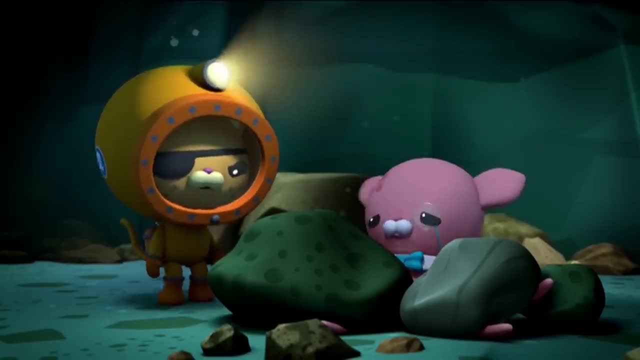 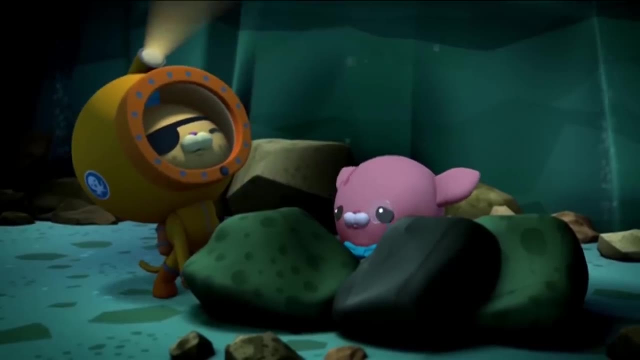 I've almost got it. It's not safe down here. Quasi, Get out while you still can. A pirate never leaves his crew behind Ow Or his tail. Arrgh, Arrgh, Arrgh, Arrgh, Arrgh. 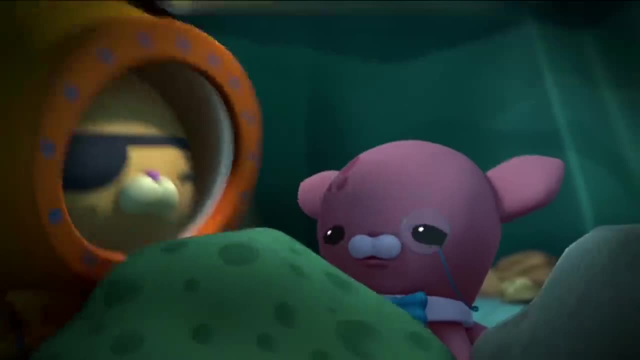 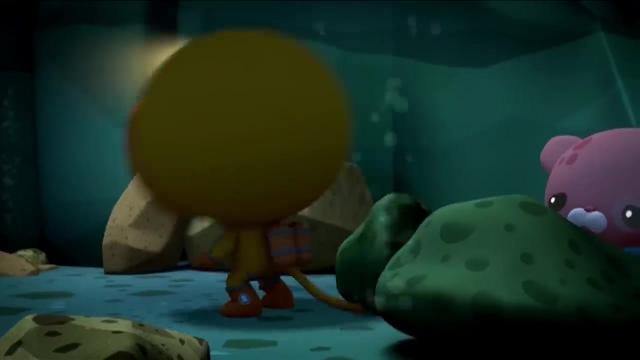 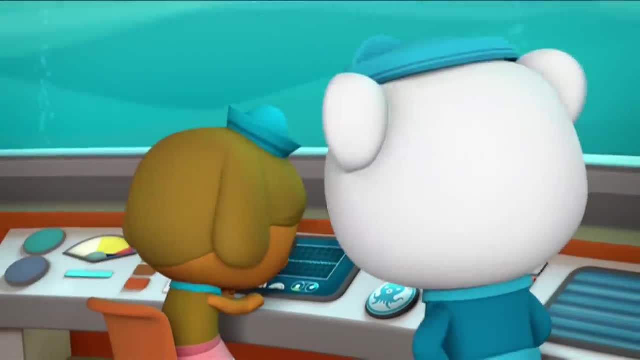 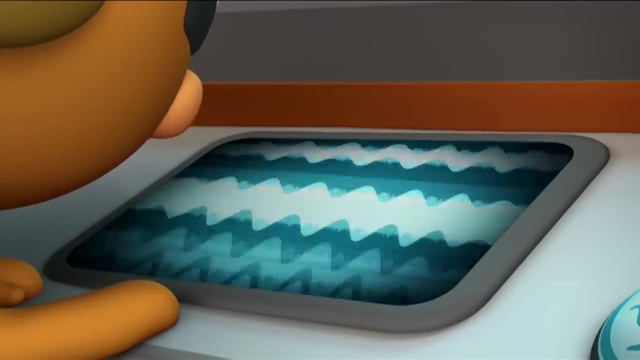 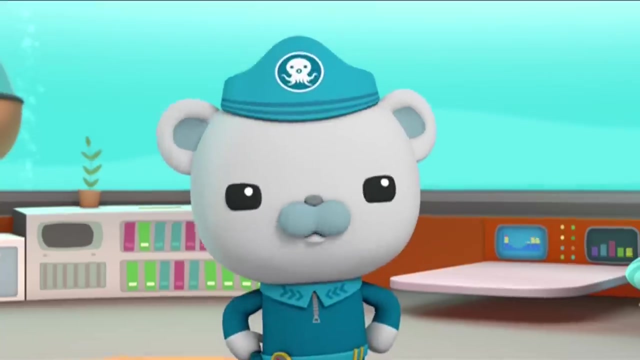 Captain, I'm picking up some big tremors coming from the Midnight Zone. The sea floor's breaking up. Come on, Captain Tanks, Giant bombers. We've lost contact. Captain Dashie, sound the octo-alert Octonauts to the launch bay. 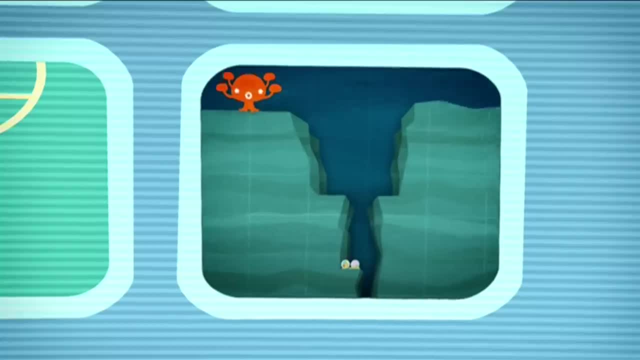 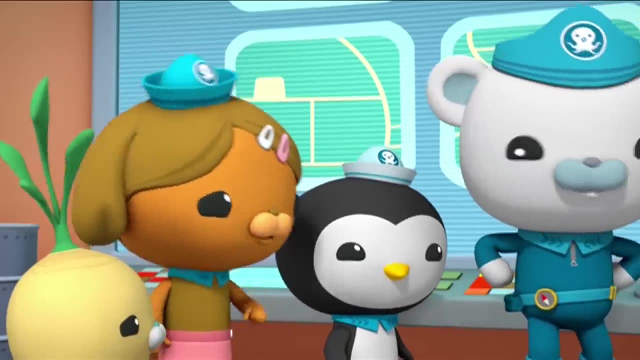 Octonauts Professor Inkling and Quasi are trapped in the Midnight Zone. They're wedged in under some boulders. We have to get them out right away. Tight space heavy lifting Sounds like a job for The Octomax suit. 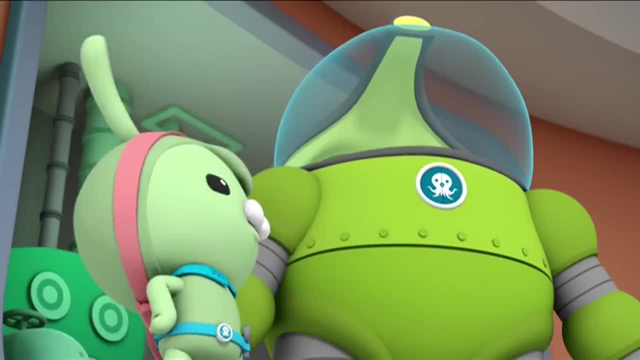 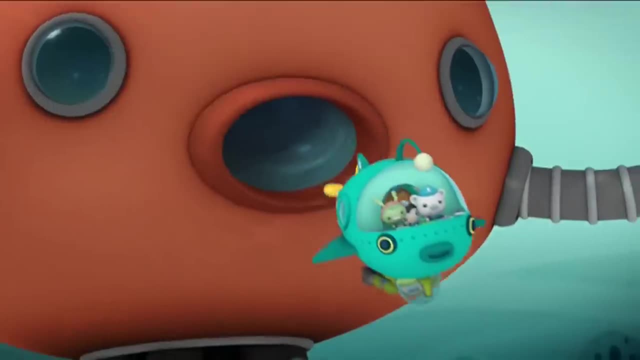 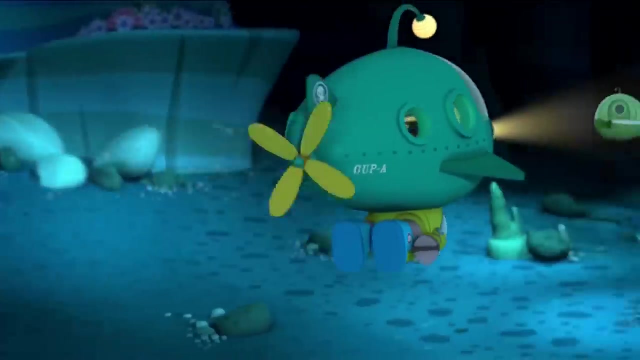 Just what I was thinking. The air tank is only good for a short mission. Then we'll have to work fast. Tweek Dashie Peso, let's go. There's the Gup E Mmm, they must be down there. 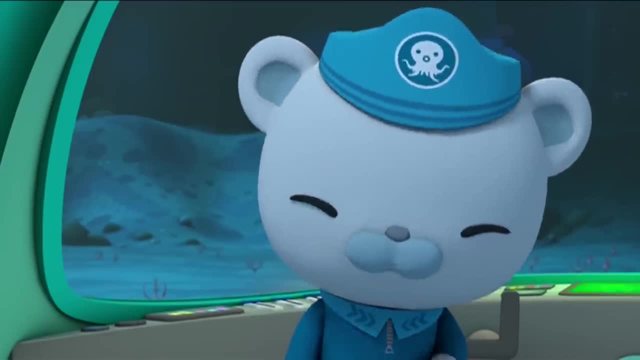 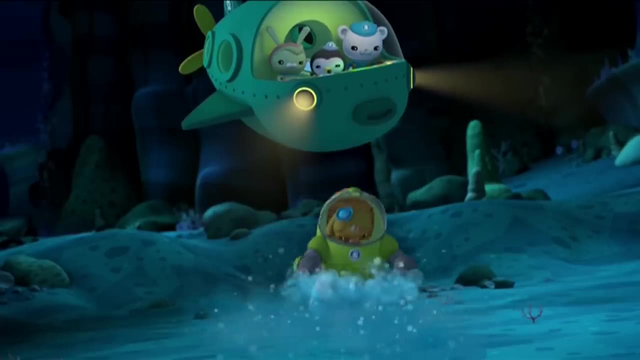 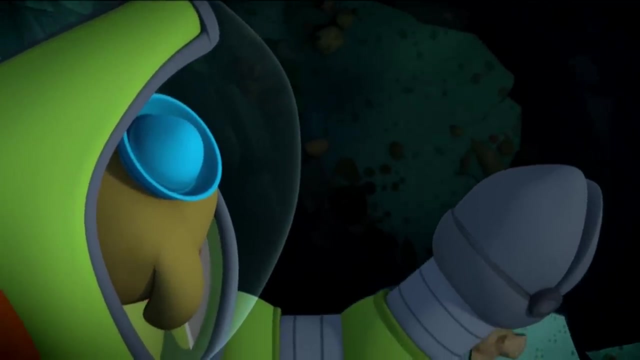 It's up to you now, Dashie. We'll monitor your air tank from here, but you'll have to work fast. I'm on it, Captain. Any sign of Professor Inkling and Quasi? Not yet, Captain, but it's dark down here. 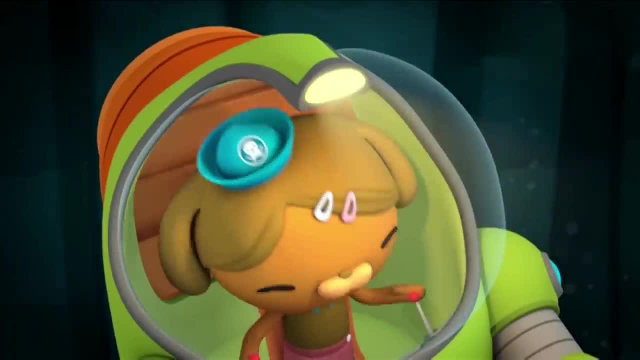 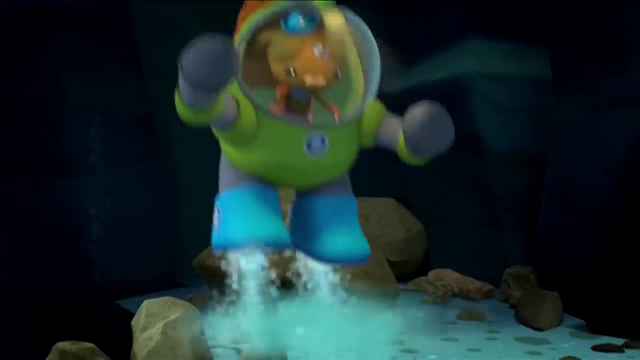 Activating searchlight Bingo. I see them, I'm going in, Captain. We read you. Dashie, Keep us posted. Looks like you two are in a tight spot, Dashie, Don't worry, I'll have you both out of there in no time. 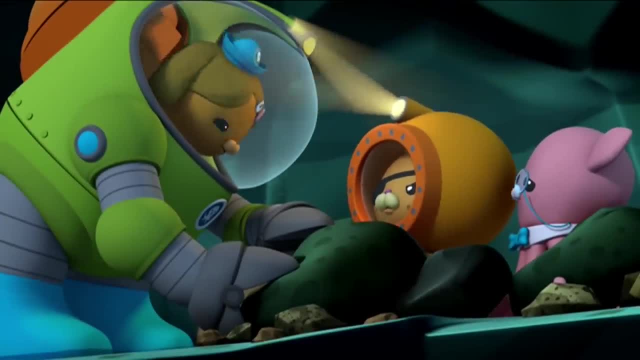 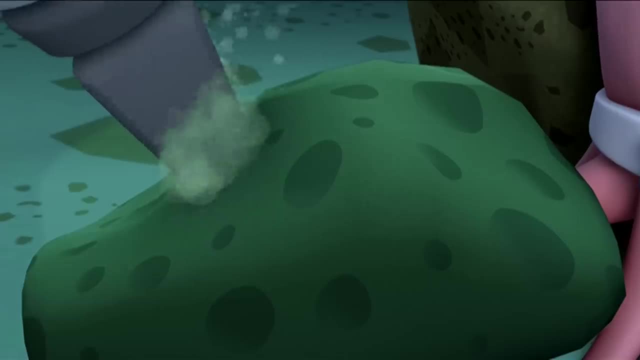 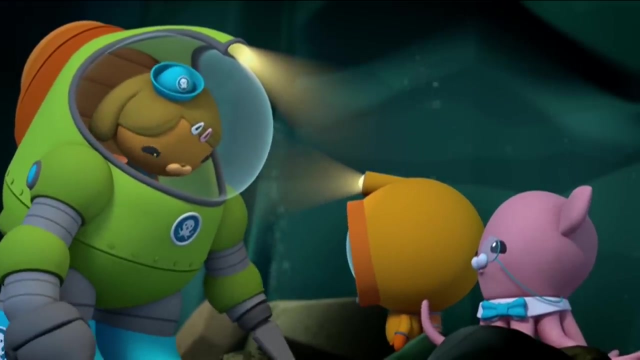 It's too heavy. Now what? Don't worry, Quasi, This suit has a few more tricks up its sleeve: Activating jackhammer. One tentacle free, two to go. Well done, Dashie. Now move the jackhammer to your right and down. 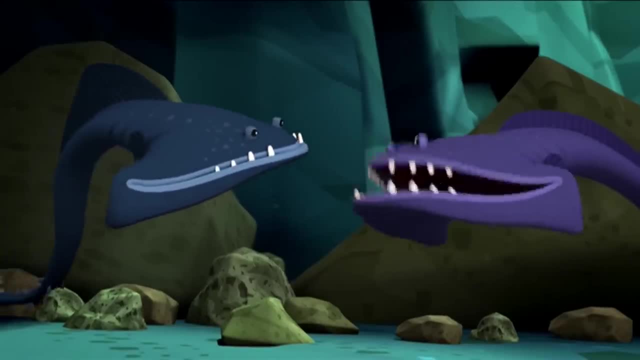 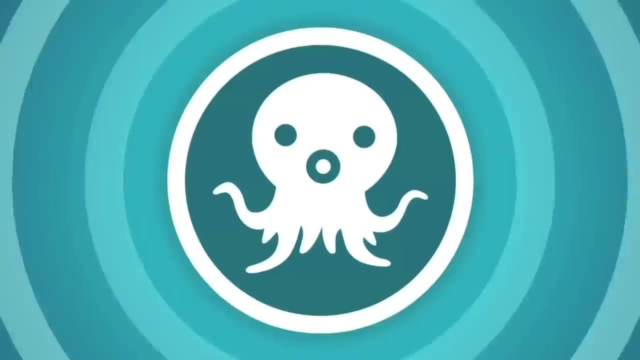 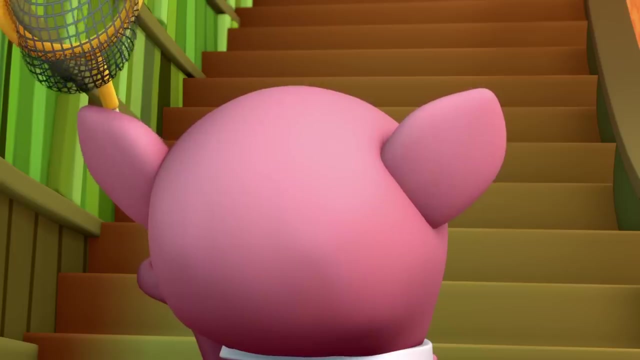 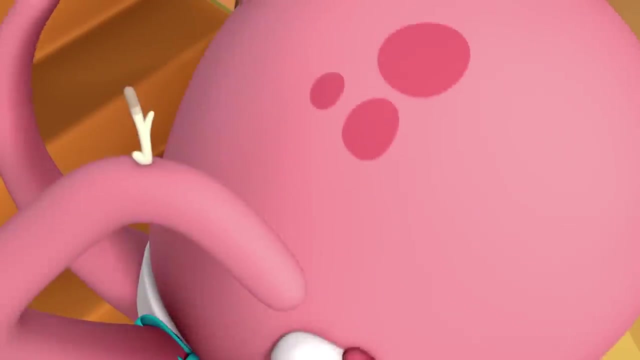 I'm still hungry for octopus. Let's swim back slowly, And then we'll open our jaws and Go Octonauts. let's split up and find that cone snow. Nobody captures me, you see. Leave me alone, will ya? 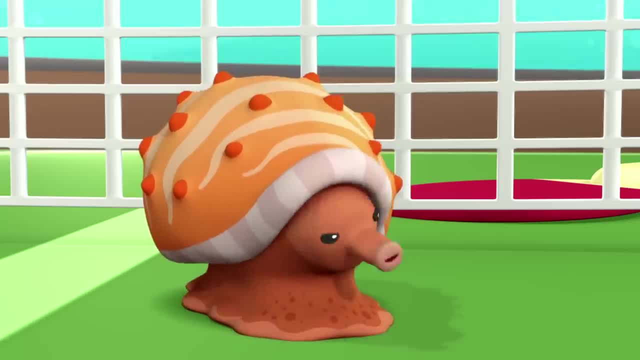 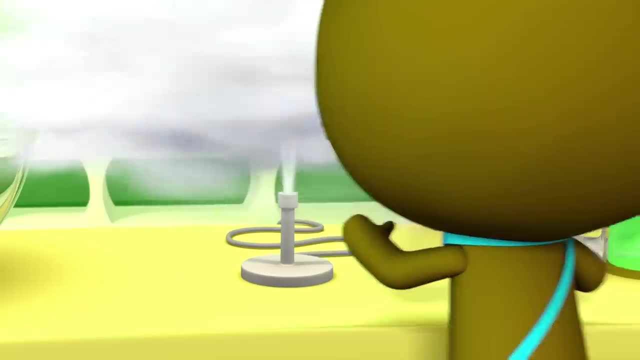 Octonauts. any sign of the cone snail? Not yet Cap Anyone else? Oh no, Inkling Dashie and Shellington have all been stung Peso I'm bringing three more patients to the sickbay. 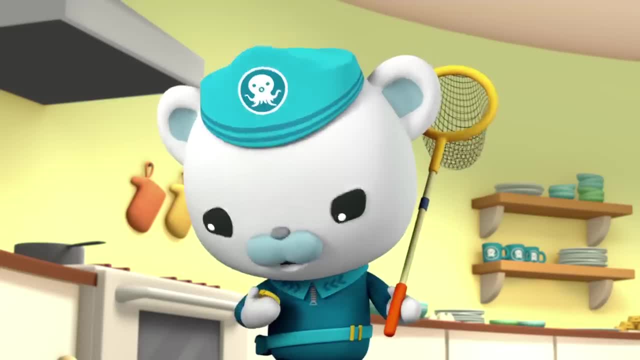 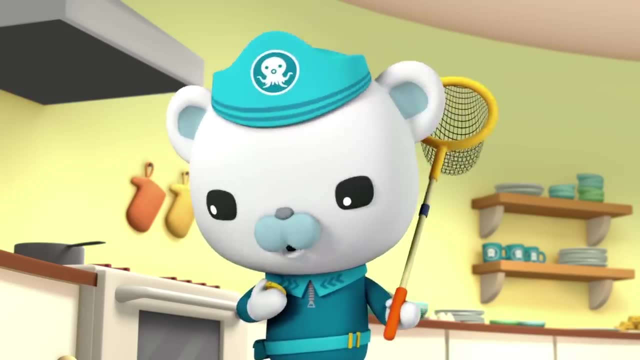 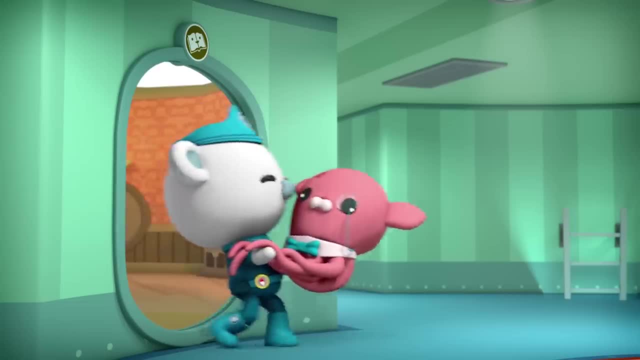 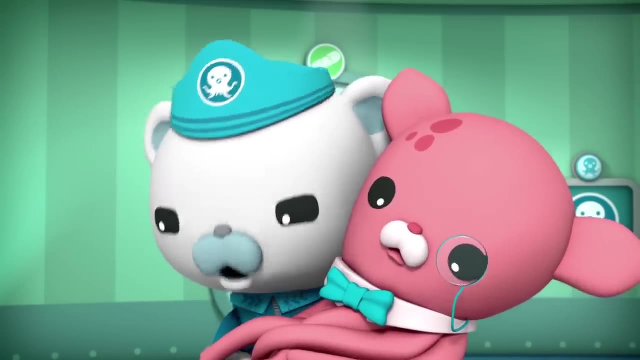 Oh no, Oh no, Shellington, You must know what by eye, Captain Tweek, the cone snail must be somewhere in the octochutes. I need you to close them off. Awesome Cap, I'll let you know as soon as folks say yes. 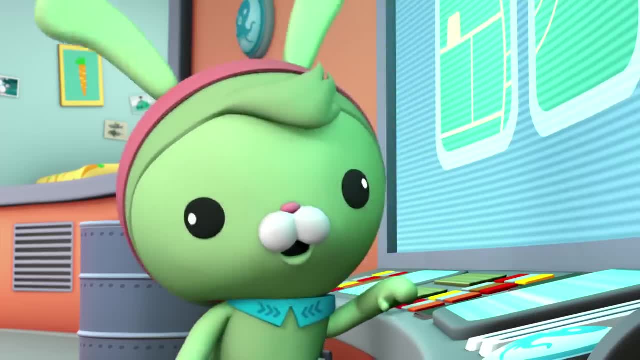 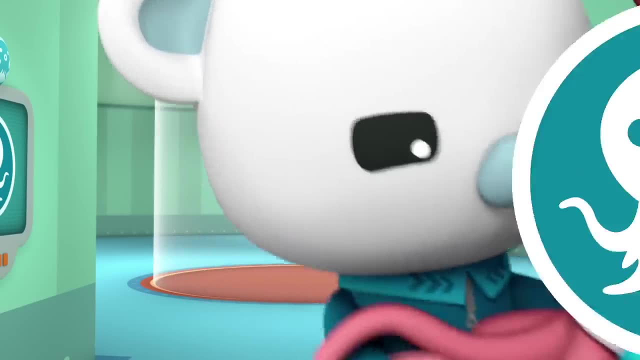 poured in 借 Sweep warmly. Tweek, Are you all right? Yes, I'm fine. There we go. That's better than never. Why See how comes the snow is not spiky. Tweek, The cone snail must be somewhere in the octo shoots. 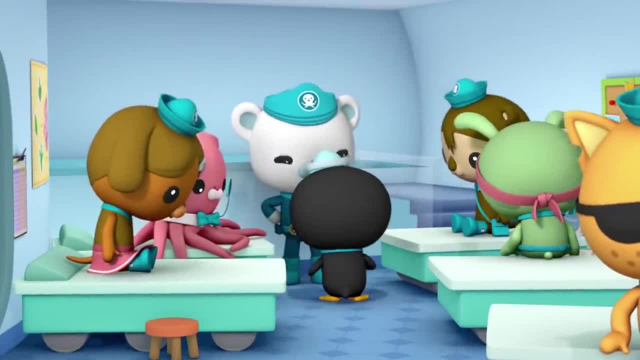 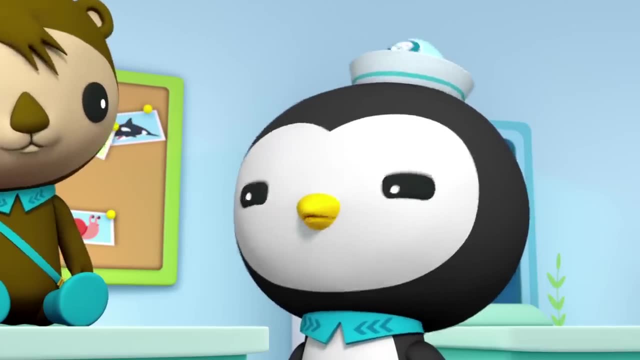 That means you don't know how to make it, Or the octo shoots. How are you doing Peso? This is a lot of patients to take care of at once. Don't worry, Captain, I'm a medic. Taking care of people is what I do. 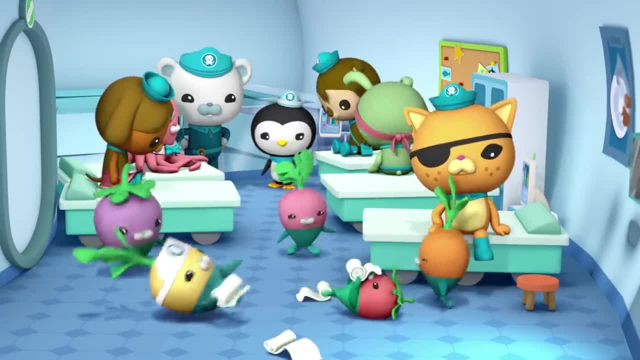 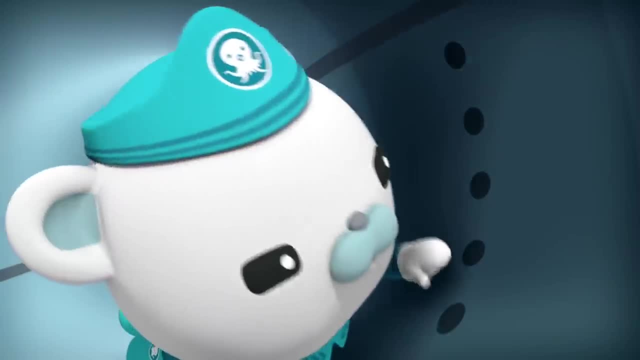 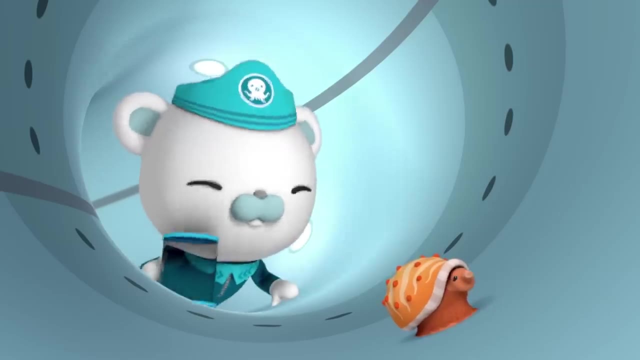 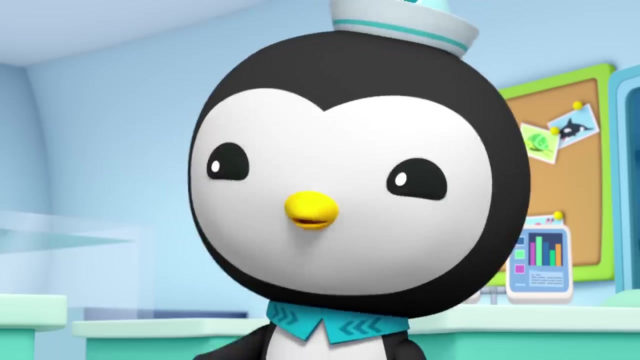 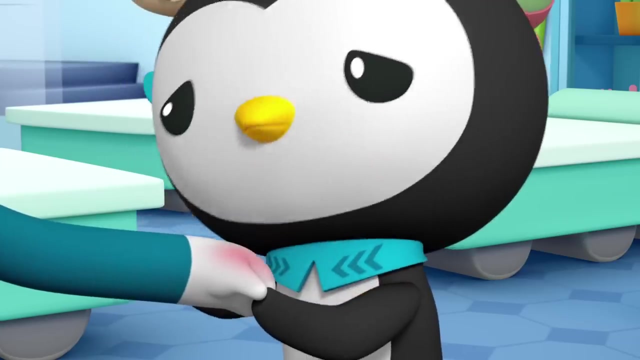 Luckily I have some help. Hmm, He must be in the vents, Right, I'm going after him. Ah-ha, Hey, watch it. What's the big idea, Captain? you did it. Oh no, You were stung. 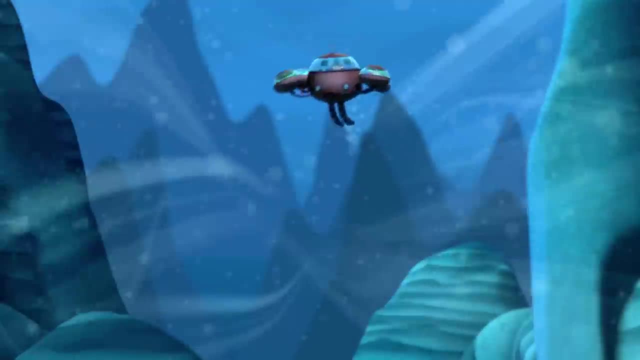 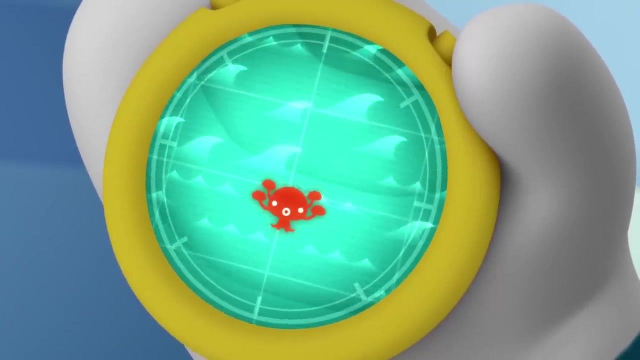 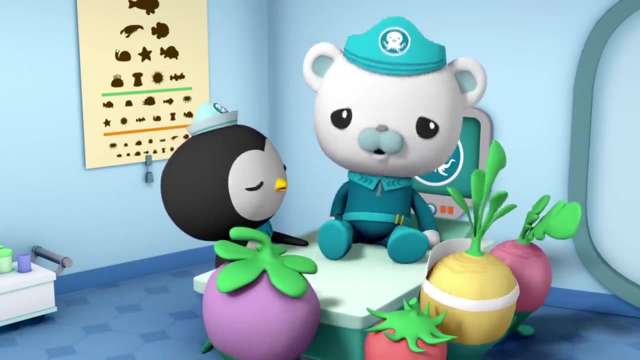 Just rest easy, Captain. Everything will be What's happening? Ship's entering the Roaring Forties- Very rough water Need to Get through. No, Captain, You're too weak. Yes, Somebody has to pilot the ship And that person is you, Peso. 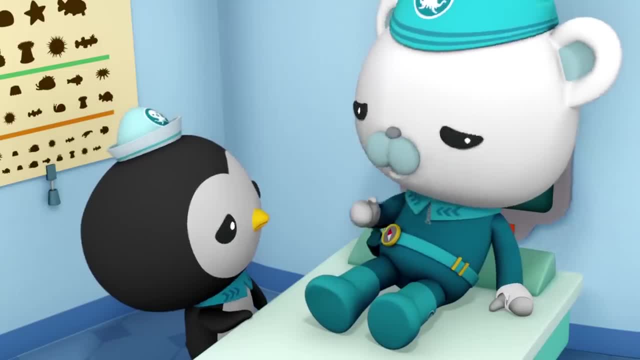 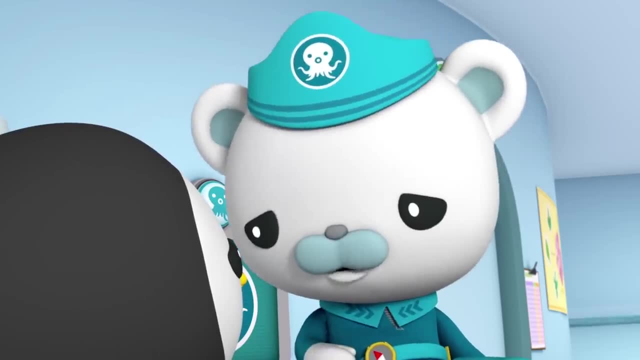 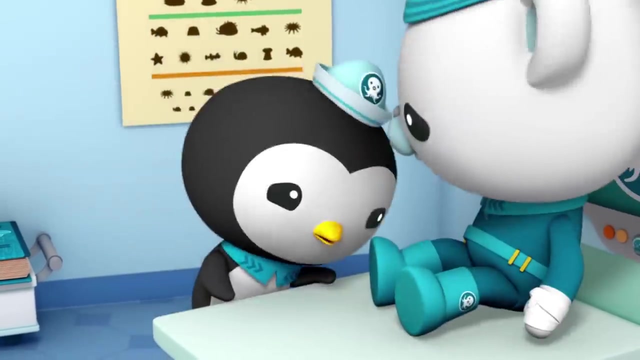 Me Peso, use the manual. You can do this. But, Captain, You've learned 317 ways to bandage an injured fin. You've performed crevictomies in the frozen Arctic. Those are medic, Medic skills And I've done those things lots of times. 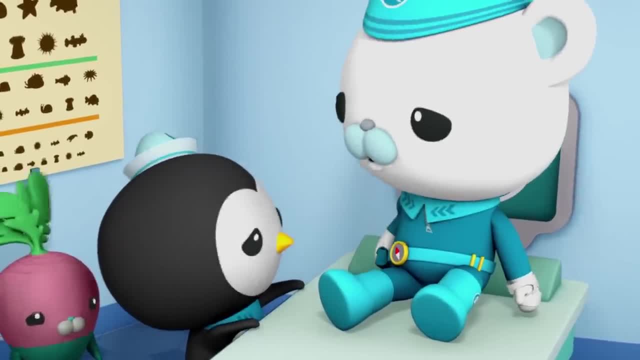 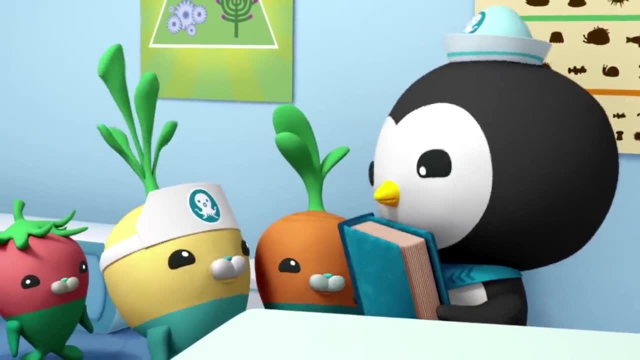 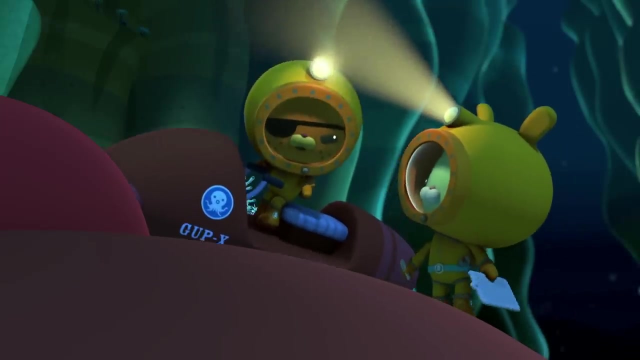 But there was a first time. We're all counting on you. I, I, I have to try, Tunip, keep an eye on my patience. What's the matter, matey? You look like you've just seen a sea ghost. 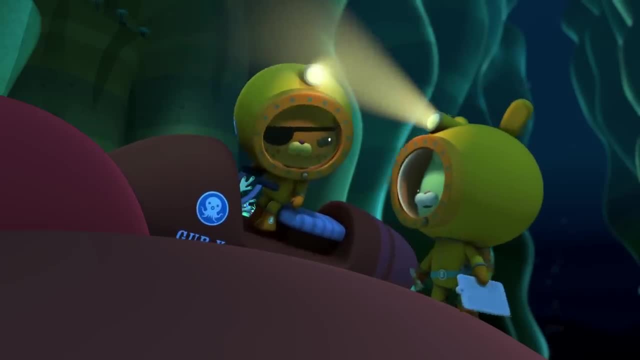 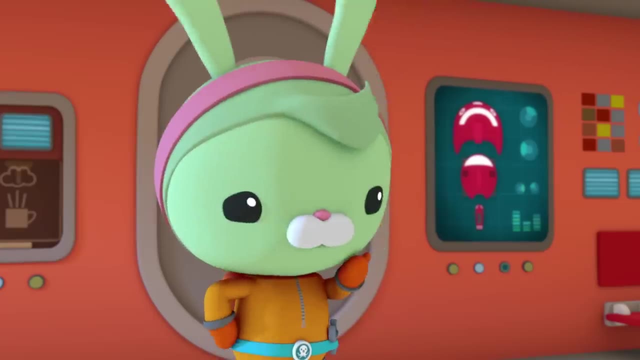 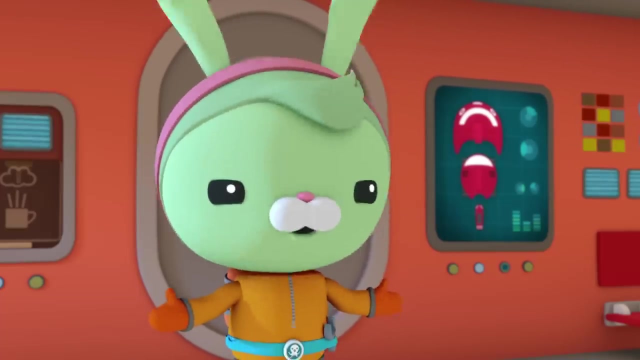 Whew, Must be my imagination. Come on, Quasi, We'd better get back inside. Come on, Tweak. What was out there? Well, I know it sounds crazy, but I could've sworn. I saw something white and furry climbing around on the guff. 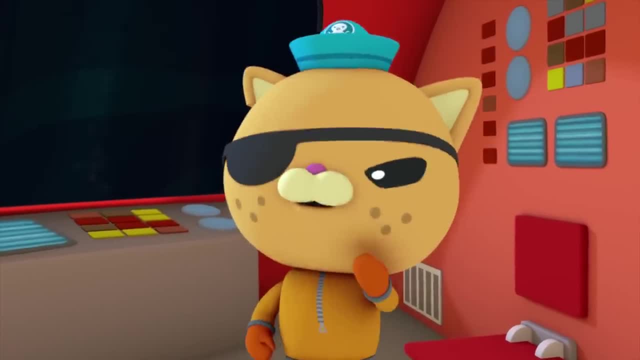 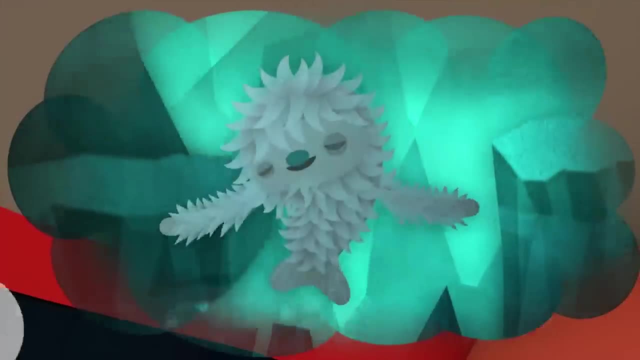 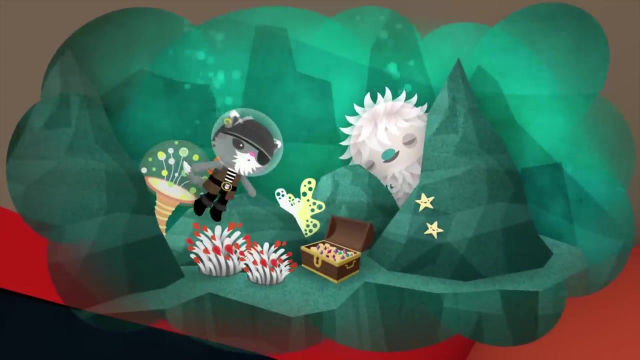 White Furry. Oh mateys, There's only one thing: it could be: A sea yeti. Half fish, half shaggy white beast. The sea yeti lurks in the darkest depths of the Midnight Zone, But you'll always smell it before you see it. 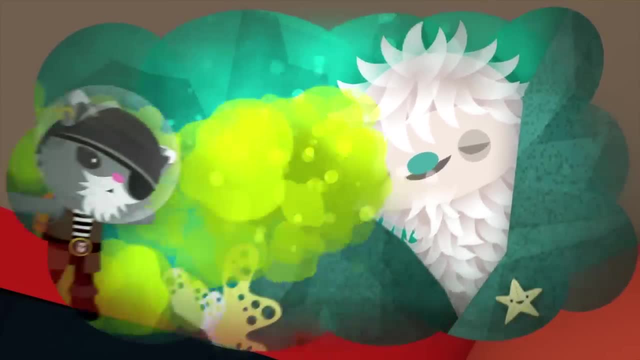 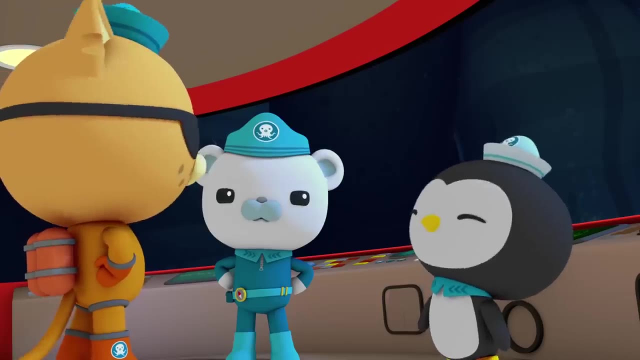 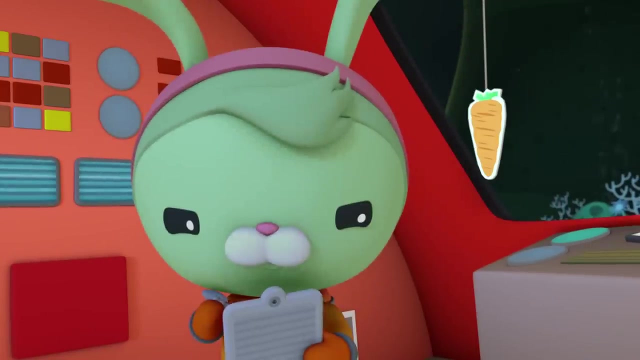 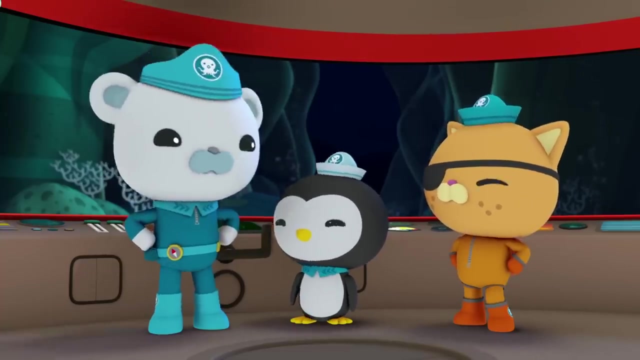 A sea yeti's foul breath smells like rotten eggs and is strong enough to knock out the mightiest pirate. Now that you mention it, it does smell sort of funny in here. Hmm, Note to self: Replace the air freshener. Well, sea yeti or no sea yeti. we'd better finish the inspection. 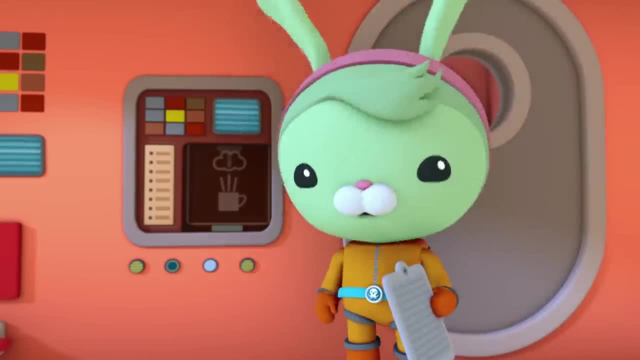 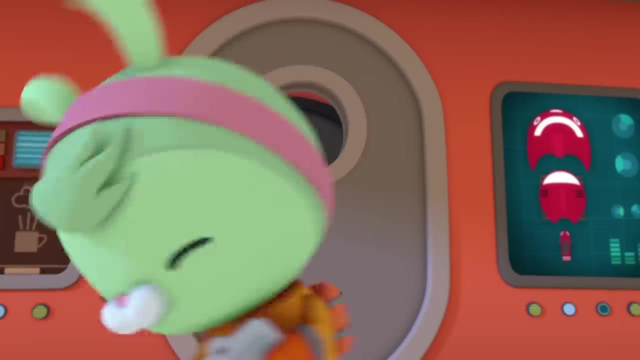 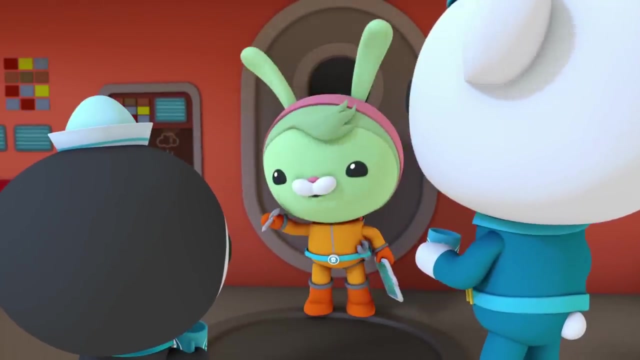 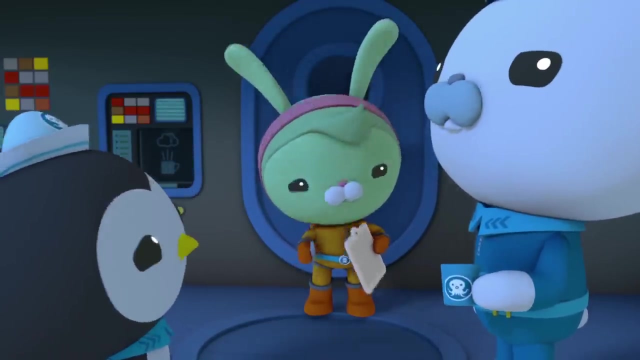 There's just one more thing on my checklist: Cap, The hot cocoa machine. Oh Well, Oh, check, That does it. The Gup-X is in total and complete, 100% work in order. Huh, Hmm, Sounds like we have a stowaway. 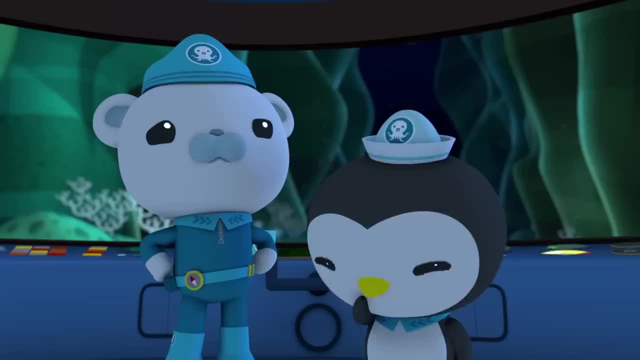 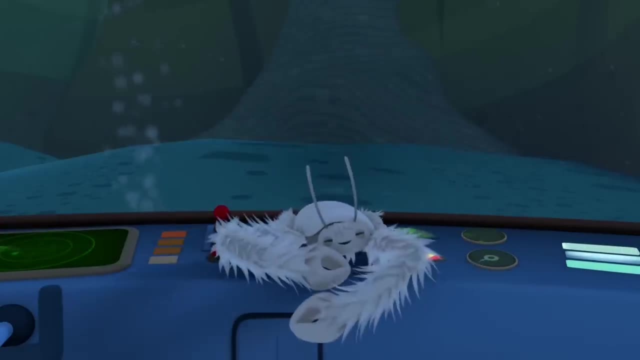 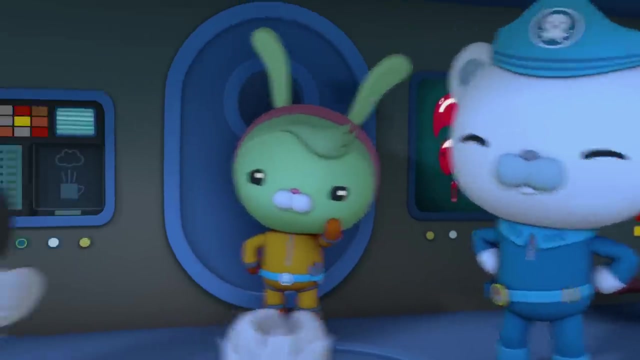 Smells like it too. Yow, The sea yeti's got me. Oh, I am not a sea yeti, I am a yeti crab And my name is Klaus, A yeti crab. Whatever you are, matey, You don't smell too good. 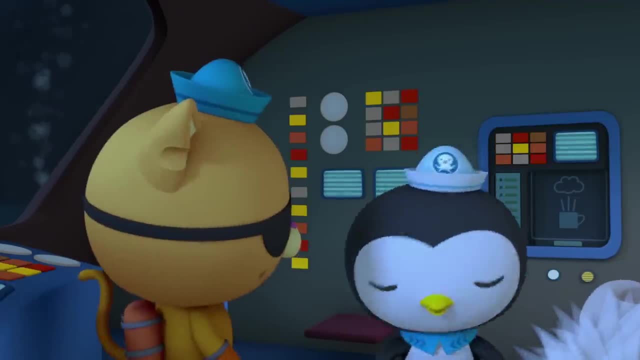 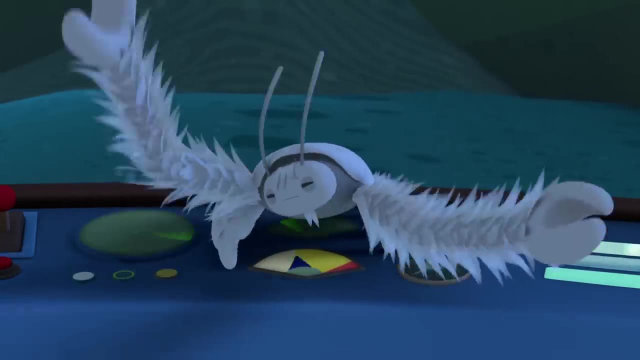 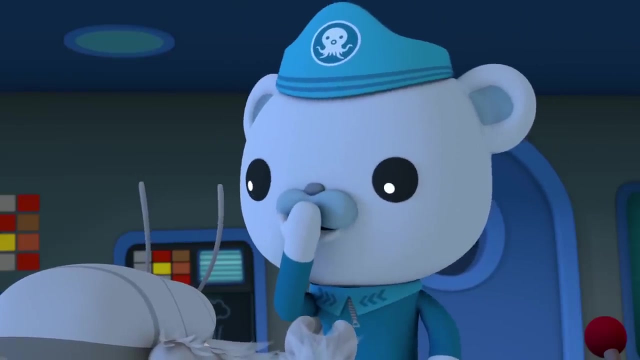 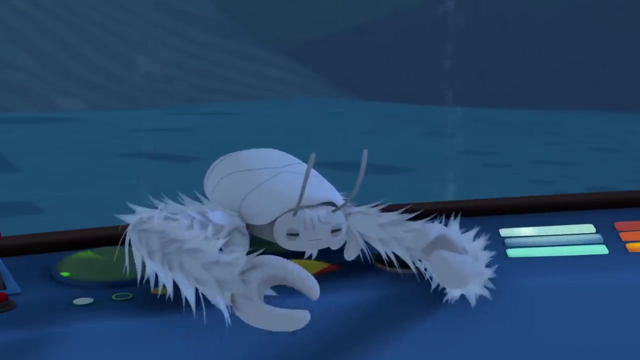 Sort of like rotten eggs. Huh Yeah, That is a smell from the hydrothermal vents where I live. Oh, smells delicious. Phew, You live near the hydrothermal vents, Aren't they very hot and dangerous? Not for a yeti crab. I use the hairs on my arms to catch tiny bits of food coming out of the vents. 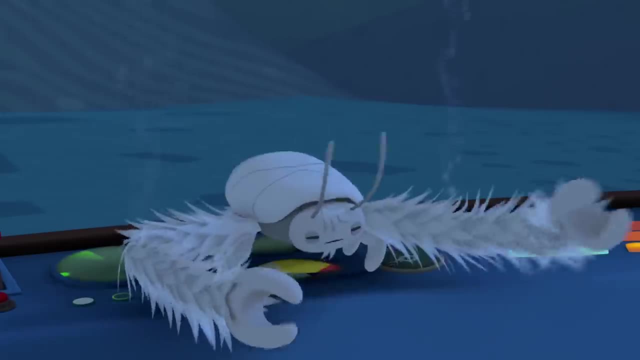 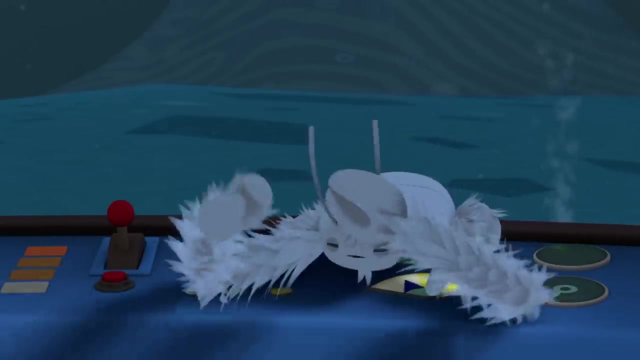 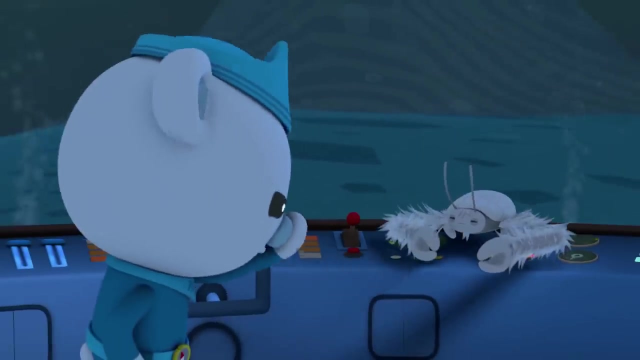 But there is nothing to eat inside this rock, and I am also hungry. This isn't a rock, It's our ship, Your ship? Oh, pardon me, We yeti crabs are blind. I cannot see a thing. In that case, Klaus, you'd better let us take you back home. 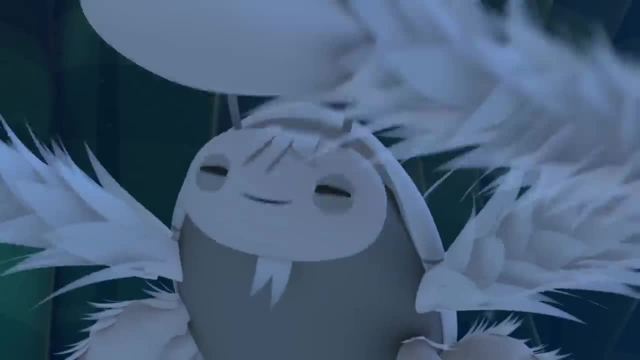 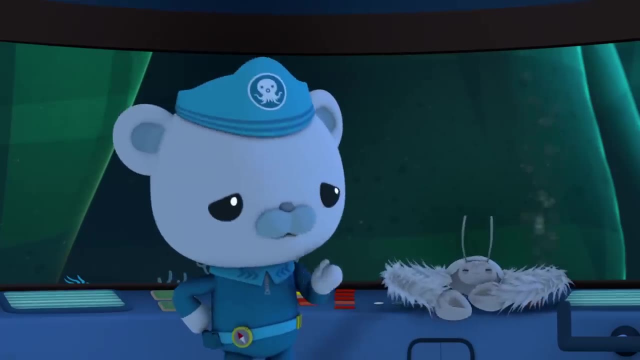 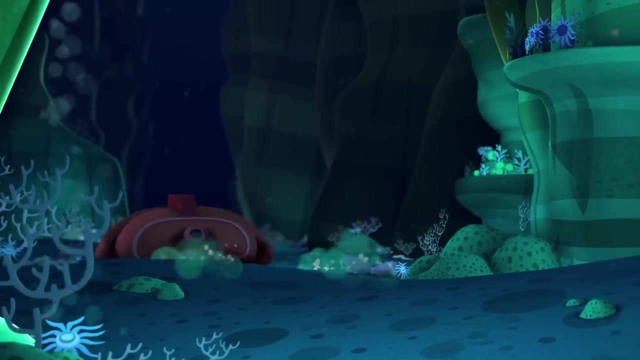 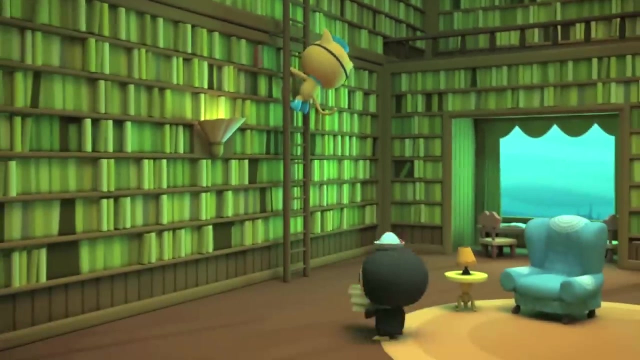 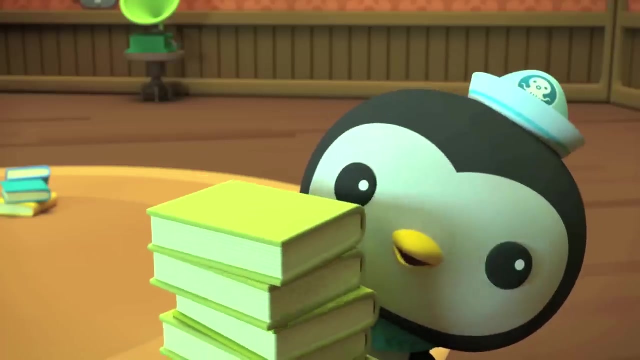 Oh, thank you. That would be wunderbar. It is almost my dinner time. All right Octonauts. Back to the hydrothermal vents. Mysterious island monsters, Castaway creatures, Exotic beasts of land and sea, Kwasi, it's been hours and we still haven't found anything about tree lobsters. 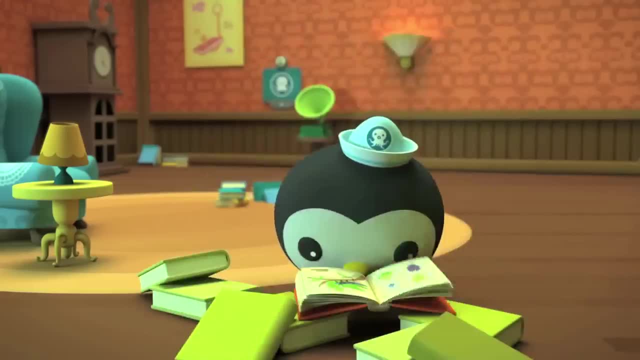 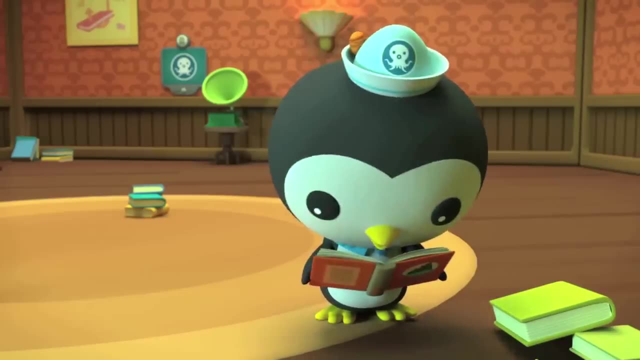 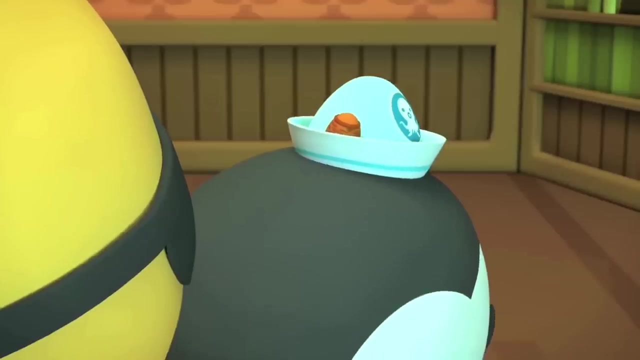 Just a few more books. matey, A tree lobster, I knew we'd find them. Listen to this, Lord Howe's Island. Stick Insects, or tree lobsters, once lived on islands off the coast of Australia. Shiver me whiskers. 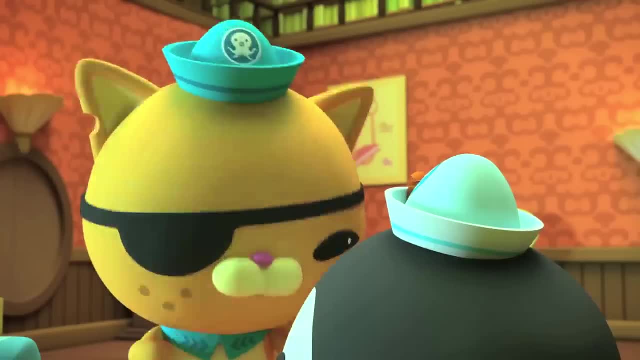 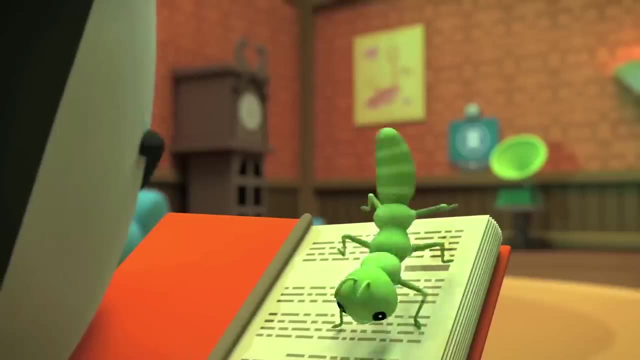 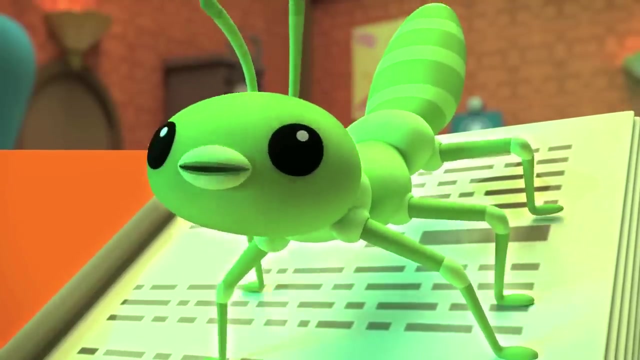 It's amazing. It's amazing, isn't it? Unfortunately, no one has seen a living tree lobster in many years. I see one right now and it's on your head: A baby tree lobster. I must have somehow brought one of the eggs back with me. 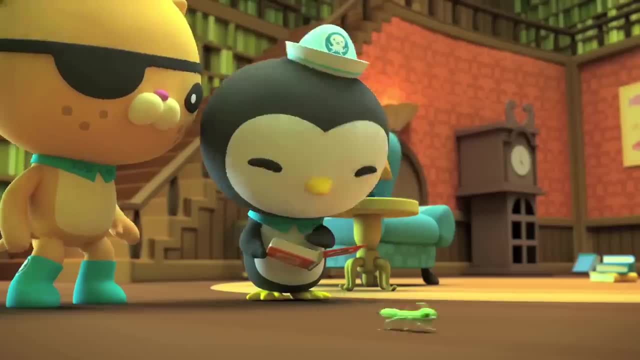 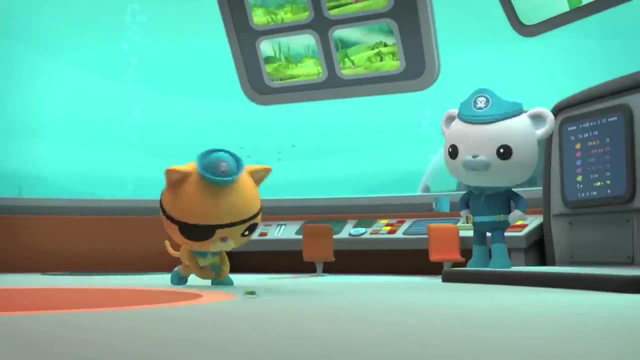 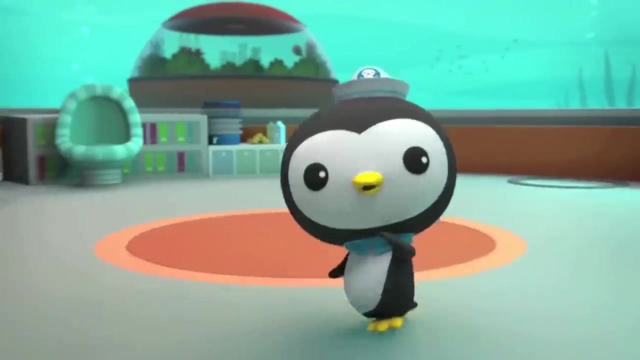 We'd better get you back home. He's getting away, Kwasi Peso. What's going on? There's a real-life tree lobster loose on the ship. We have to catch him. Captain Sound the octo-alert Octonauts to the agent. No Octonauts to the launch. 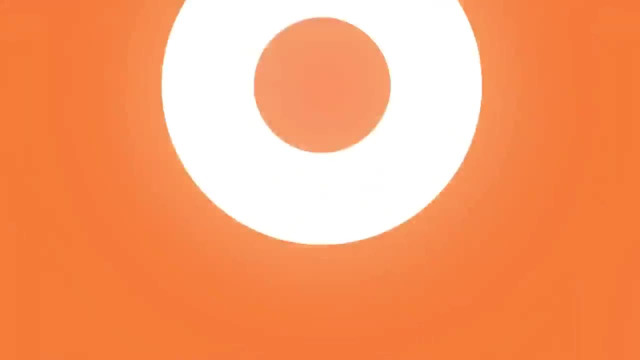 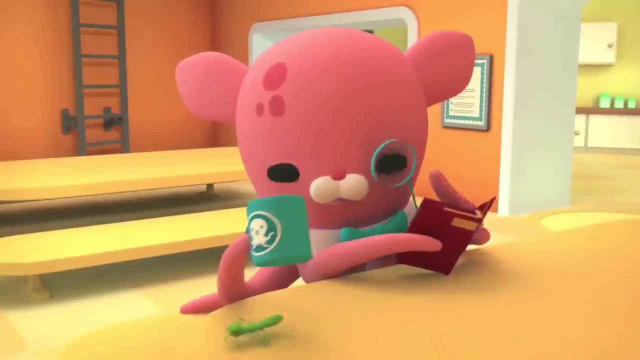 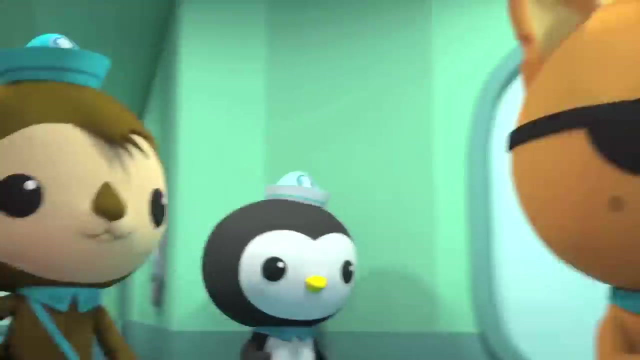 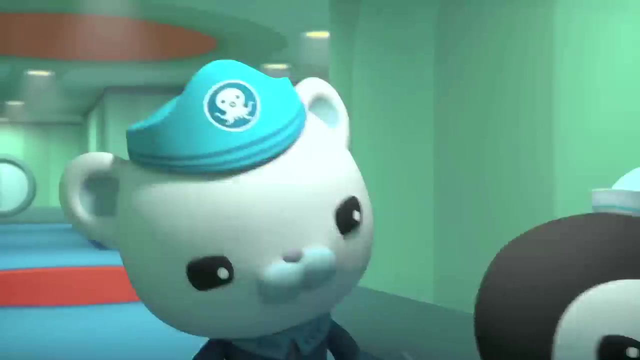 Follow that tree lobster- Incredible. I've never seen anything like it. Ha-ha. We knew that tree lobsters were real, didn't we Peso? All right, He's heading for the kitchen. Watch out vegetables, Yes. 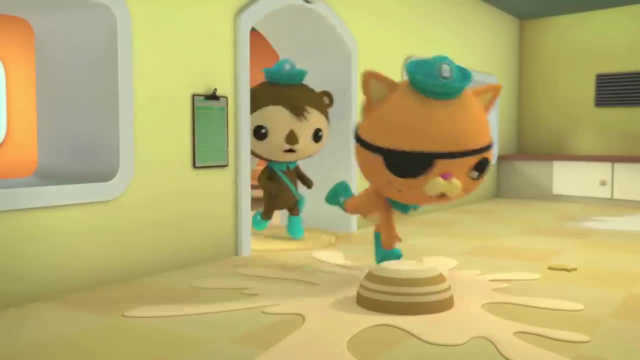 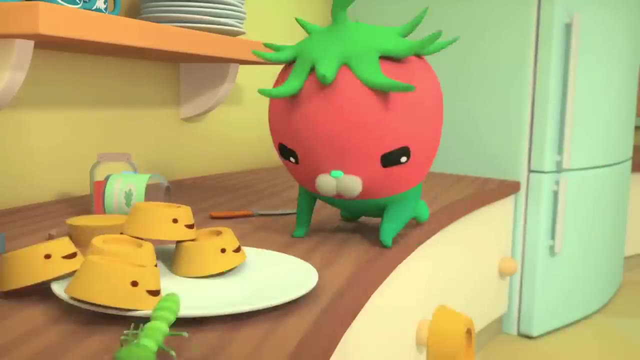 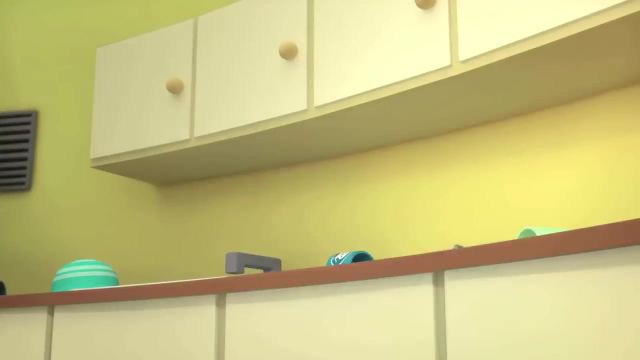 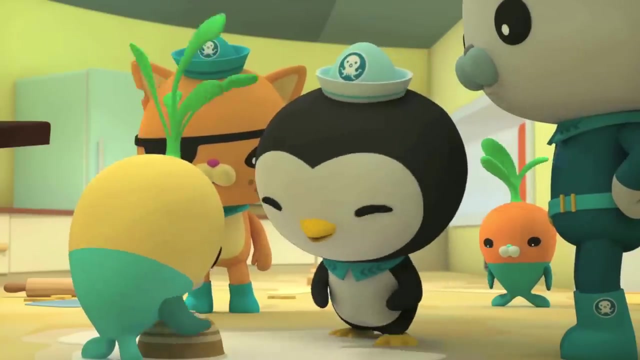 Ah, Ah, Oh, Ha-ha-ha-ha-ha. Ha Ha Ha, Ooh, got him. Ha Ha Ha. Lift it up slowly, Tunip, We don't want to startle him.